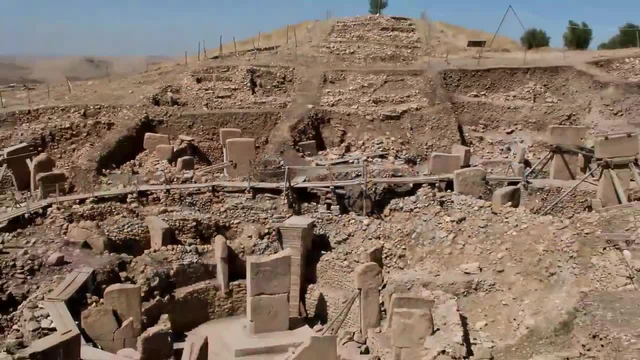 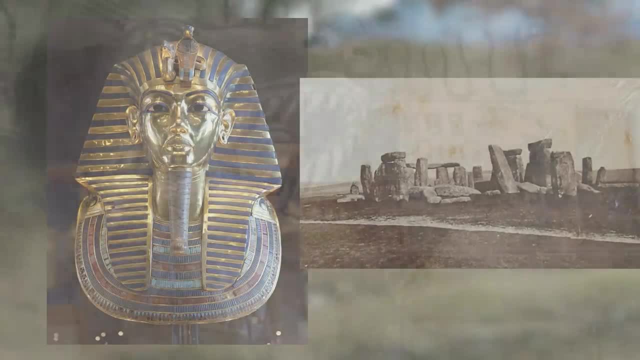 Archaeology. It's a fascinating field of science devoted to unearthing the shared past of humanity. To most people, it's mainly mummies and Stonehenge, but to archaeologists like me, it's more than that. Today I Trade the Explainer, am going to take a deep dive into some of the 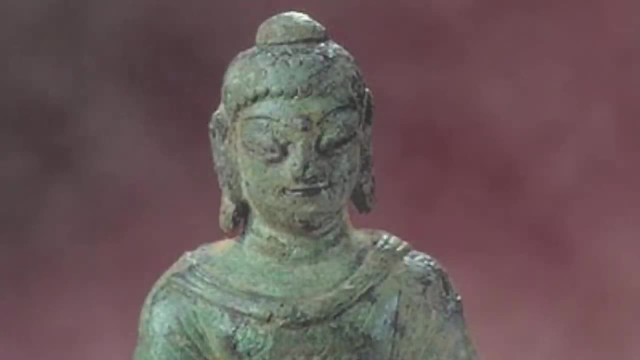 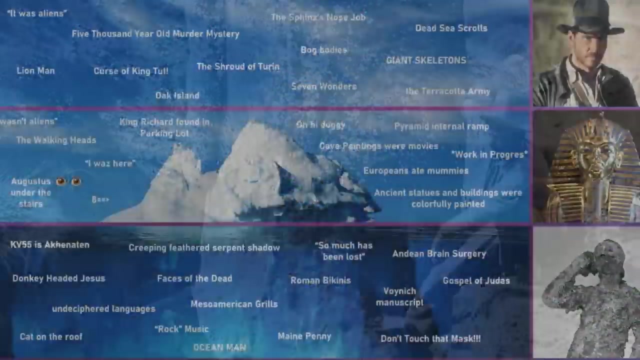 weirdest, most obscure and just fascinating finds and stories in the history of archaeology that the average person doesn't really get to hear about. And I am doing this in the iceberg meme format, where at the top are things people generally know about and as we get closer and closer to 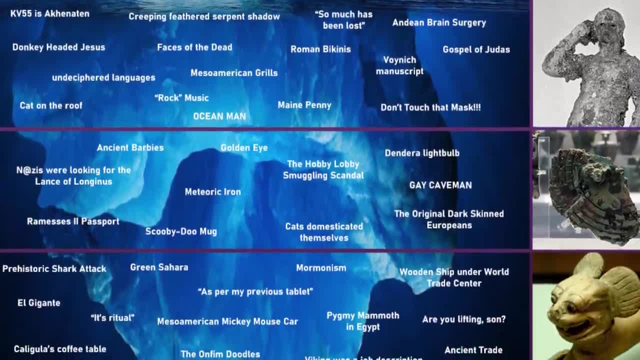 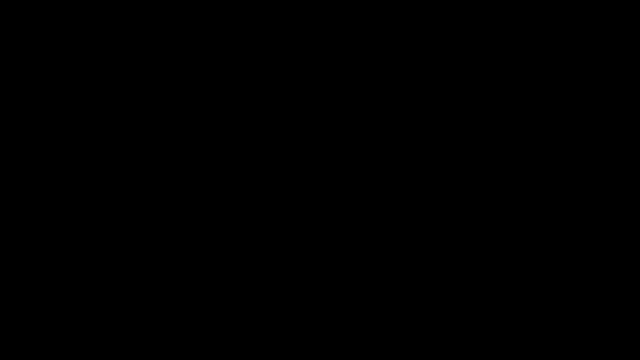 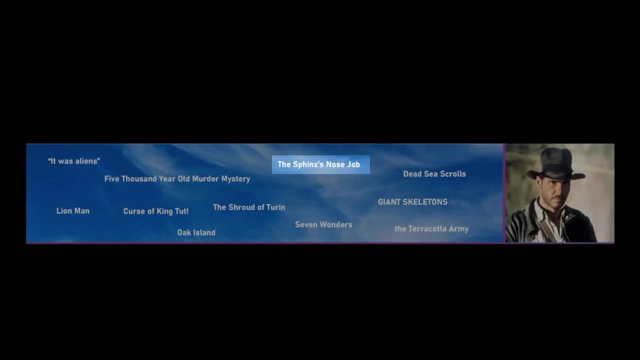 the bottom, the topics will get weirder and weirder and more niche. Okay, are you ready? This is the Archaeology Iceberg: The Sphinx's Nose Job. This refers to the apparent absence of the Great Sphinx of Giza's nose. A popular legend claims that the nose job is the nose job of the Great Sphinx of Giza. The Sphinx's nose job is the nose job of the Great Sphinx of Giza. The Sphinx's nose job is the nose job of the Great Sphinx of Giza. 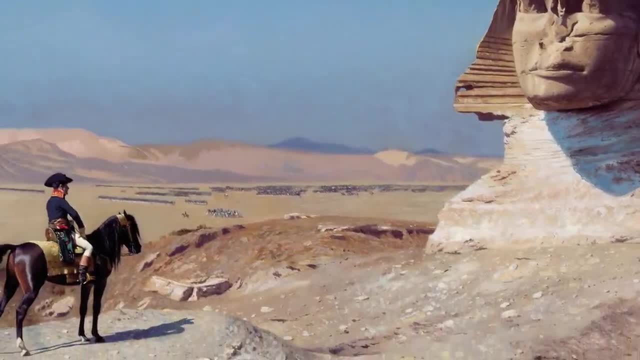 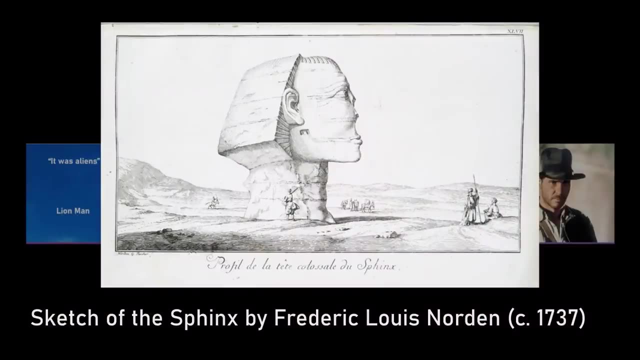 The nose was shot off with a cannonball by a couple of Napoleon Bonaparte soldiers during the 19th century. This story, however, is clearly false. as many illustrations show, the Sphinx already lacked a nose centuries before Napoleon was even born. The nose is thought to have been: 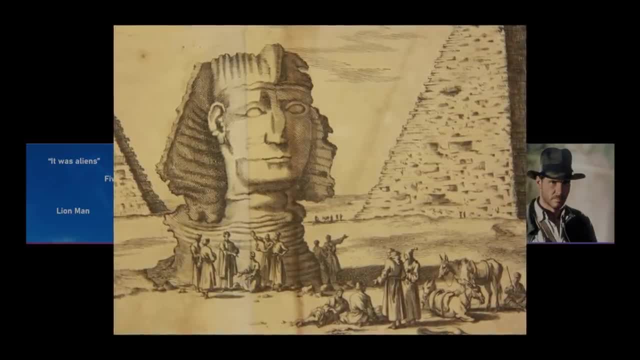 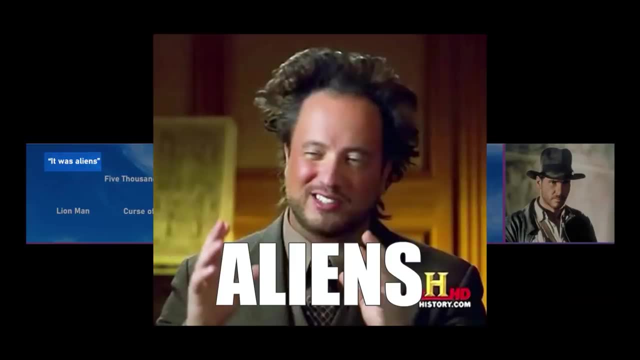 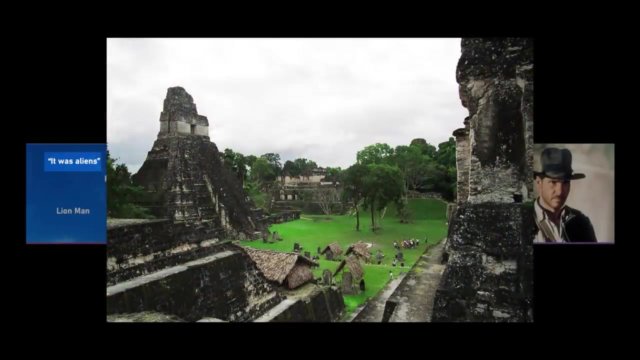 intentionally removed sometime during the 3rd to 10th centuries AD. It also once had a beard. It Was Aliens. This statement refers to the fringe ancient astronaut or ancient aliens conspiracy theory popularized by Erich von Däniken. The theory is essentially that ancient civilizations, namely non-European ones, 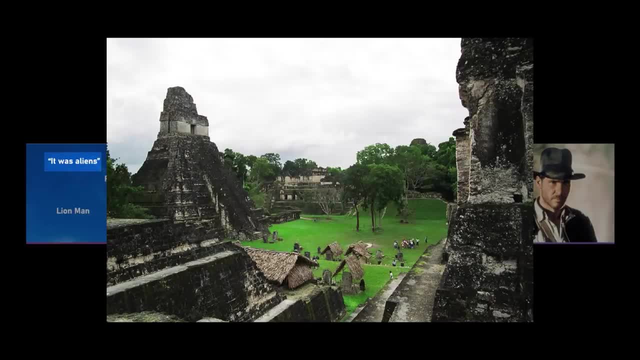 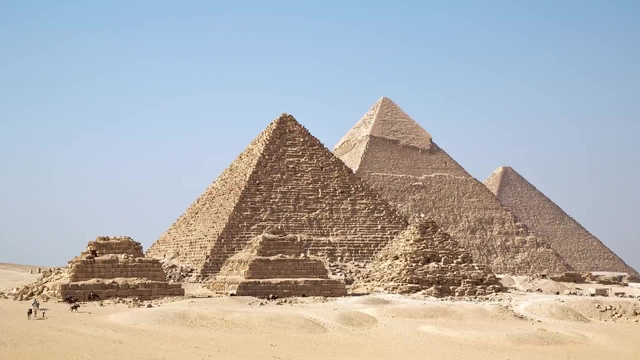 couldn't have constructed or made their technological advancements without the assistance of a more advanced civilization of aliens teaching them how to do it. Aliens apparently helped build everything, from the pyramids to Stonehenge, to the Nazca lines, because we were too stupid to do it ourselves. 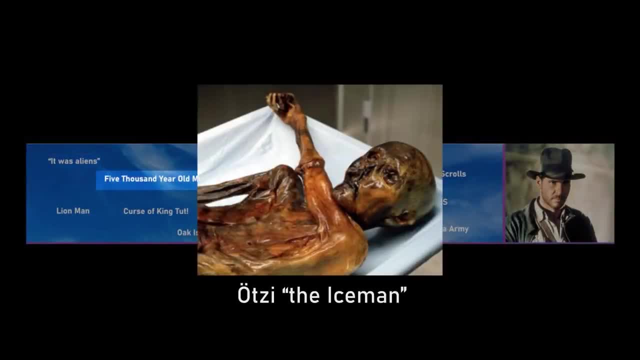 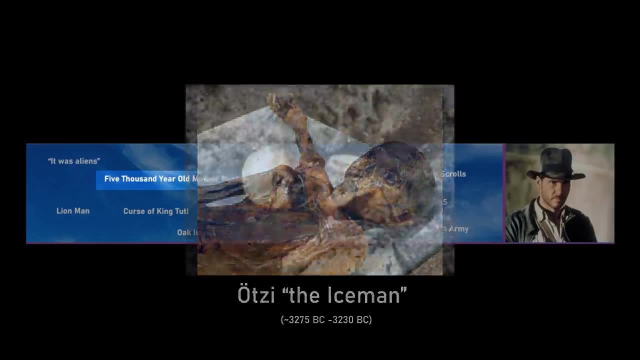 5000 Year Old Murder Mystery- A reference to Ötzi the Iceman, a naturally mummified human body dating to 3300 BC. He was discovered encased in ice on the border between Austria and Italy with his 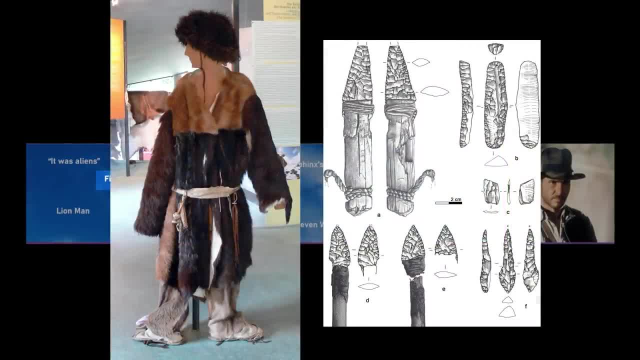 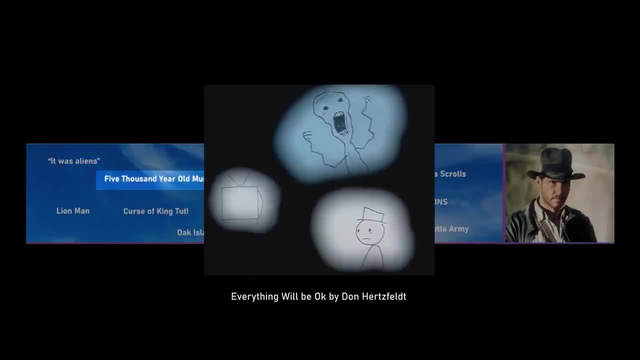 clothes, belongings, skin and organs all intact. He is perhaps one of the oldest and most well preserved human specimens to date. Scientists explored its colon and everything on live television. Examinations of his body appear to show that Ötzi was murdered by an unknown assailant. 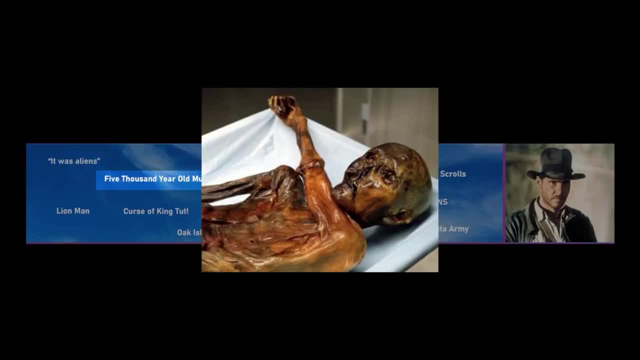 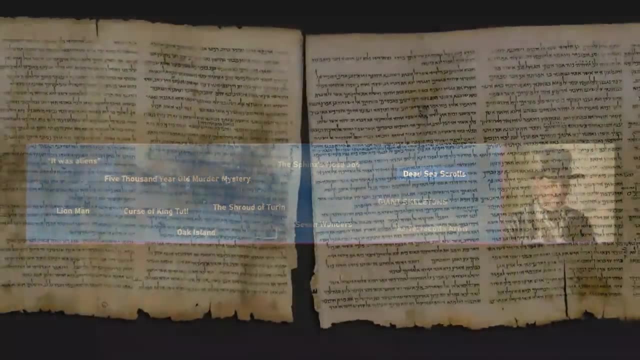 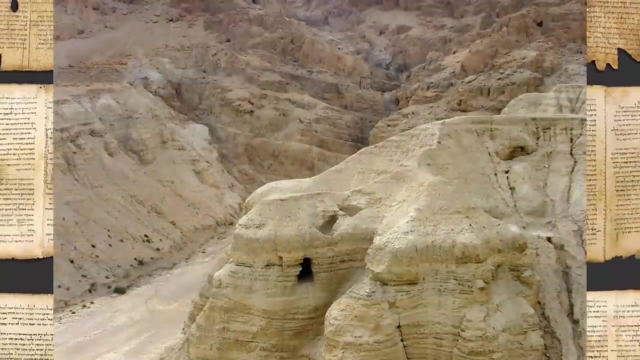 and left for dead in the snow thousands of years ago for reasons unknown. It's a real cold case. Dead Sea Scrolls: These are possibly one of the most significant archaeological finds of the past century. They are a collection of Hebrew manuscripts discovered in a system of desert caves. 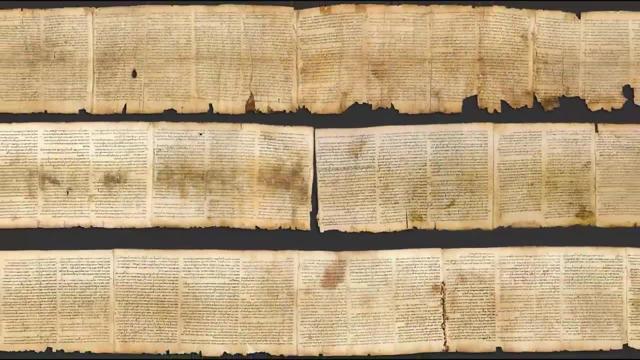 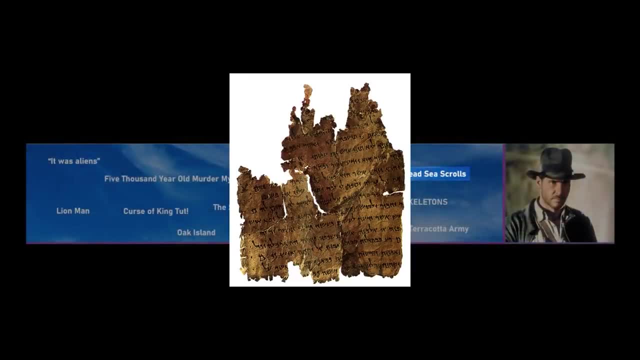 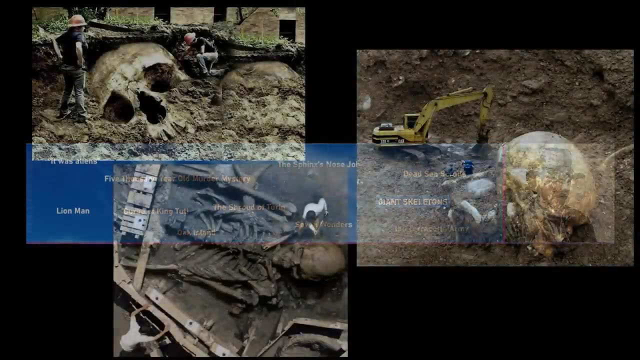 in the West Bank, originally by a goat herder. This collection of documents consists of some of the oldest surviving copies of the Hebrew Bible or Old Testament, dated to about 408 BC to 318 AD. Giant Skeletons- This is a reference to Nephilim conspiracy theories on the internet. 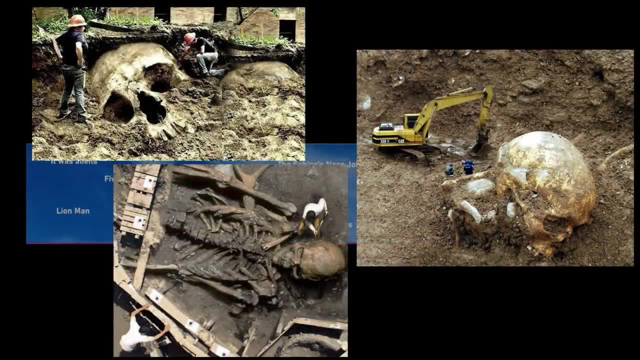 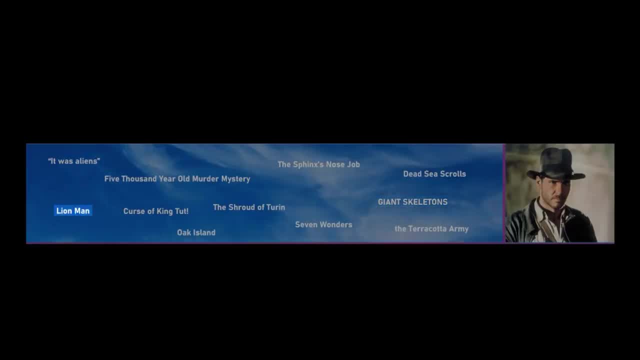 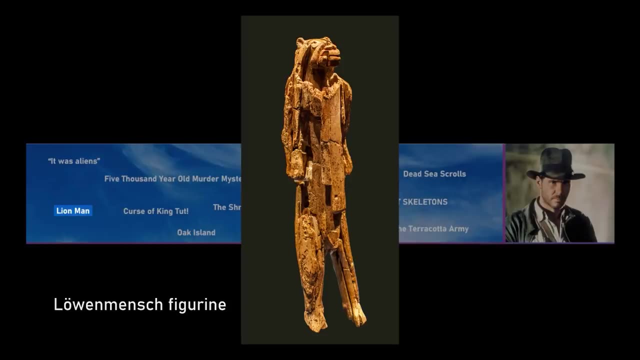 Dozens of poorly photoshopped images of giant skeletons are presented as evidence for a race of building-sized humans in our distant past- Lion Man. This is the Lawenmensch, a prehistoric figurine of a lion-headed man carved into mammoth ivory and dating to between. 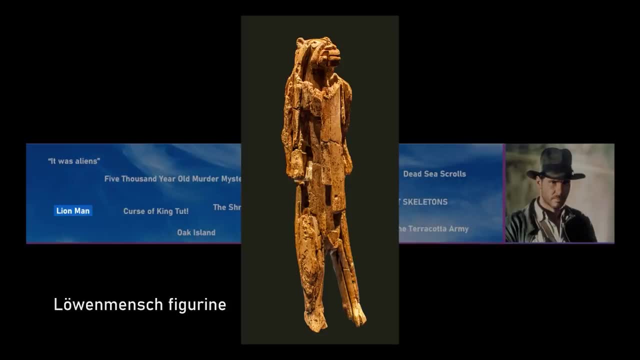 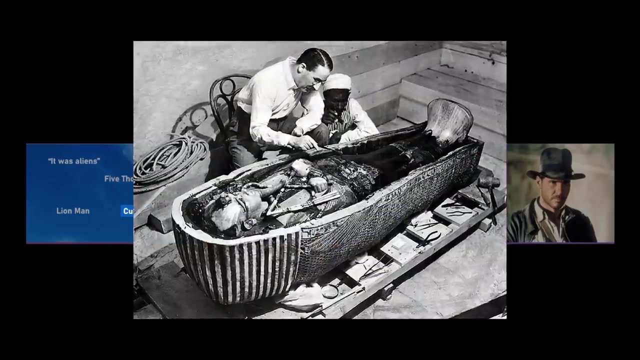 35,000 to 40,000 years old. It is one of the oldest examples of figurative art and fursonas. Some say it might be a bear-headed man instead of a lion, but who knows? Curse Of King Tut. This refers to the superstitious belief that the opening of the tomb belonging 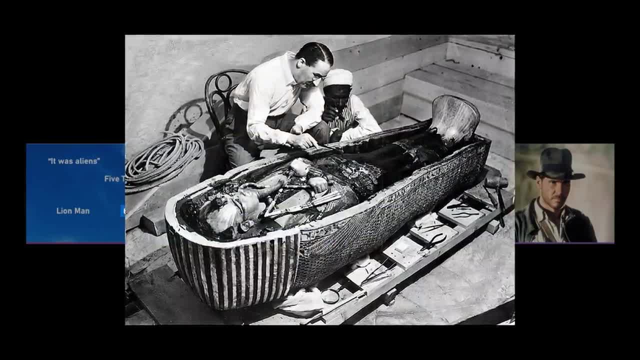 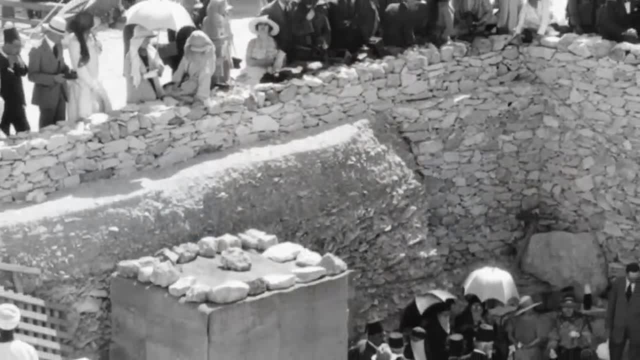 to the boy pharaoh Tutankhamun in 1923, placed a curse on the excavation team and other visitors, resulting in many untimely deaths. In truth, out of the 58 people who were present when the tomb was opened, only about 8 died prematurely within a dozen years. 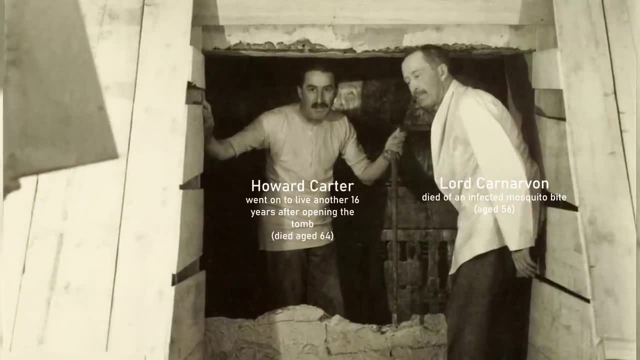 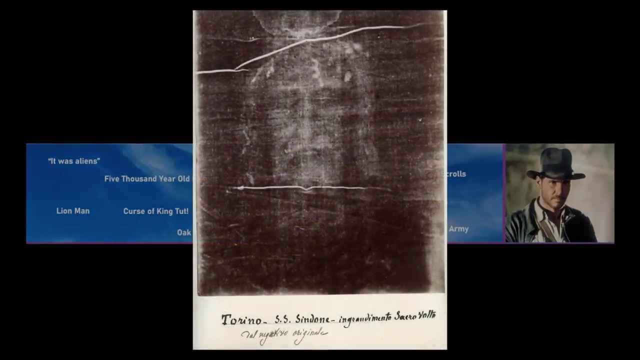 Many of those deaths were the result of outside factors such as malaria and fever, and probably not related to the excavation at all. Most people who survived the tomb went on to live otherwise healthy and long lives. The Shroud of Turin. The Shroud of Turin is a controversial linen cloth which contains the 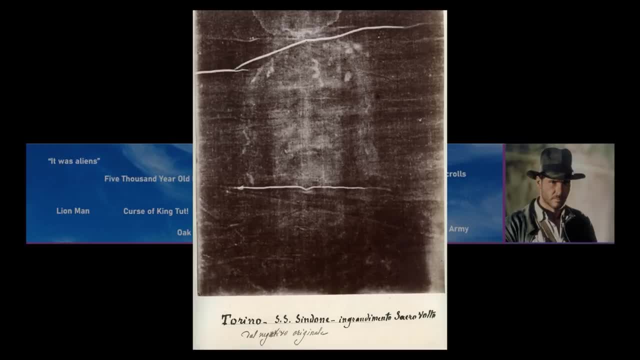 negative image of a bearded man. Many have claimed that the cloth was used to wrap Jesus Christ after his crucifixion. However, numerous scientific tests conducted on the cloth have shown it to be most likely a counterfeit product of the Middle Ages rather than an authentic relic. 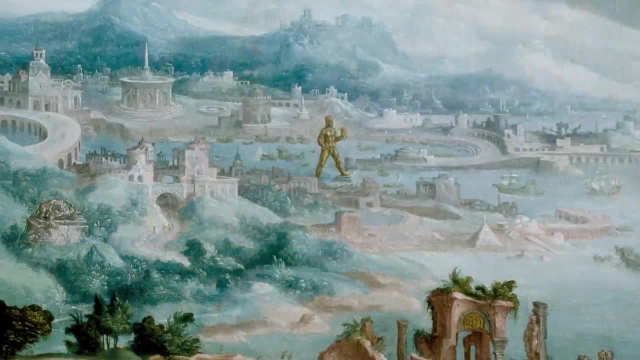 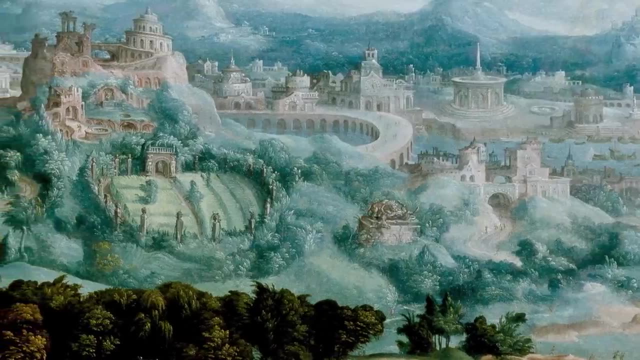 Seven Wonders. According to ancient historians, there were seven legendary man-made minds built in antiquity that Greeks and Romans marveled at for their beauty and sheer impressive scale. All of them, save one, the Great Pyramid of Giza, have been 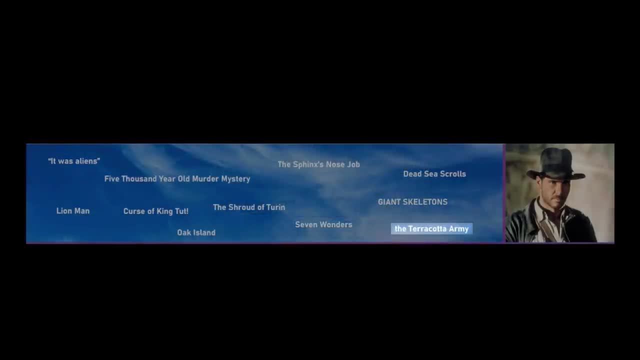 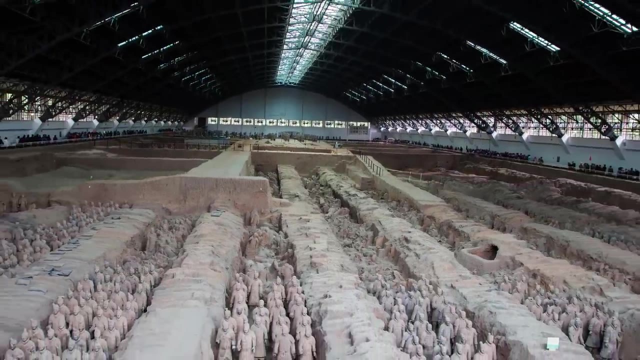 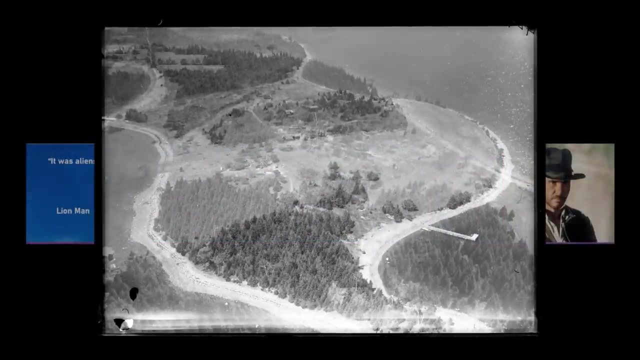 destroyed or lost to time. The Terracotta Army: This is an immense collection of terracotta sculptures depicting the vast army of Qin Shi Huang, the first emperor of China, and buried with him for the purpose of protecting him in the afterlife. Oak Island- Oak Island is an island in Nova Scotia that has been the 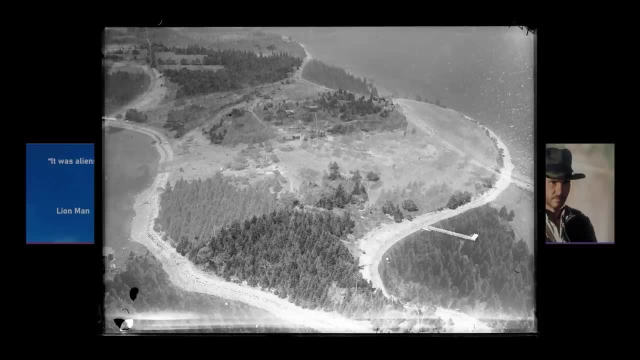 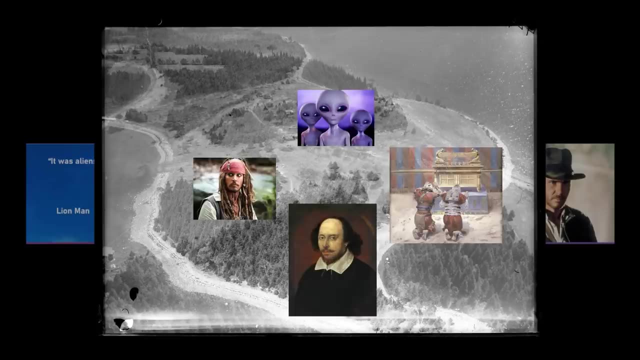 focus of pseudo-archaeologists for several hundred years. Many enthusiasts have become convinced that anything from alien technology to pirate gold, to the Ark of the Covenant, to Shakespeare's lost plays, exist beneath the island in the so-called money pit. The search has been fruitless for many decades, as no. 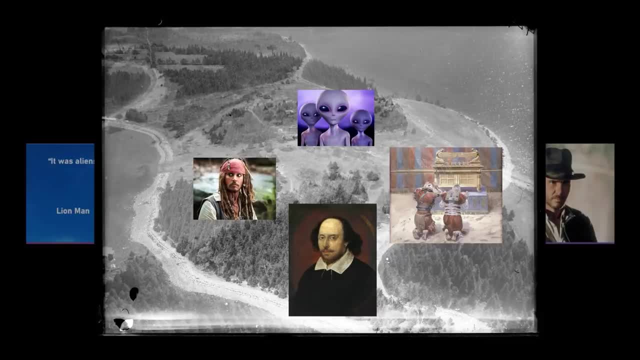 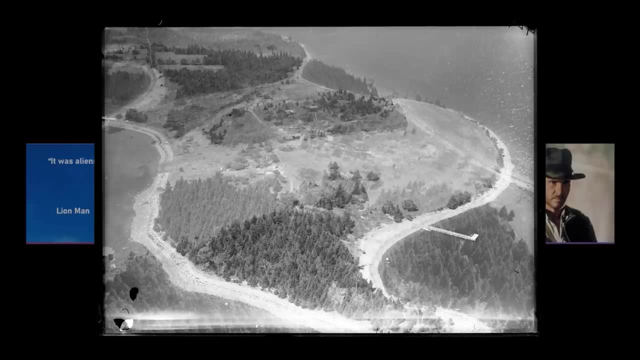 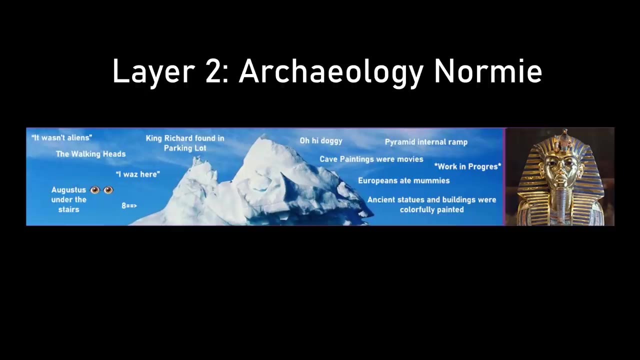 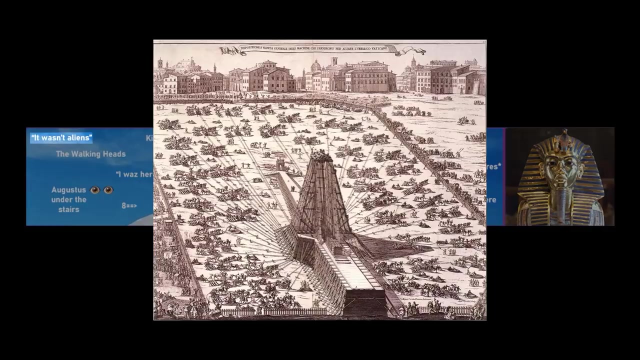 significant treasure, site or artifacts have been uncovered. despite the claims of its proponents, There's probably nothing there. Also, like King Tut's tomb, a curse is believed to exist around the site. However, this hasn't been substantiated. It wasn't aliens. If there's one thing archaeologists have discovered, it's that 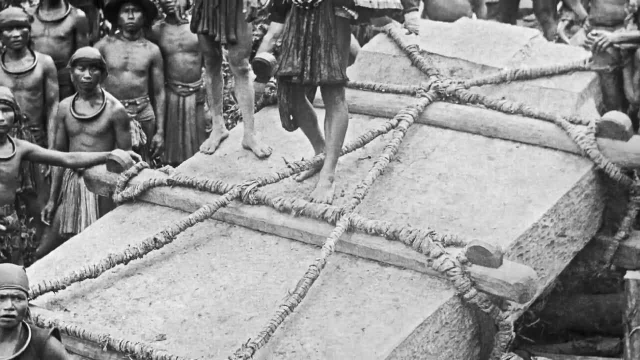 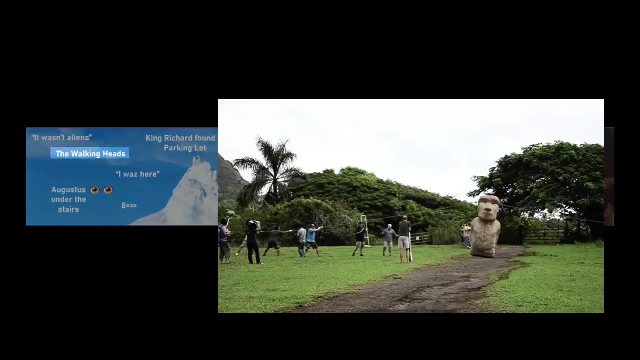 humans are crafty and smart buggers, constantly finding unique and ingenuitive ways to reach a goal. Just because it wasn't white people doesn't mean it was aliens. The Walking Heads In 2012,: a team of archaeologists. 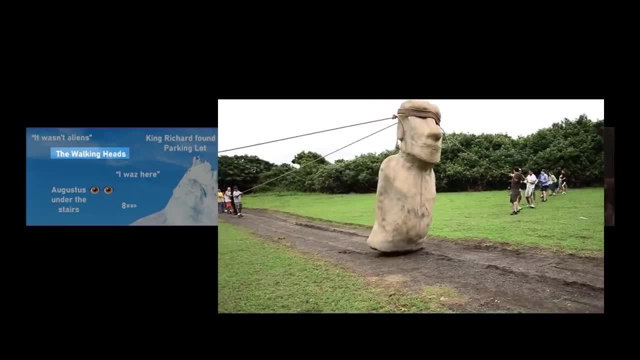 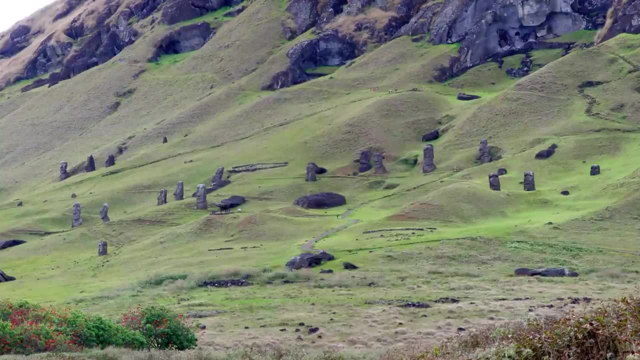 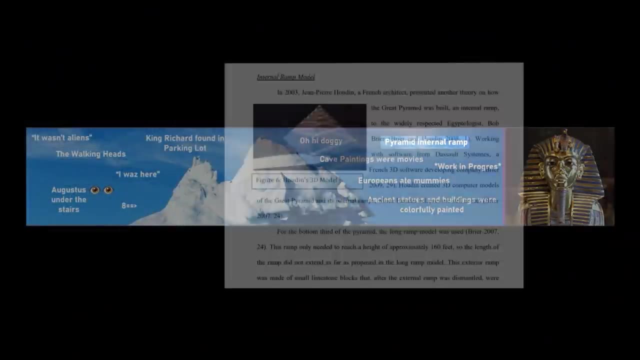 successfully transported a five-ton Moai head replica using only rope and manpower as an experiment to replicate the methods by which the people of Easter Island in the past might have transported the heads themselves. No aliens were required. Internal ramp theory: This refers to one of the several 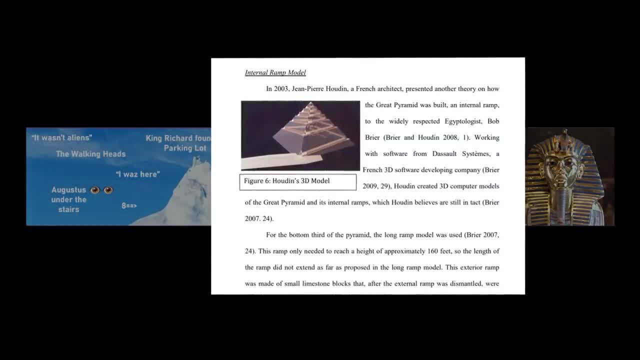 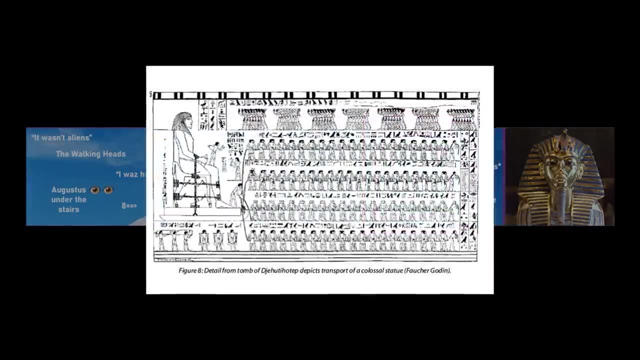 competing methods by which the Great Pyramid of Giza was constructed. The internal ramp theory posits that an internal spiral ramp exists within the pyramid itself and aided in the dragging of building materials during construction. Archaeological evidence supporting this view exists, although it has not yet been found. 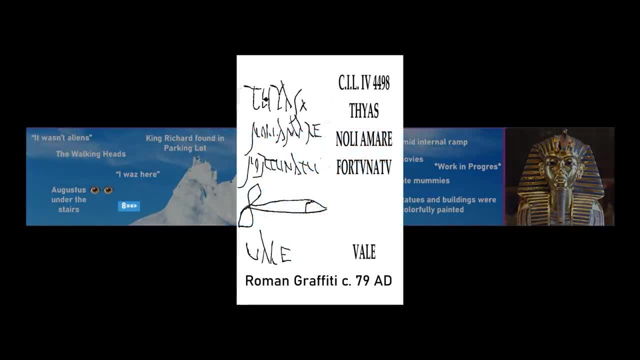 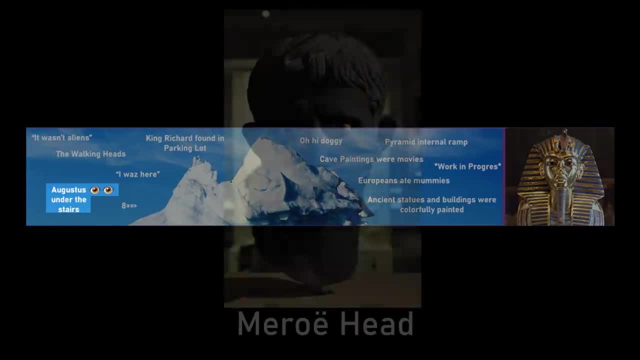 been fully accepted. yet There is seemingly a universality of humans' tendency to draw these little rocket ships on everything. Augustus Under the Stairs. This is the Meroe Augustus, a decapitated bronze head originally belonging to a statue of the famous Roman Emperor. 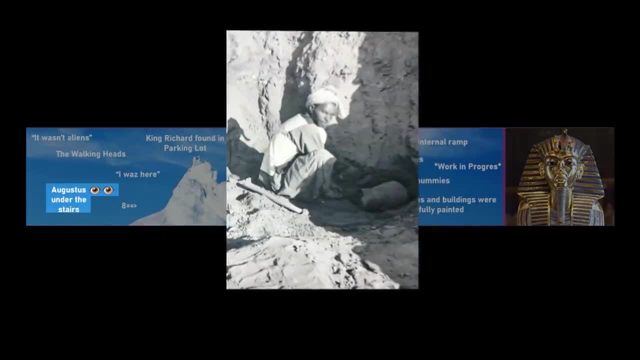 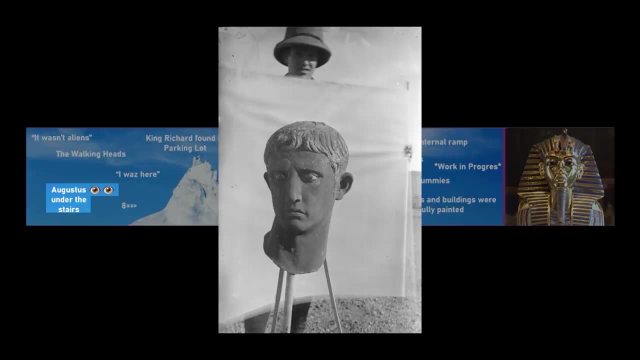 It was discovered beneath the staircase of an ancient Kushite temple in what is now Sudan. In 24 BC, the head was hacked off from its original body in Roman Egypt by invading Kushite soldiers, who took it across the border as a prize of war Back in Kush, 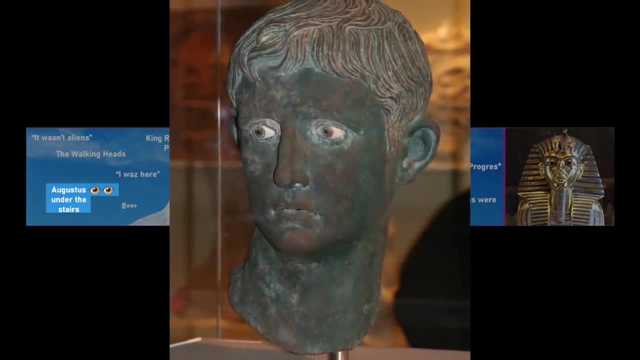 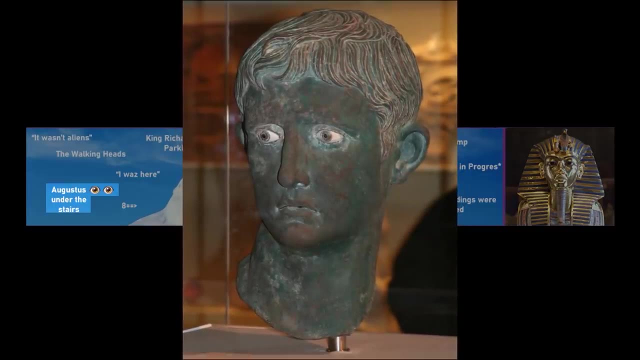 as a gesture of victory, the head was buried beneath a temple staircase, so worshipers would symbolically step on the defeated Emperor's face. This insult, however, had the unintentional consequence of preserving it over thousands of years, better than pretty much any other. 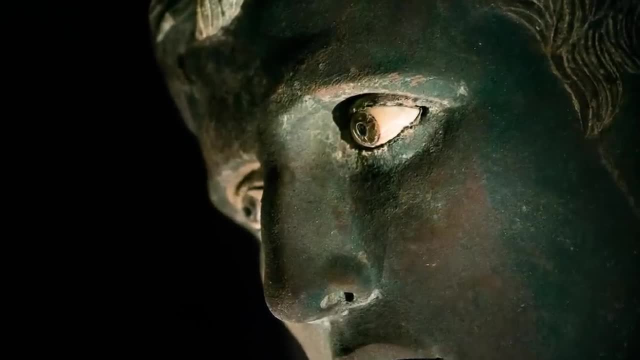 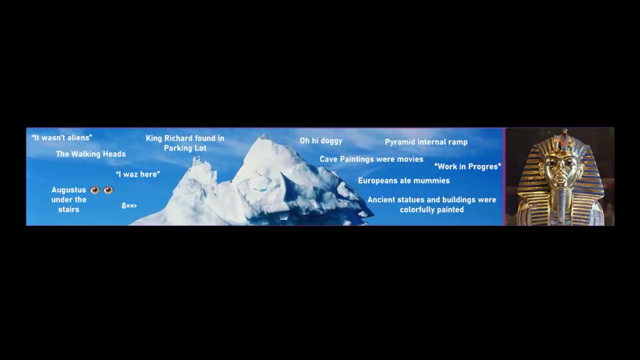 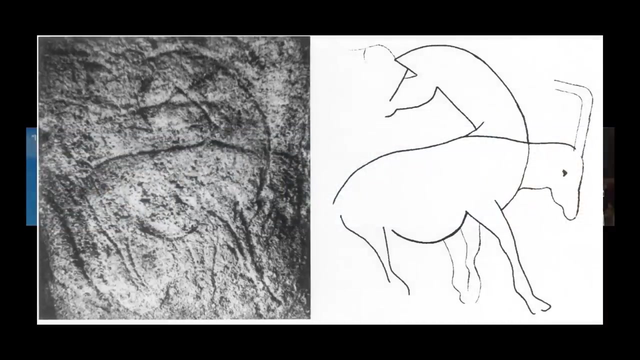 Roman bronze. Notably the head, retains its decorative inlaid eyes that are often missing in other specimens. Also, the eyes look like prime meme material Cave Pages. This is an interesting theory concerning the extra heads and extra limbs that are commonly depicted. 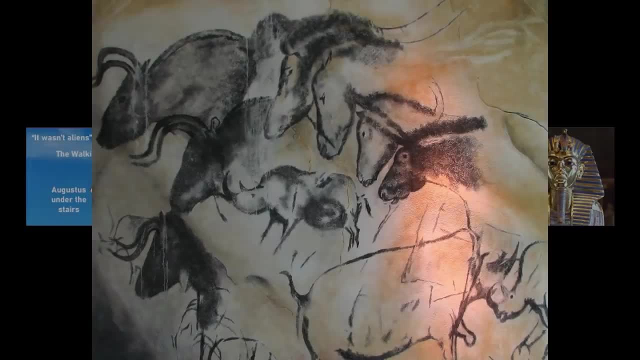 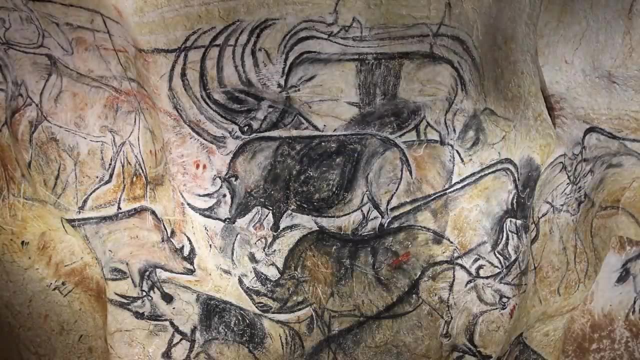 in prehistoric cave paintings of animals. The theory speculates that these duplicated body parts were drawn intentionally to create the illusion of movement. The light of torches would twist the shadows along the cave walls and make the images appear to come alive through a primitive form of animation by early humans. 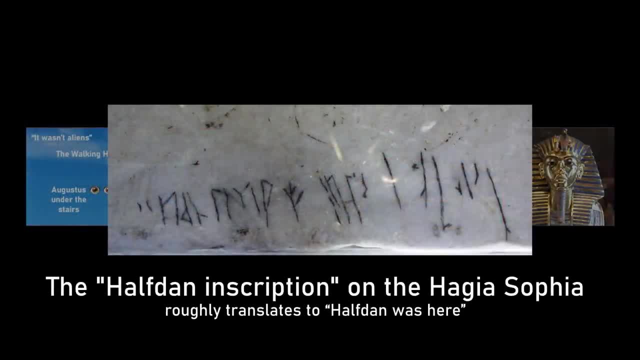 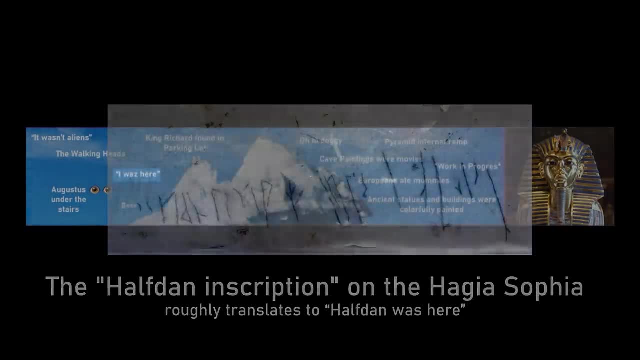 I Was Here. Throughout history, humans have always had the tendency to leave dumb, goofy inscriptions simply stating they were here. There's literally thousands of examples of these Work in Progress- The best way for archaeologists to learn about how people in the past did things. 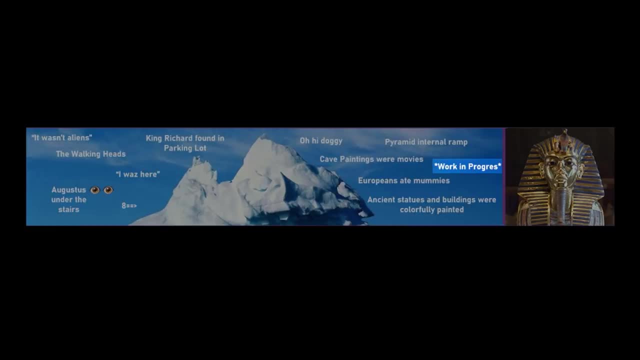 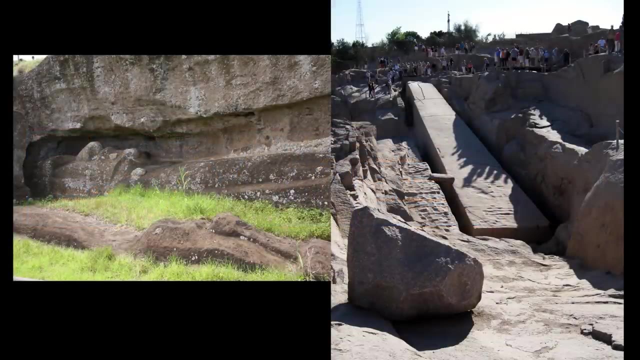 is to see what they just gave up on and left incomplete or abandoned. For example, there are dozens of unfinished moai and Egyptian obelisks chiseled out of the rock but never fully completed. These are often due to accidental damage during construction. 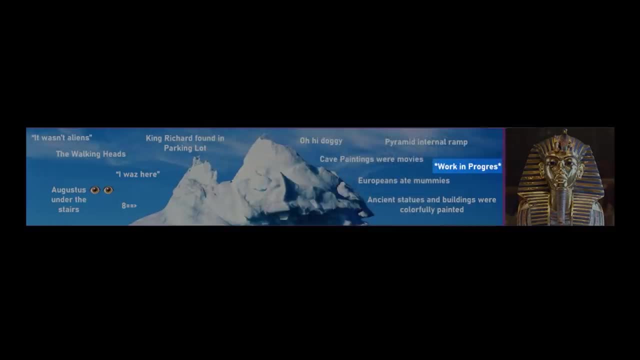 or a simple lack of enthusiasm to finish them. Some of these things are still on display, but they're still waiting to be finished after thousands of years. Man, I thought my procrastination was bad. Europeans ate mummies From the Middle Ages up until relatively recently. 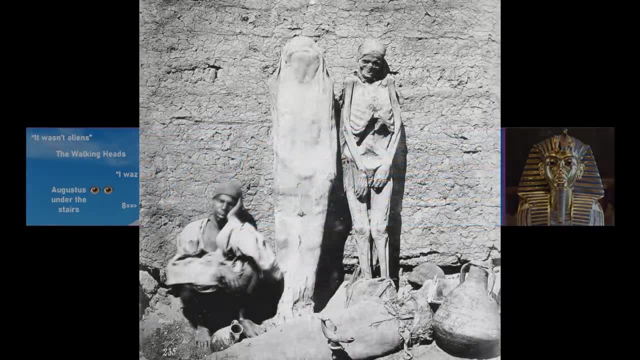 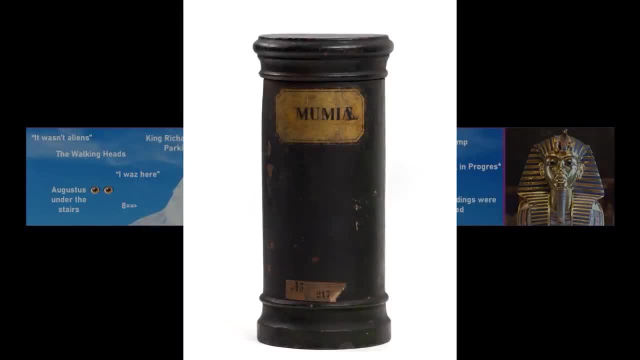 wealthy Europeans would consume the flesh of Egyptian mummies by grinding them into a powder called mummia. It was believed that this powder had great medicinal properties and could treat gout, epilepsy and cataracts. King Richard found in a parking lot. Remember that one-time archaeologist. 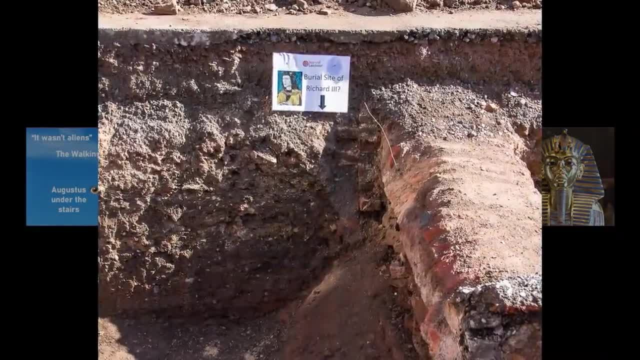 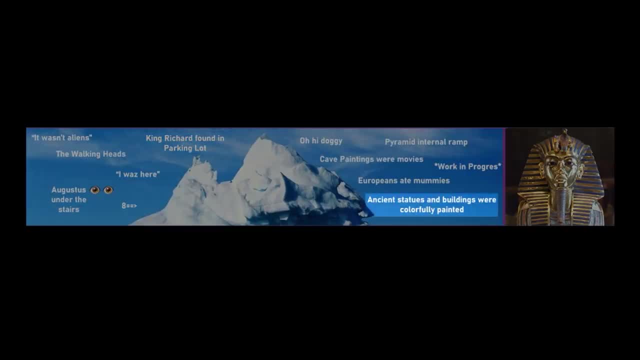 straight up found the skeleton of King Richard III, the last king of the Plantagenet dynasty, beneath a car parking lot. Good times, Ancient statues and buildings were colorfully painted, Although many of the ancient statues and buildings that survive to us today appear to be rather 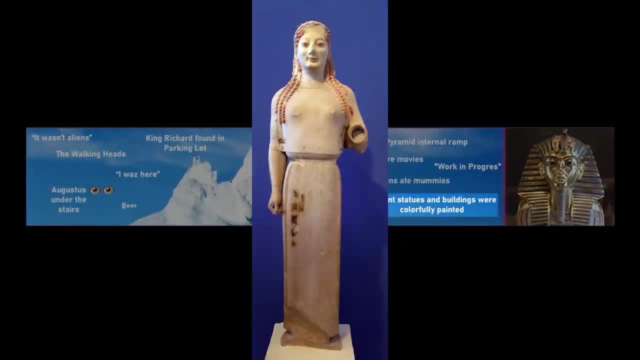 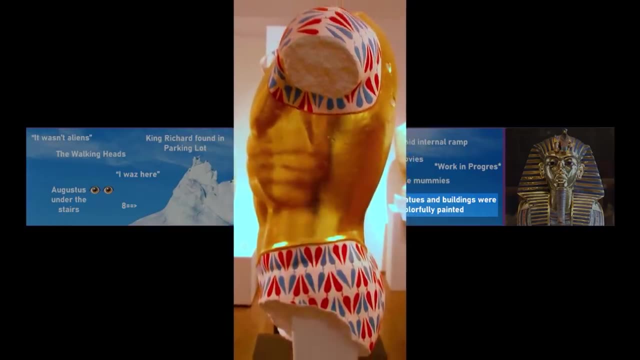 drab stone or smooth white marble in the past, they would have looked much different. Closer analysis of these monuments have shown that many would have been beautifully painted in their heyday, with faint traces of their pigments still detectable. The ancient world was in truth. 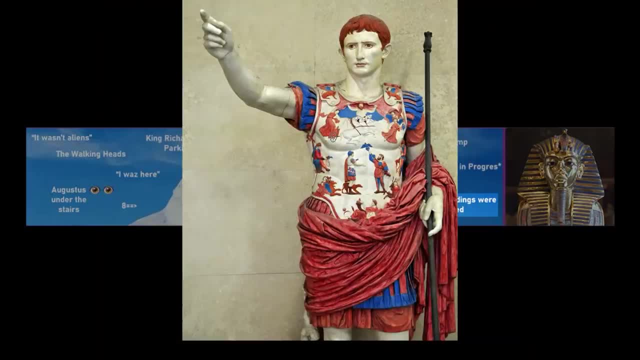 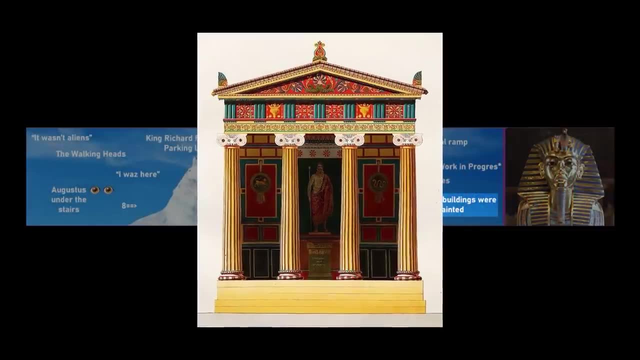 very bright and vibrant. From this statue of Augustus to the entire Parthenon, to Aztec temples, to the Sphinx's face, all of it would have been filled with color, But, due to time, many of these pigments have long since faded. Hi doggie. 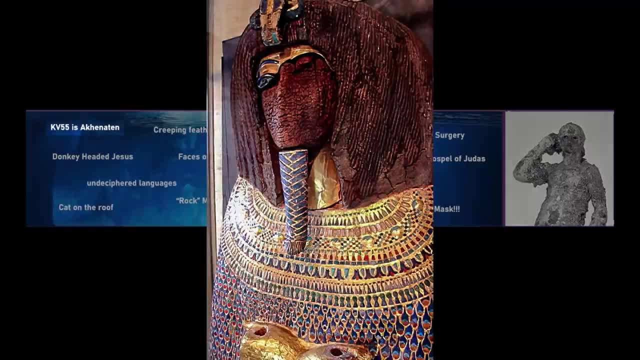 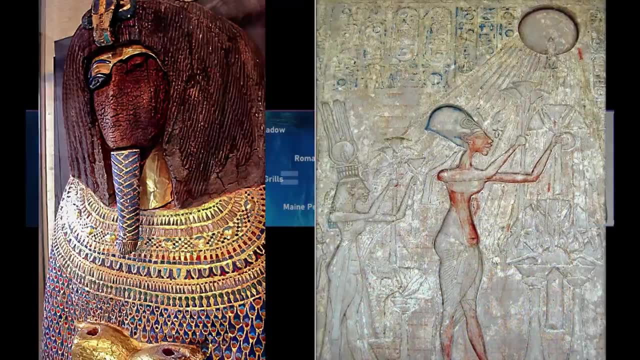 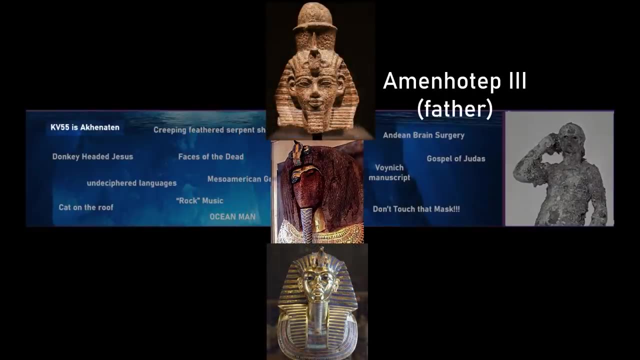 KV55 is Akhenaten. It refers to the interpretation that the mummy in Valley of the King's Tomb, KV55 is the infamous monotheistic pharaoh Akhenaten. DNA evidence appears to support this long-suspected identity, as the individual in this tomb was both the son of Amenhotep III as well as the father. 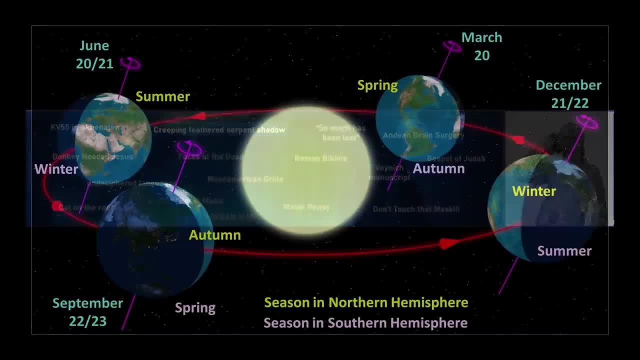 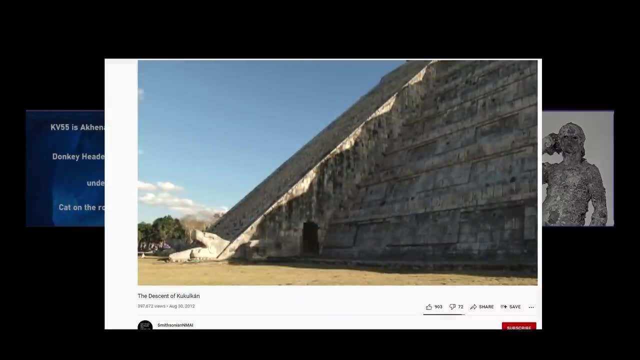 of Tutankhamun Creeping feathered serpent shadow During the spring and autumn equinoxes at the Mayan temple of Kukulkan in Chichen Itza. the sun hits the pyramid in just the right way that it causes a series of triangular shadows to creep down the front stairway. This effect only lasts a few. 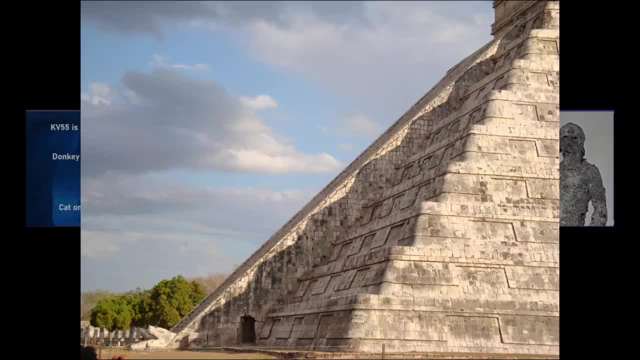 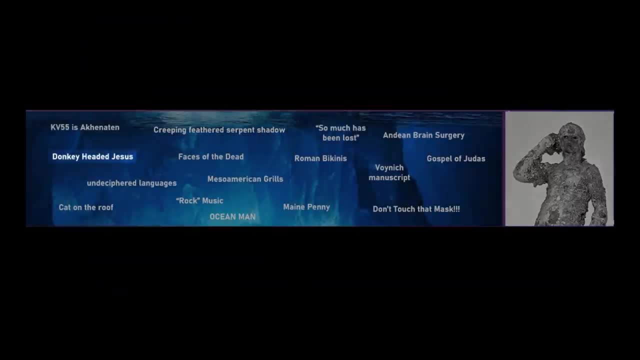 minutes out of the entire year, But through this clever arrangement of architecture, the dark body of the feathered serpent god appears to slither down to its fearsome carved head. This is the Alexis sistentios graffito, a piece of graffiti in Rome that might be. 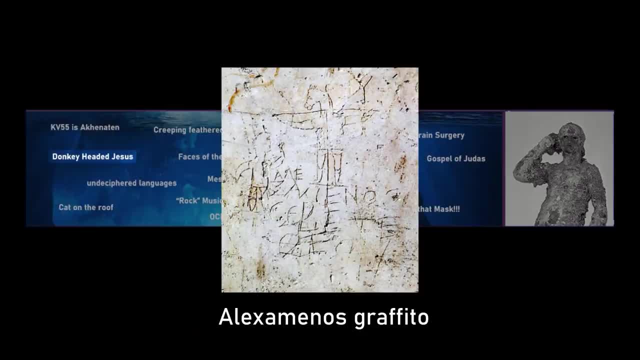 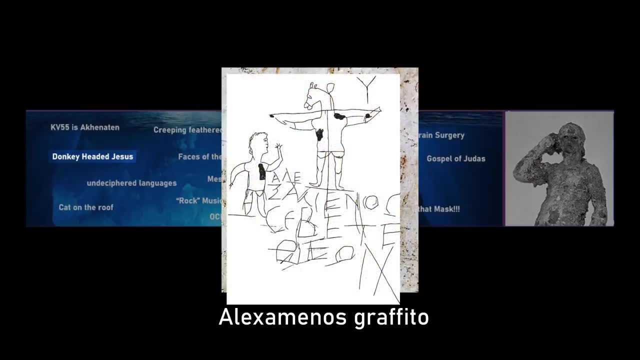 the earliest depiction of Jesus, Dated to around 200 AD. this graffiti shows a young man worshiping a crucified figure with the head of a donkey. The inscription accompanies the image stating in Greek that Alexis worships his god. It. 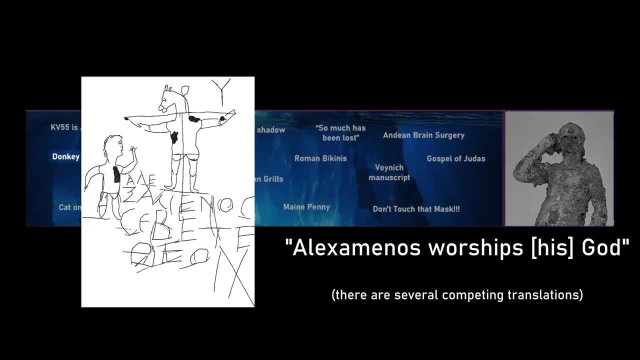 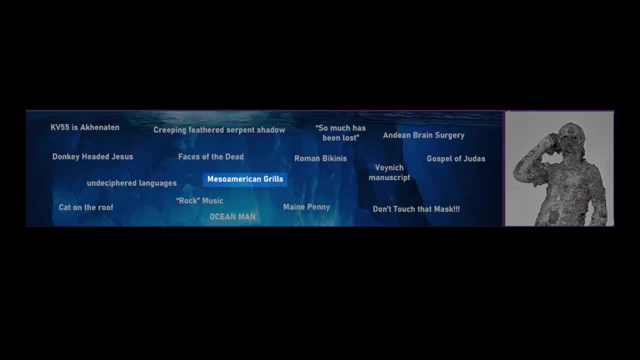 is thoughts that the drawing was created to mock someone who's still in need of a father. It's also thought that Perl early Christian named Leximenos, the donkey-headed figure being an insulting caricature of Jesus of Nazareth. Mesoamerican grills: Among several pre-contact cultures in Mesoamerica, the teeth. 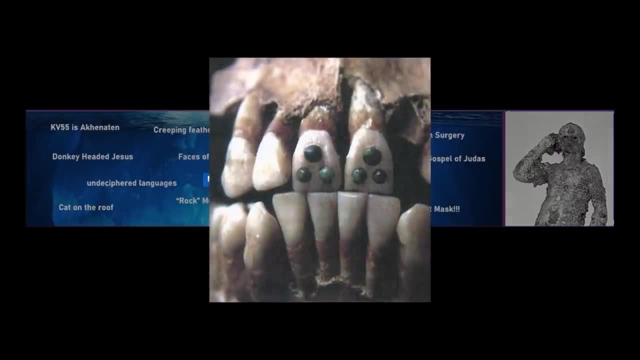 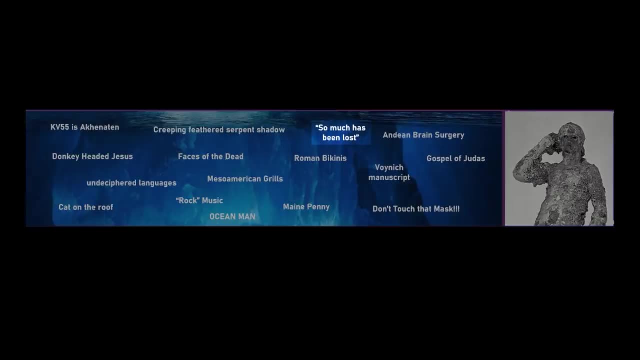 of elites were drilled into and filled with inlays of precious stones and jewels. These ancient grills were a type of status symbol as well as a huge health hazard. So much has been lost. Everything that has survived is only an incredibly small fraction of what actually existed in the 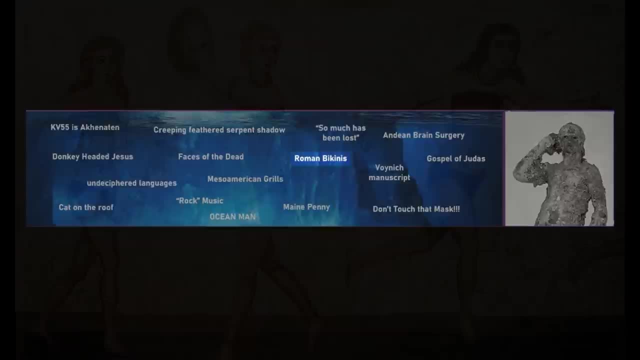 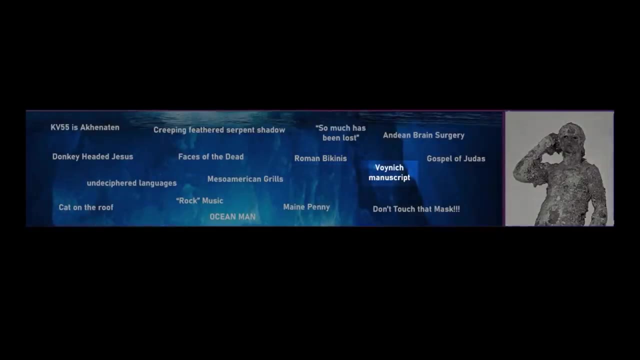 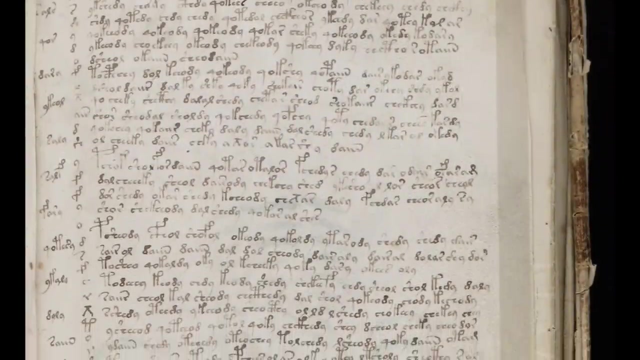 past Roman bikinis. There are several well-preserved Roman floor mosaics that depict a bunch of women wearing bikini-like athletic outfits. Voynich manuscript. The Voynich manuscript is a rather mysterious document written in an unknown writing system. It consists of nearly 240 pages. 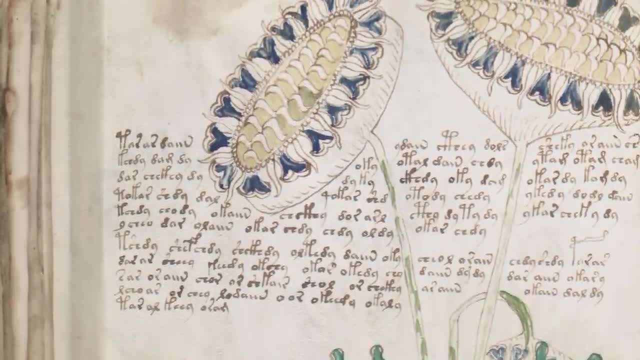 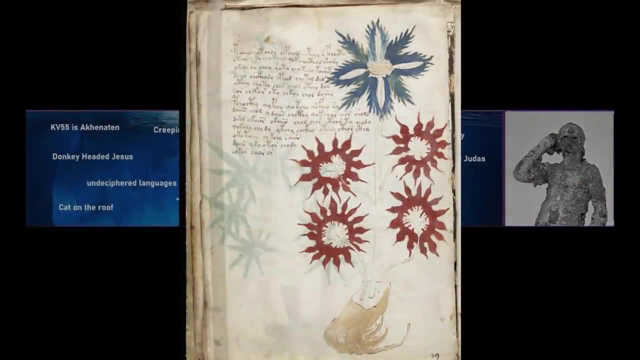 and is filled with illustrations of fictitious plants, mythical creatures and people. It has been carbon dated to the early 15th century, although its exact origin is a little muddy. It is unclear who wrote the manuscript and why. It seems probable that it was written in some. 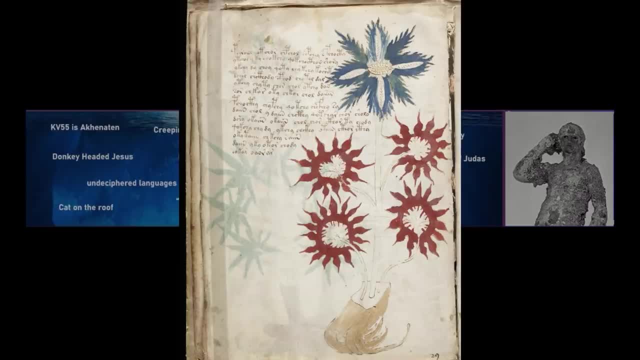 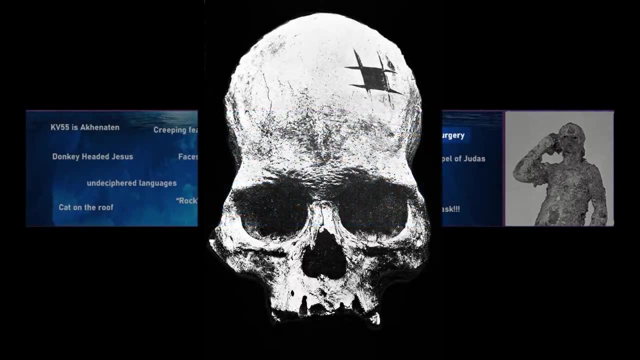 kind of cipher or code that only the author understood. Andean brain surgery. Several civilizations in the Andes Mountains conducted skull and brain surgeries and were actually pretty good at it, as evidenced by the high survival rate of patients, estimated to be around 90%. 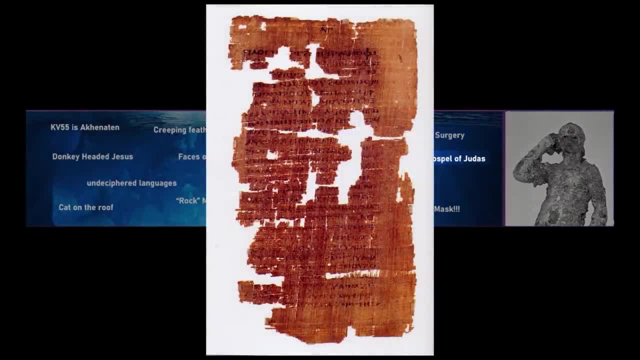 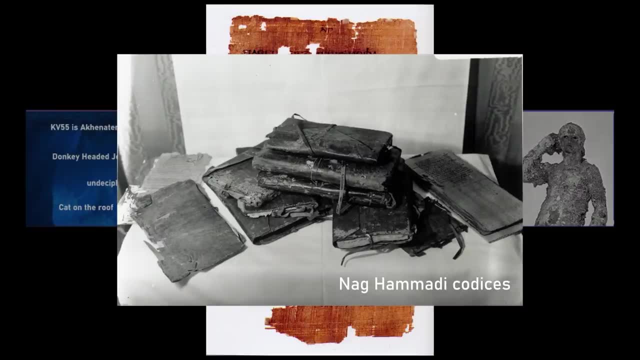 Gospel of Judas. This refers to one of the lost gospels found in the Nag Hammadi library, a collection of religious texts belonging to an early but now extinct sect of Christianity. The only fragmentary copy of the Gospel of Judas that survives us is one of the most intriguing of these documents. 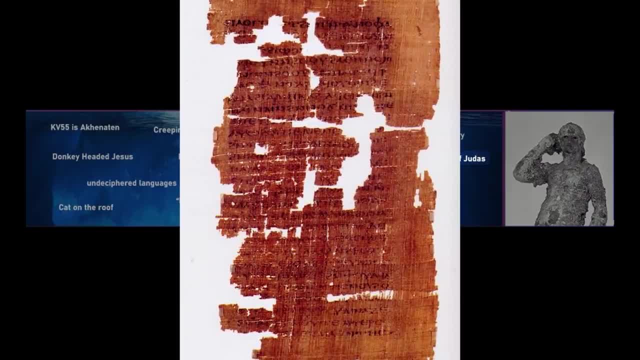 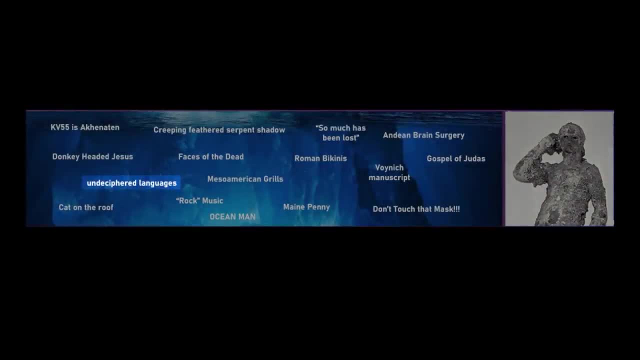 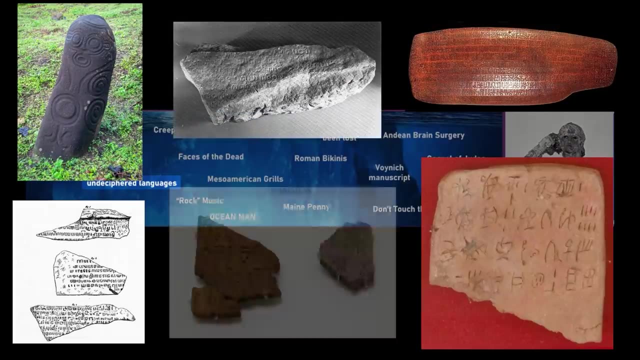 as it narrates an alternate narrative of Jesus' crucifixion and frames Judas not as a traitor but a loyal servant to the end. Undeciphered languages. All around the world there are dozens, if not hundreds, of inscriptions on everything from clay tablets to old boulders, Written in 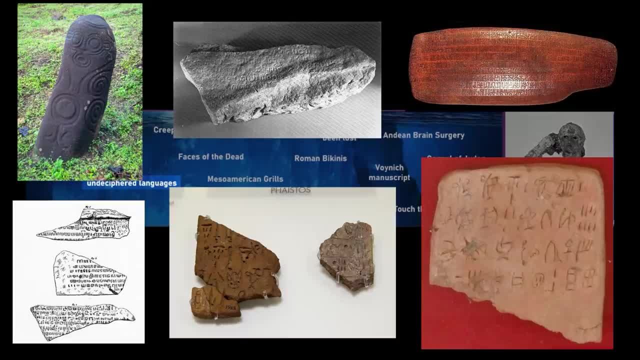 the same language. these inscriptions are as of yet undecipherable to modern experts. Although we would very much like to, we currently have no way to read what these inscriptions say because the languages they are written in have been lost to time. From Rongo Rongo on Easter. 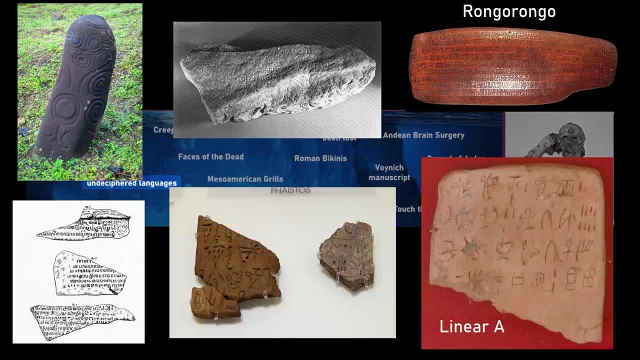 Island, to Linear A in Minoan, Crete, to the Somali scripts, to the Singapore Stone, to the writing on the back of the starving Saqqara statue. All of these are completely unreadable scripts and they still keep their secrets, At least for the moment, that is. 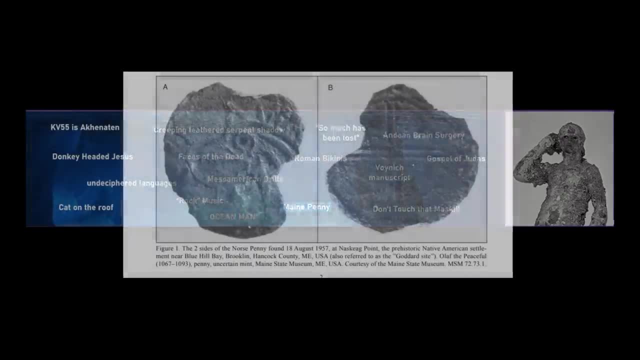 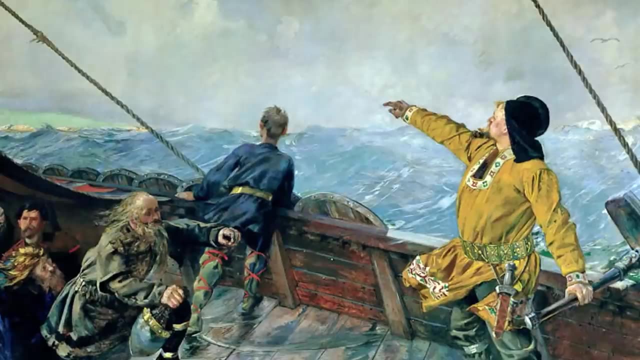 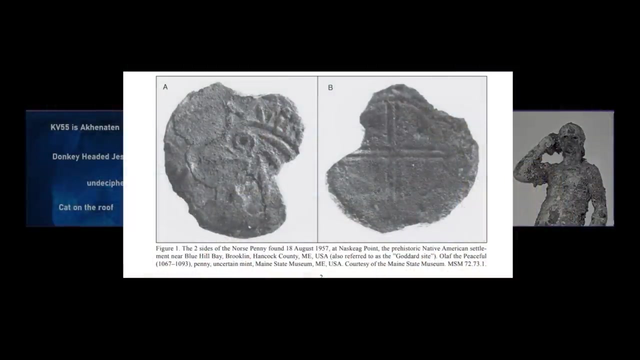 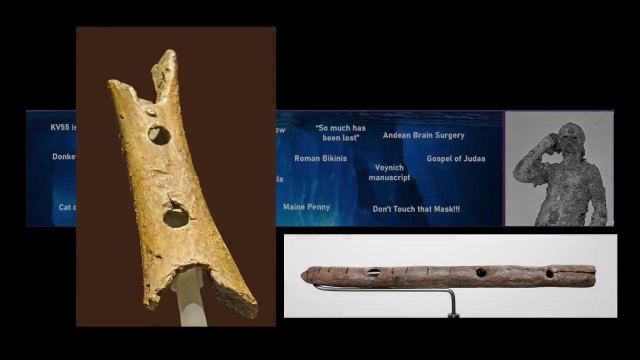 Maine. Penny Rock Music. Several fragments of Paleolithic flutes have been discovered in caves and dated to tens of thousands of years old. These ivory and animal bone flutes flutes were made by some of our earliest ancestors during the Ice Age. Archaeologists have reconstructed. 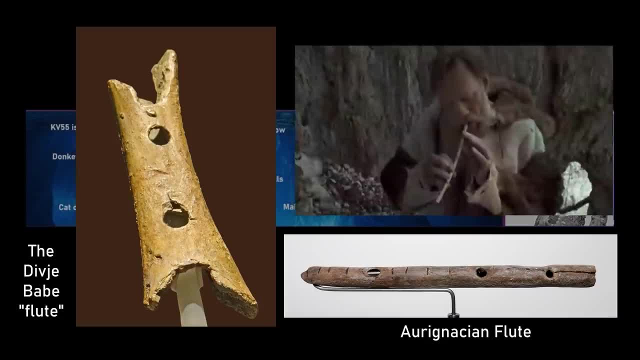 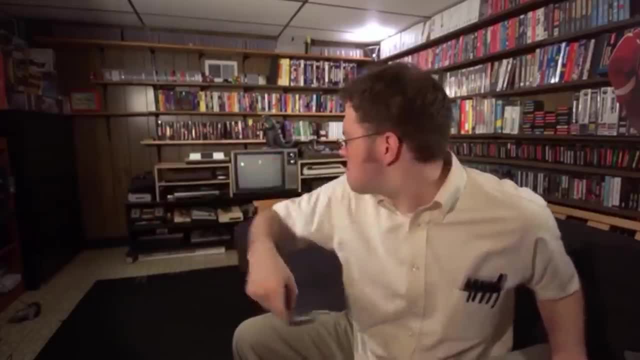 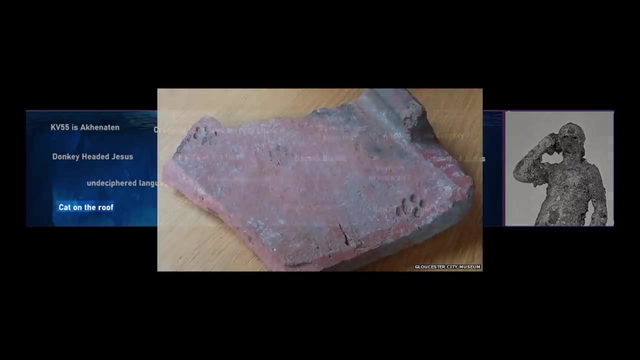 them to determine what Stone Age music would have sounded like. and boy is it eerie to imagine hearing their sad notes echoing throughout a forest in the dark of winter. Want to listen to some tunes? Cat on the Roof. As this Roman roof tile shows, even after 2000 years, cats have never changed. 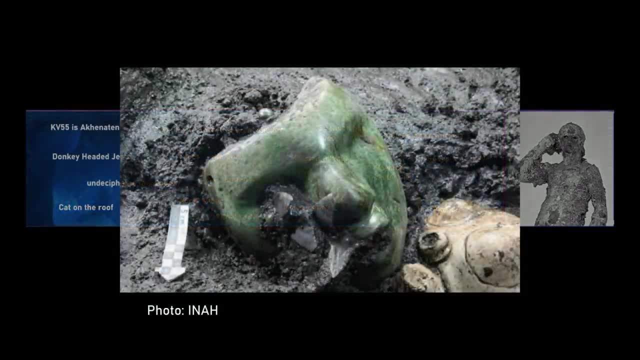 Hey, don't touch that mask refers to an image of a carved green stone mask discovered beneath the Pyramid of the Sun in Teotihuacan, Mexico, back in 2011.. Due to its resemblance to the stone mask in JoJo's Bizarre Adventure and the mask in the mask, a lot of people online joked that. 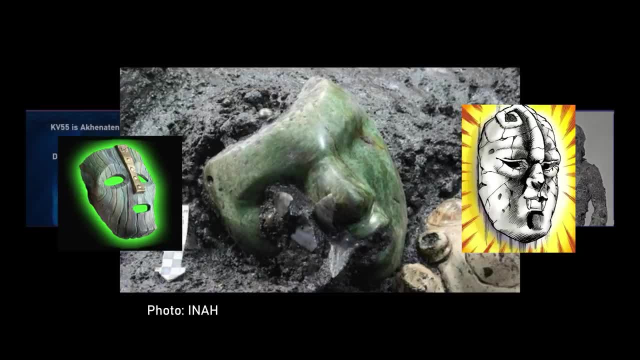 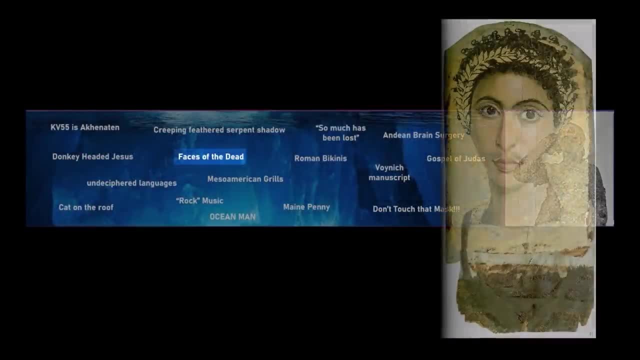 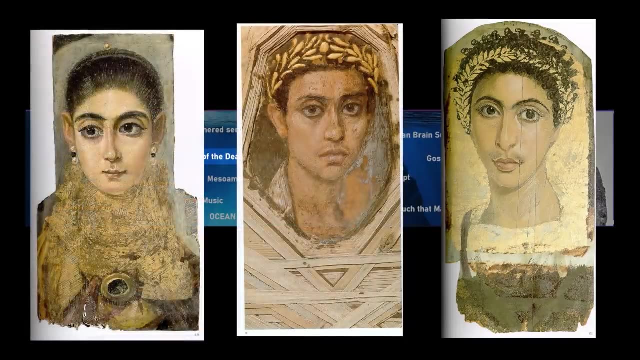 the archaeologists should leave the mask alone, because disturbing it would end the world. Ugh, they might have been right. Faces of the Dead. In Roman Egypt, mummies of people belonging to the upper class were typically buried with highly detailed portraits of their living faces. Many of these coffin portraits have 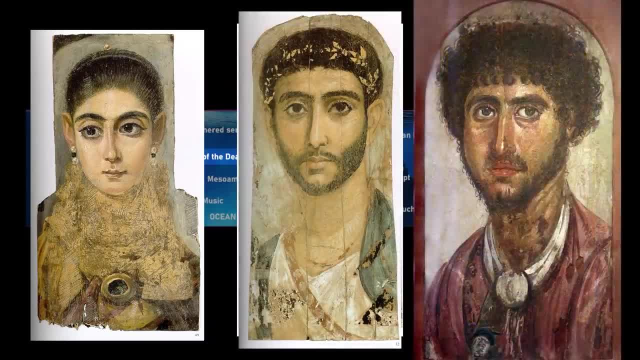 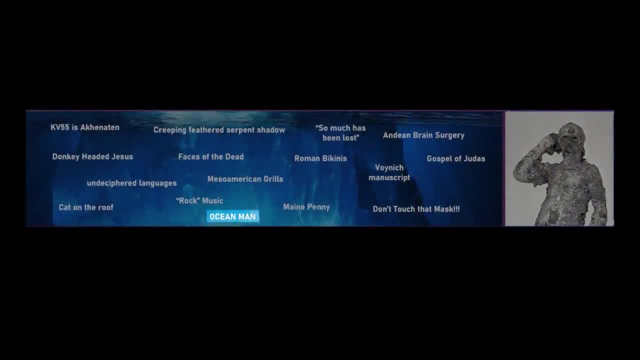 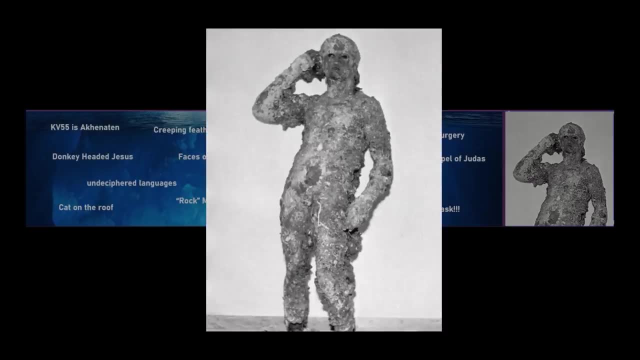 survived us over the centuries and are incredibly lifelike, showing a wide range of facial shapes, hairstyles and personalities. Ocean Man. In the summer of 1964, the nets of an Italian fishing trawler snagged something off the coast of the Adriatic. This was what they found. The fishermen had discovered an 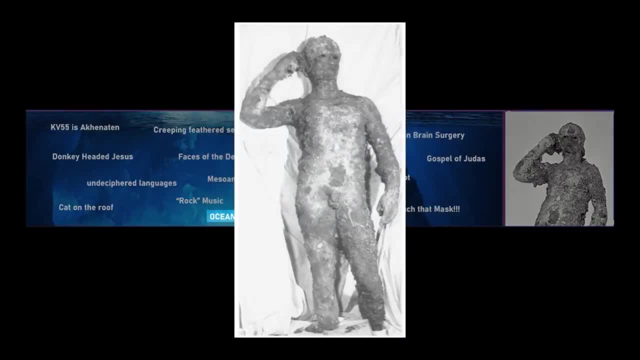 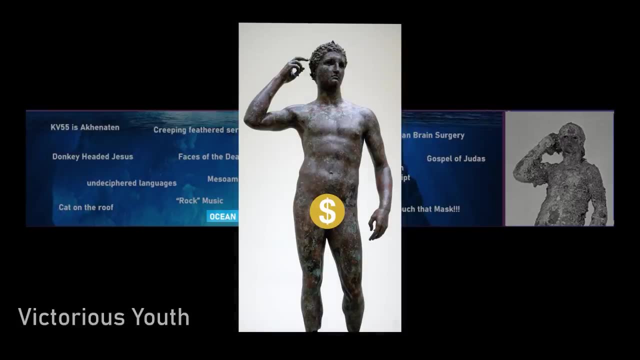 ancient bronze sculpture encased in centuries of patina and sea scum. Extensive cleaning revealed that the statue was a lithe and beautiful athlete, and consequently he is now referred to as the Victorious Youth. The sculpture was sculpted sometime during the Hellenistic. 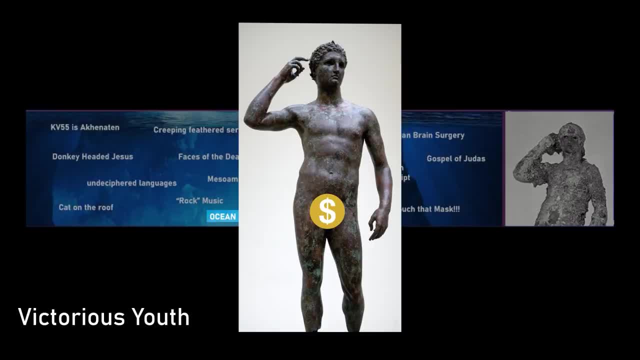 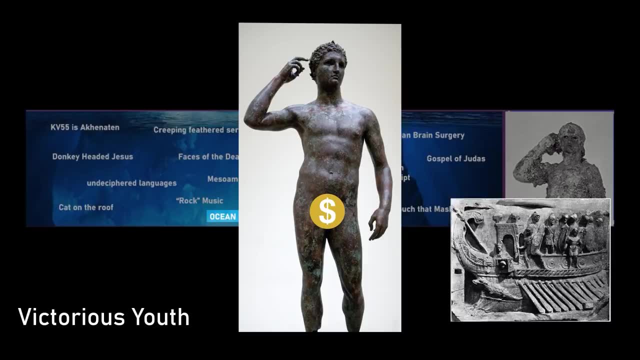 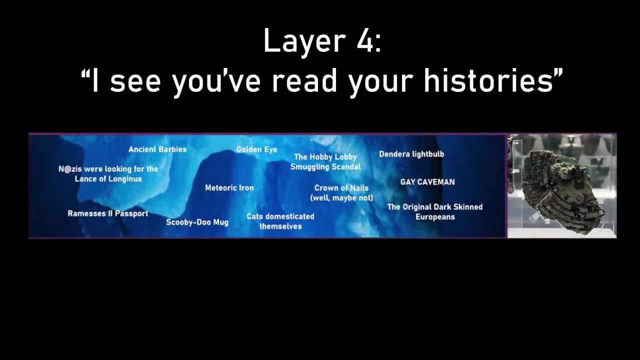 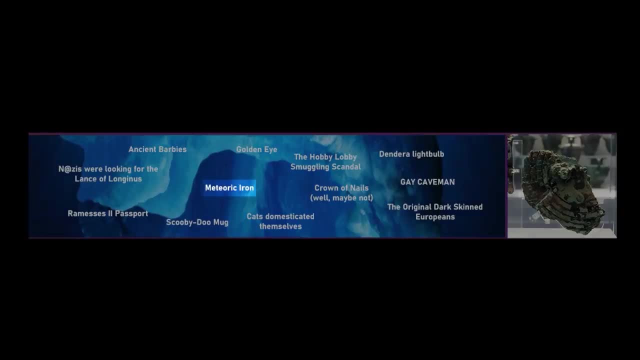 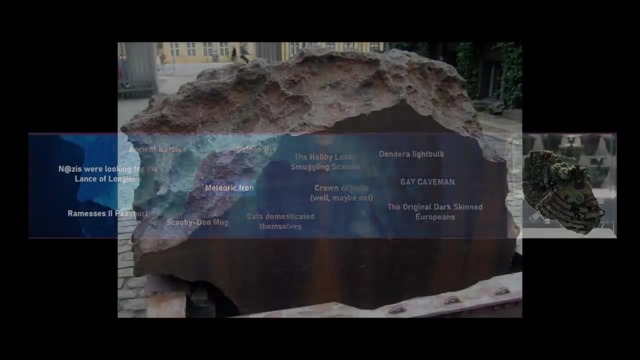 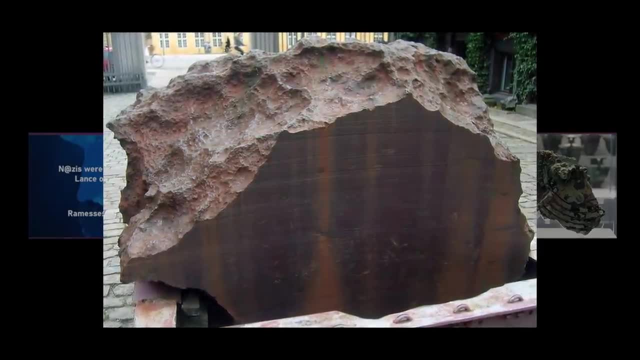 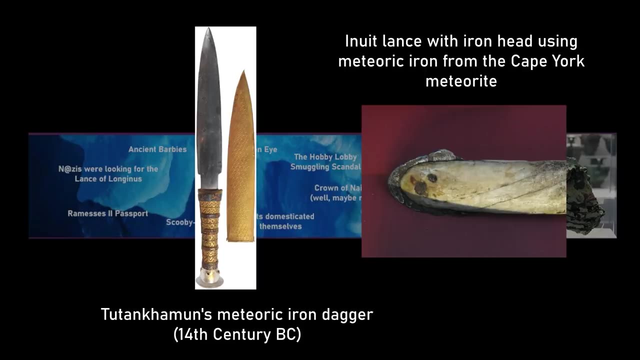 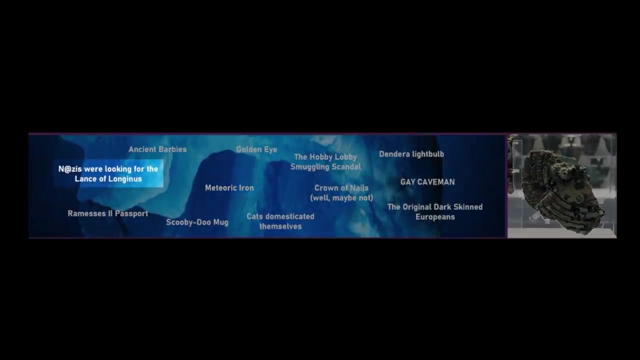 the past, a very rare opportunity to fashion metal tools and weapons. Scientific evidence has shown that artifacts like King Tut's dagger and the spearheads of some Inuit lances were in fact fashioned out of iron harvested from space. rocks fallen from the heavens. Whoa The Nazis took the lance of. 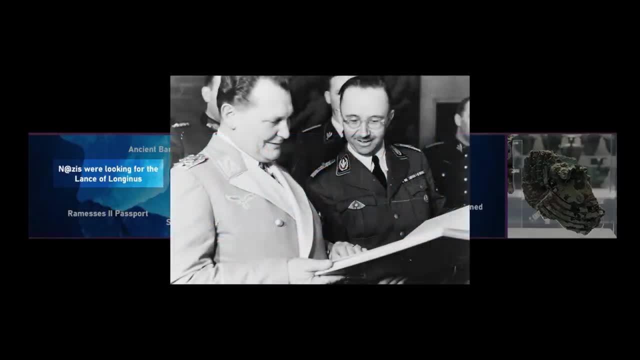 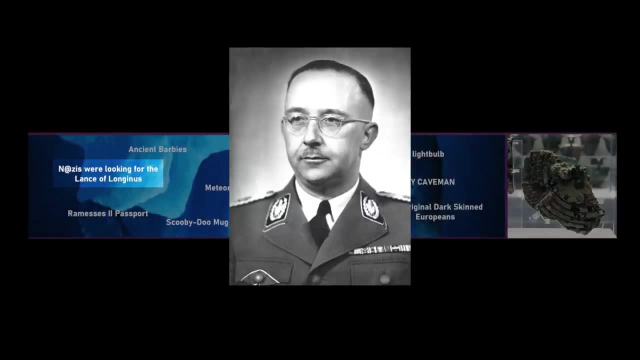 Longinus. During the 1930s, several Nazi leaders took a keen interest in the field of archaeology. Heinrich Himmler greenlit several searches for legendary places and artifacts like the city of Atlantis and the Ark of the Covenant. 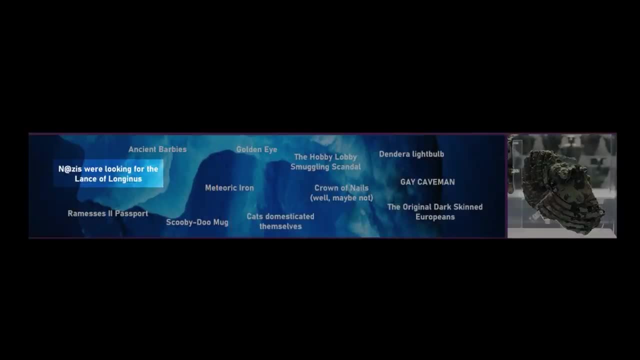 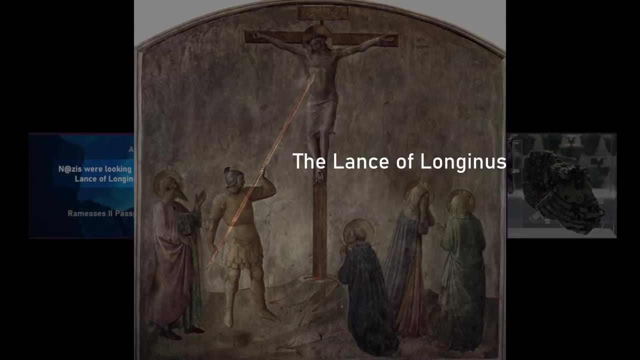 apparently to no avail. One object that was supposedly recovered by the Nazis was the lance of Longinus, or Holy Lance, the spear allegedly used to pierce Jesus's body on the cross. The Imperial Regalia of the Holy Roman Empire dubiously claimed to have acquired the lance of 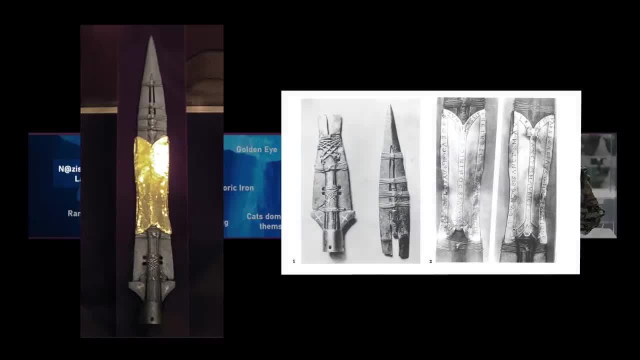 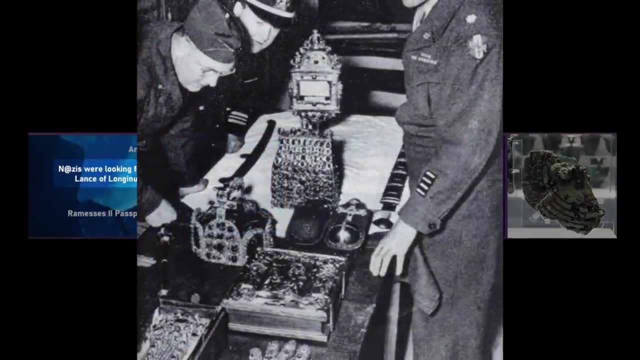 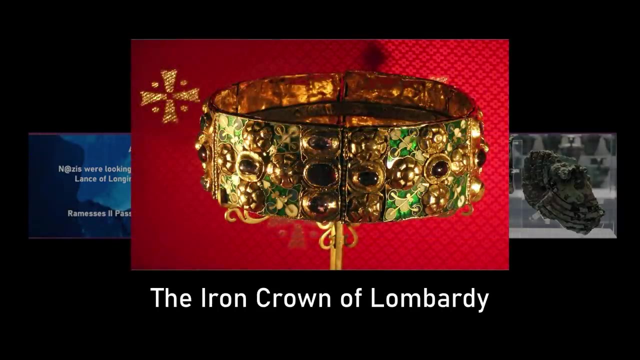 Longinus in the Middle Ages. In 1938, after the annexation of Austria, the relic was brought to Adolf Hitler and displayed in Germany for a short time. After the war ended, however, the Holy Lance was returned to Vienna. Crown of Nails- Well, maybe not. The Iron Crown of Lombardy is a metal crown made 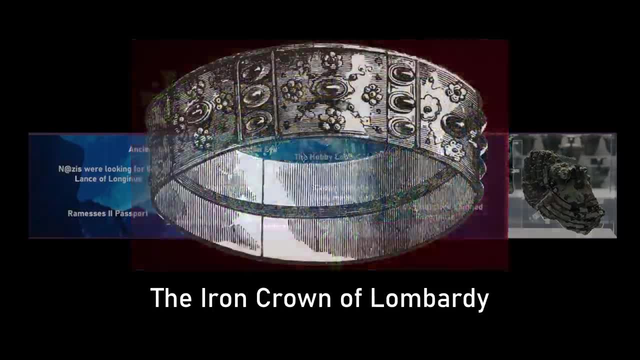 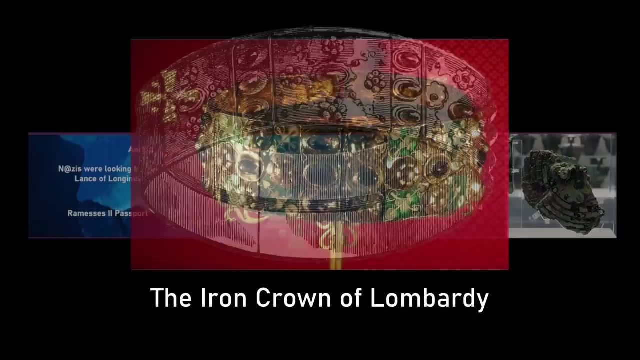 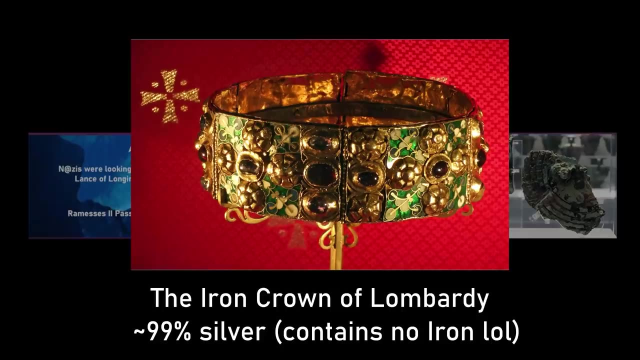 during the early Middle Ages. for a Christian Italian king, A band in the crown was supposedly made from one of the iron nails used in Jesus's crucifixion. However, an examination of the headwear has revealed that it is 99% silver, not iron, meaning the legendary story surrounding it is 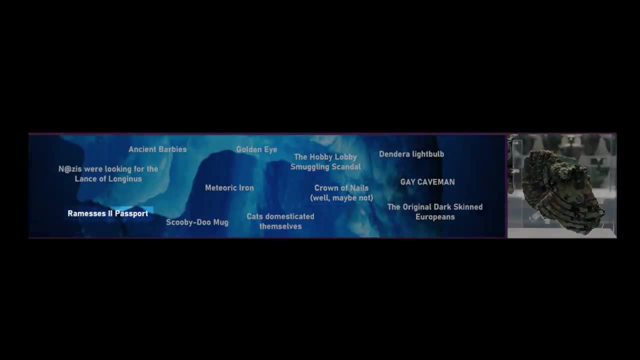 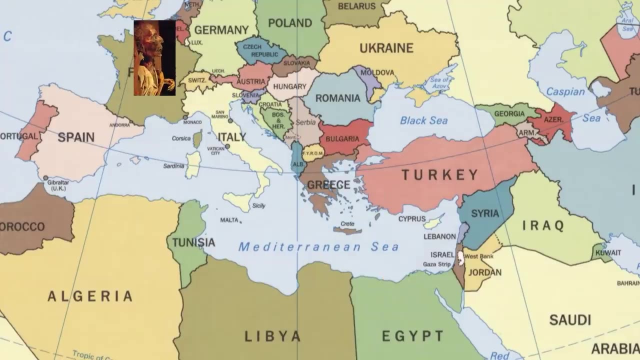 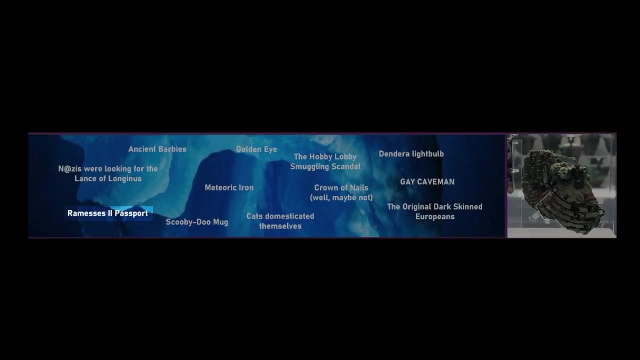 almost definitely false Ramses II Passport. In 1976, the 3,000-year-old mummy of Pharaoh Ramses II was flown from Cairo, Egypt, to Paris, France, so that he could receive a much-needed restoration. A popular internet rumor states that, in order to leave and enter the two countries, 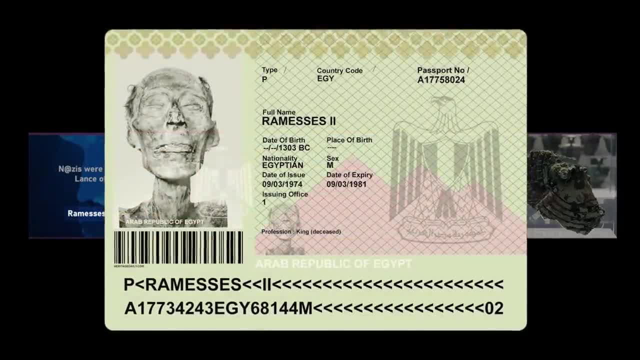 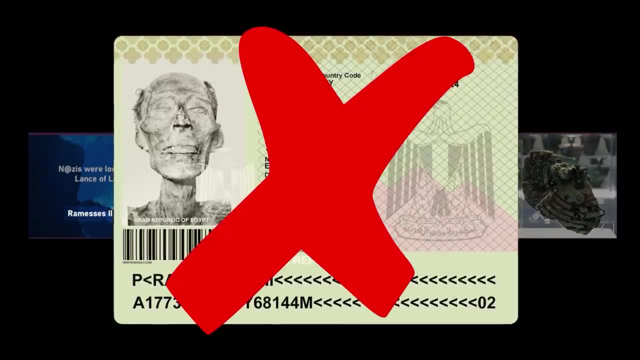 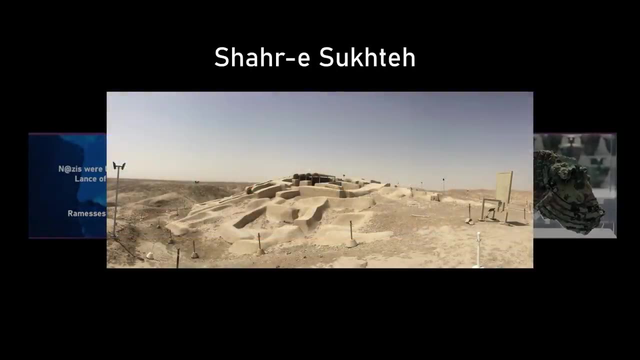 Ramses had to be issued a passport. This is a bit of a half-truth, as, although a lot of paperwork was created for him, an actual physical passport was never produced. This image circulating around on the internet is a clever photoshop. Golden Eye At the site of Shari Sukte, a skeleton belonging to a woman possesses the. 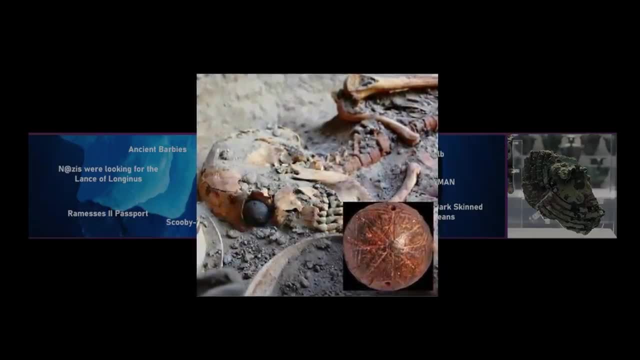 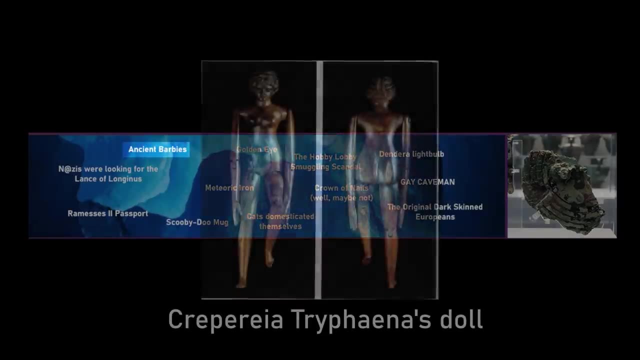 oldest artificial eyeball ever found. The eyeball was covered in a thin layer of gold and was worn regularly while the woman lived. Ancient Barbies, Ancient dolls for children, have been discovered at several archaeological sites around the world. Ancient Barbies, Ancient dolls for children, have been discovered at several archaeological sites around the world. 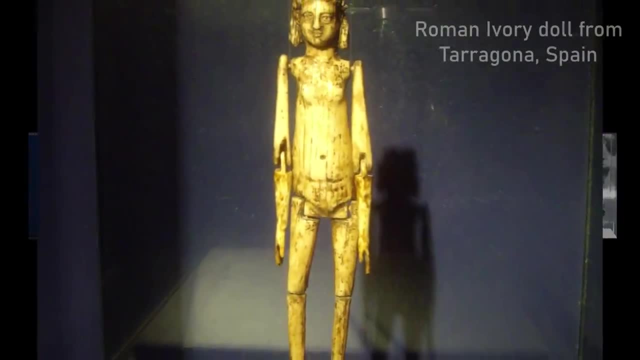 Some are all incredibly creepy-looking- They were cried-man-like consoles, компьютered dolls. Some are actually HYPERVALENT dolls and incredibly similar to modern Barbie dolls, with Posable limbs and decorative clothes that can be swap-ed out. 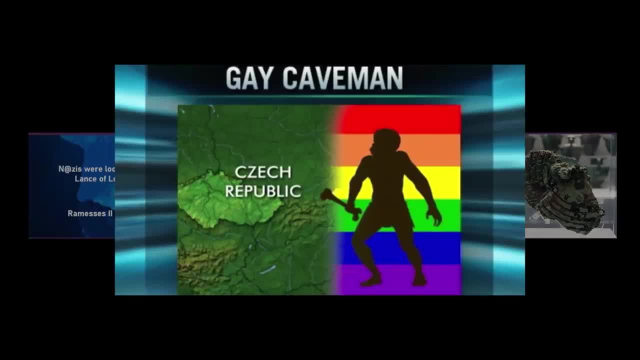 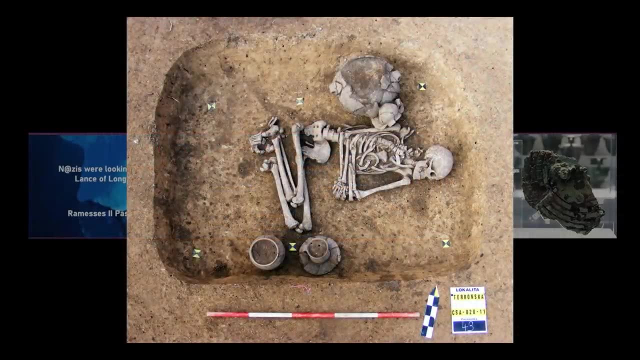 rappelling gay caveman lady. This was an incredibly bad piece of journalism, gay caveman, okay. so in 2011, in the Czech Republic, archaeologists uncovered a prehistoric skeleton that appears to have been biologically male, but had been buried in a ceremonial manner. 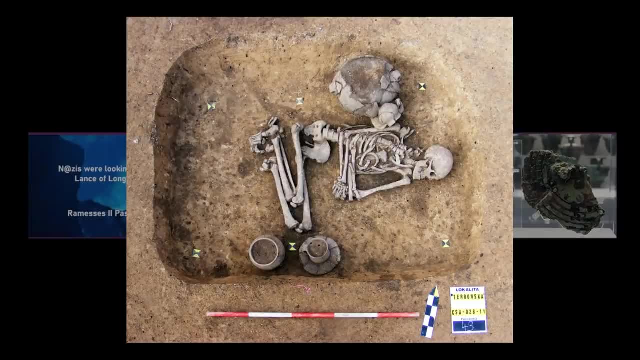 that was typically reserved for females in this society. This led the archaeologists to speculate that this individual, very 57-year-old Bastard, Angela's mother, should be silent. levada is not a very clear citizen who had never read a book before. however, the archaeologist right easiest to read even a young hermit- didn't know that this was important, Only people interested in the cause of her killing. 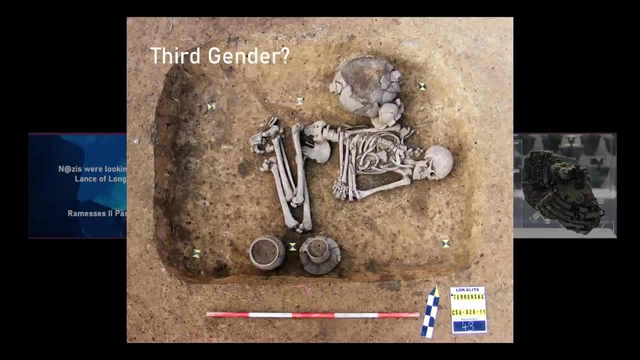 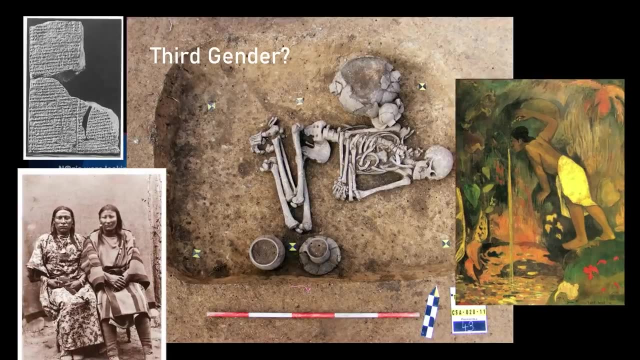 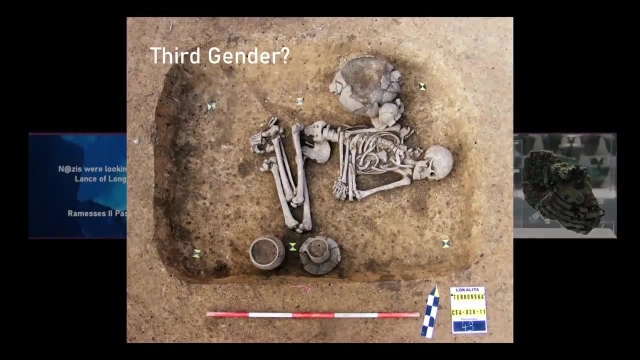 might have represented an example of a third gender or an individual with a gender role that was neither wholly male nor wholly female, something common in many cultures throughout history. Third gender burials like this are actually quite common in archaeology, particularly in North America and in pagan societies. Now, the media totally misunderstood. 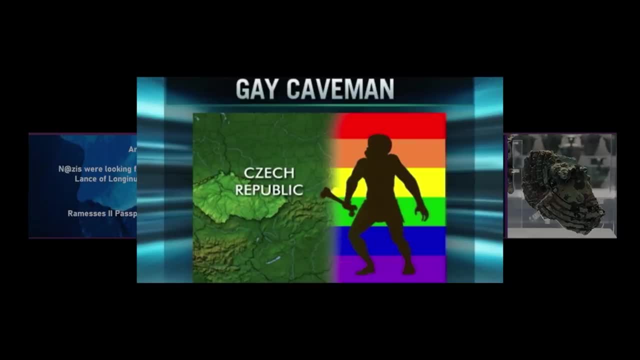 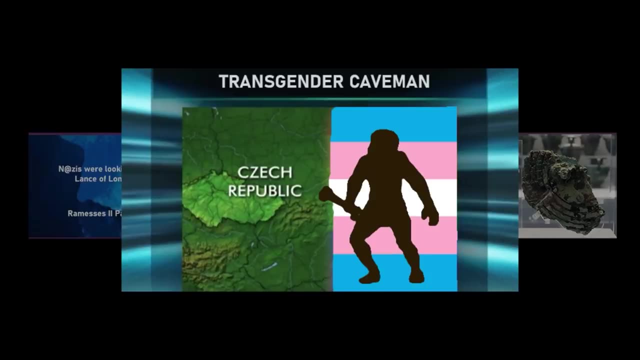 the story. News articles shouted: gay caveman. when the original archaeologist said nothing of the sort. It might be more accurate to think of this individual as a transgender caveman or non-binary caveman. That being said, there are some archaeological finds that might represent: 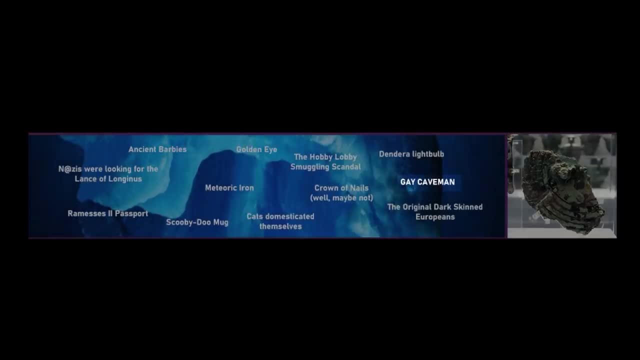 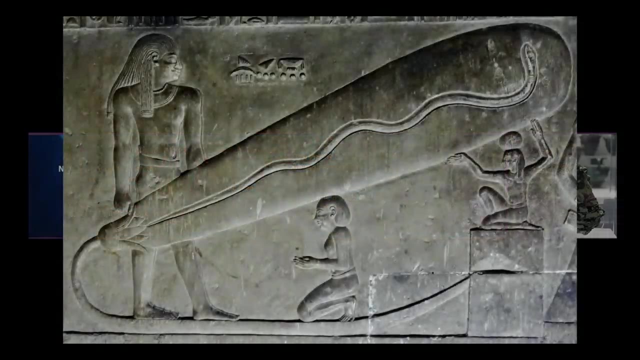 two individuals in same-sex relationships, but as with many things in archaeology, it's hard to know for sure. Dindra Lightbulb: This is a stone relief in the Egyptian temple of Hathor, vaguely resembling a modern lightbulb. The relief is actually a depiction of a scene out of Egyptian mythology. 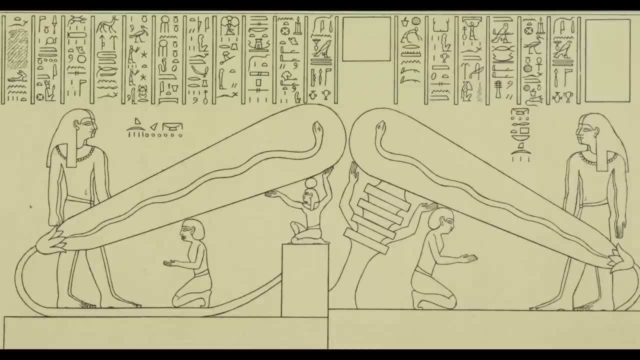 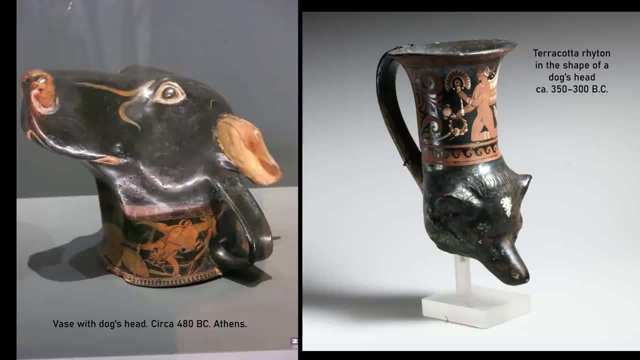 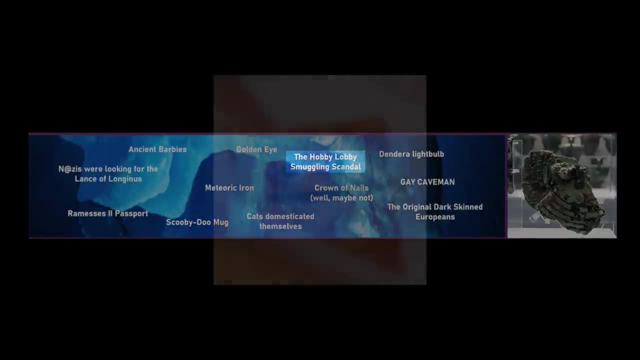 involving a serpent emerging from a lotus flower. The nearby hieroglyphics confirm this interpretation. Scooby-Doo Mug Refers to these really amazing Greek terracotta vases made in the shape of realistic dog heads. The Hobby Lobby Smuggling Scandal. Whoa boy, this is quite the doozy. 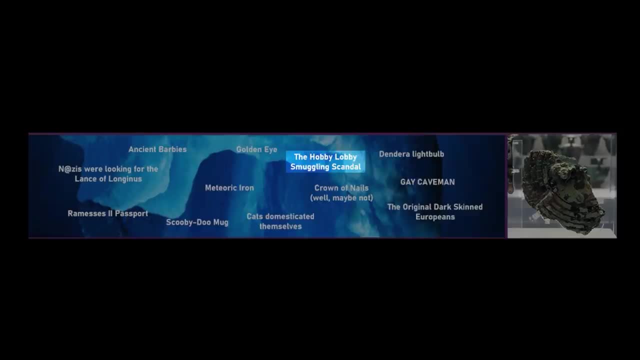 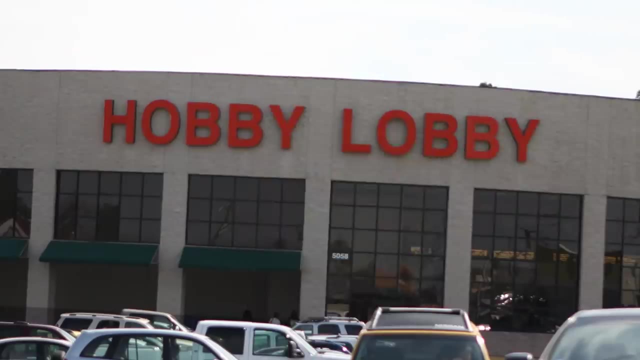 Okay, so starting around 2009,, representatives of the popular arts and crafts store chain Hobby Lobby, you know that store. your grandma gets her minion stickers and scented candles from purchased $1.6 million worth of ancient Iraqi artifacts from dealers in the United Arab Emirates. 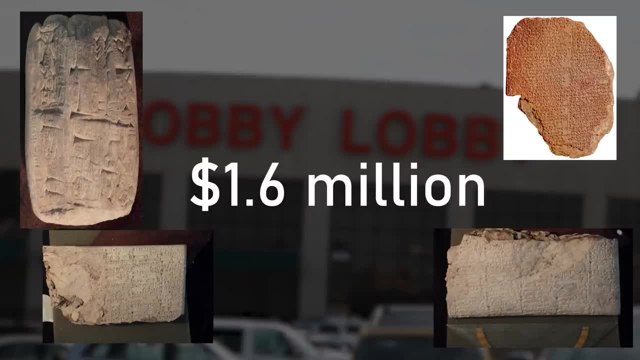 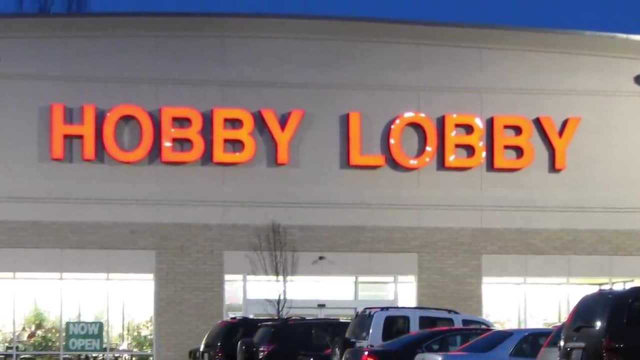 Literally thousands of Mesopotamian cuneiform tablets and cylinder seals. The Evangelical Christian Green family, the owners of Hobby Lobby, wish to put many of these artifacts on display in their Museum of the Bible, A museum that has often been criticized for its- let's just say- lenient. 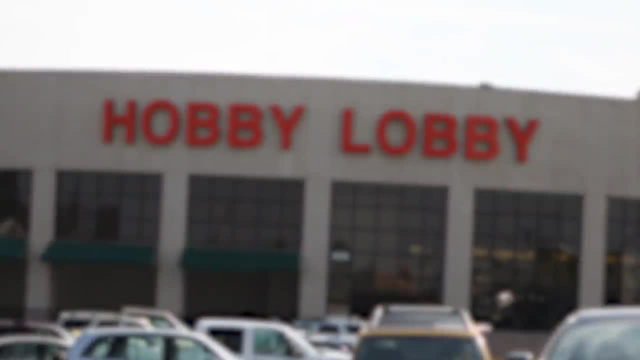 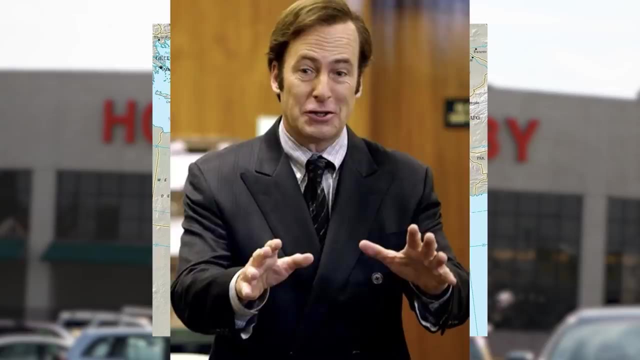 views towards historical accuracy. Now you might be wondering how these artifacts from Iraq ended up in a completely different context, And I'm happy you wondered that, because Hobby Lobby, allegedly sure as heck didn't. As it happens, the majority of the items lacked much, if any, supporting documentation of their 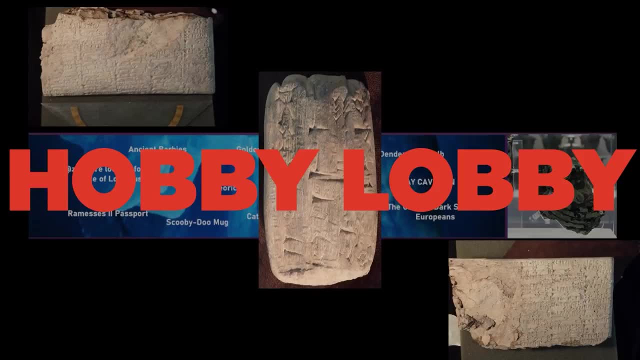 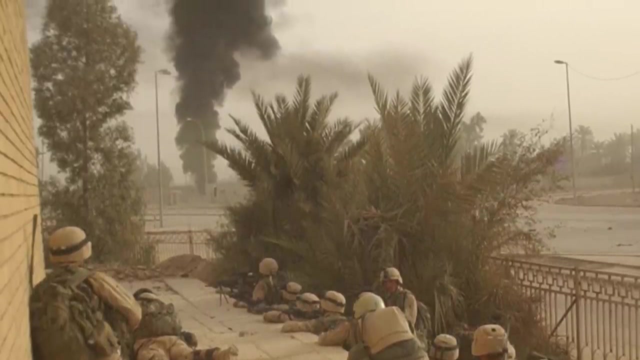 past ownership, which is crucial to ensuring an artifact was obtained legitimately and not through- I don't know- looting. Well, guess what? Hobby Lobby bought over 5,000 illegally looted artifacts. You see, after the American invasion of Iraq in 2003,, the country was left in complete disarray and looters quickly began to. 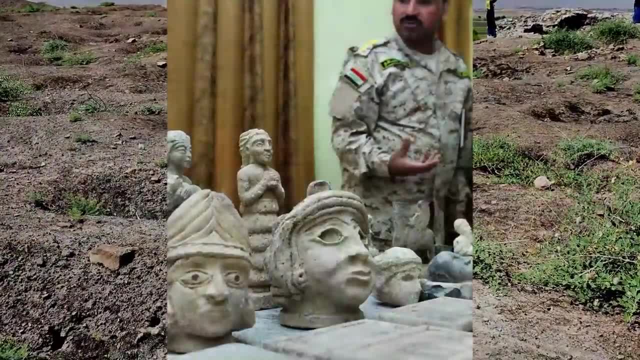 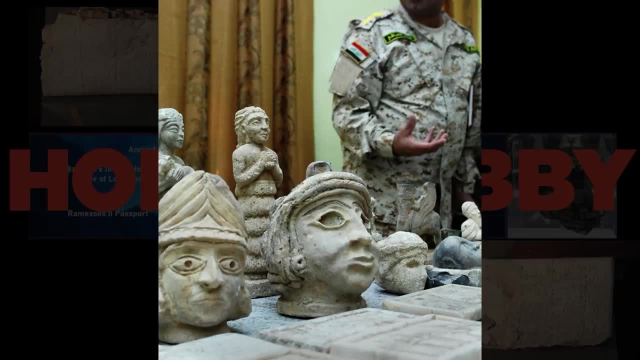 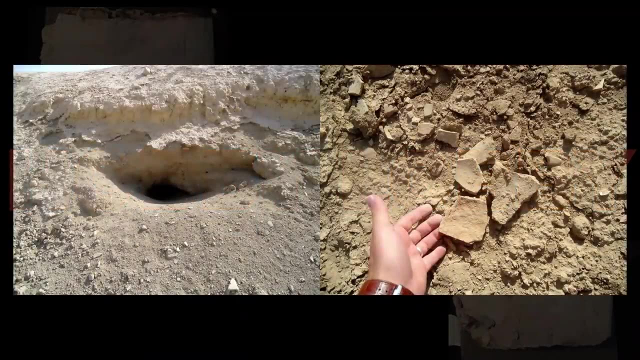 pillage Iraq's archaeological sites and museums, Selling the stolen artifacts to dealers on the black market. These items would then resurface outside the country, their shady origins left unquestioned by future buyers. We know that some looters were just local civilians just trying to make money to feed their families. 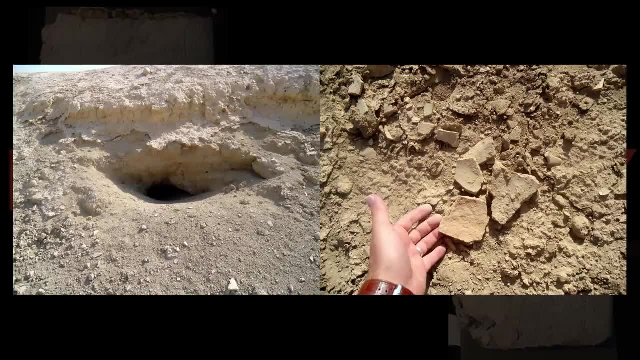 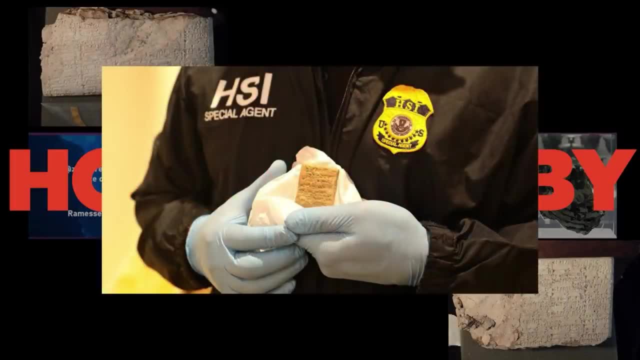 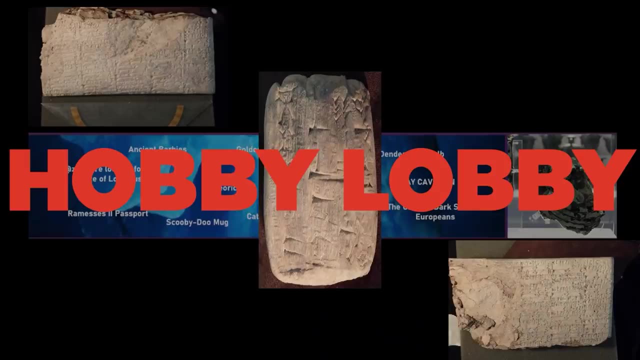 However, others have been connected to more malicious organizations. In 2011,, US Custom Agents seized several shipments of Hobby Lobby's artifacts after correctly suspecting that they had originally been acquired through illegal means. Now it is uh debatable if the parties involved 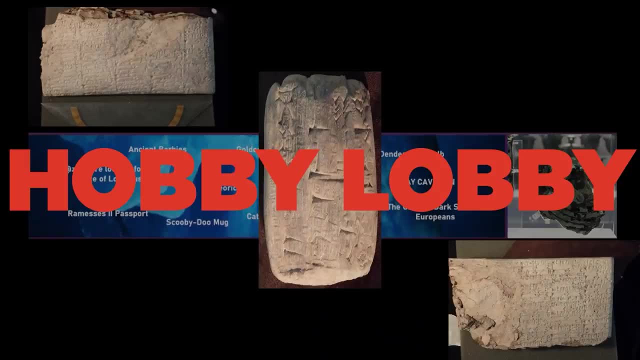 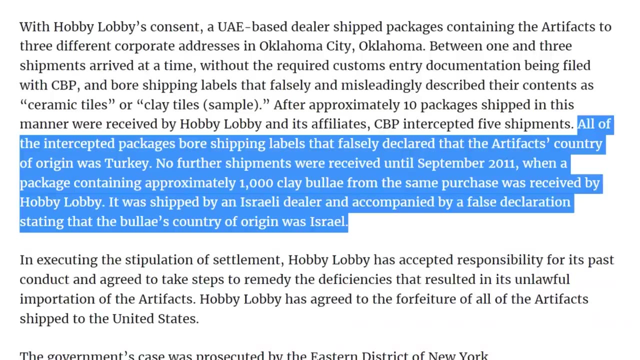 were aware of the illicit origins of these artifacts, but let's just say that they had been, uh ahem, accidentally mislabeled in custom declarations as ceramic and clay tile samples from Turkey and Israel, and not Iraq or the United Arab Emirates. Whoops. 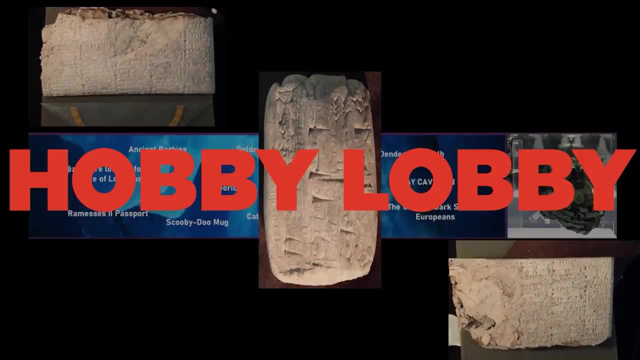 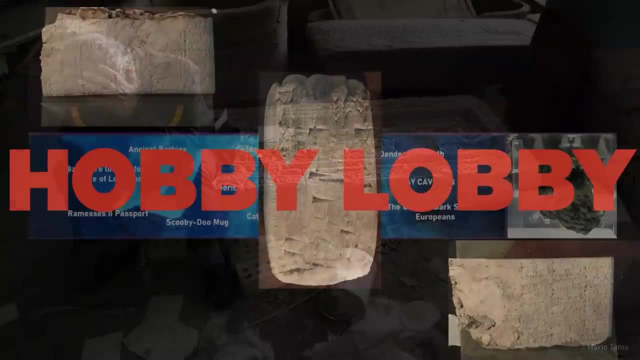 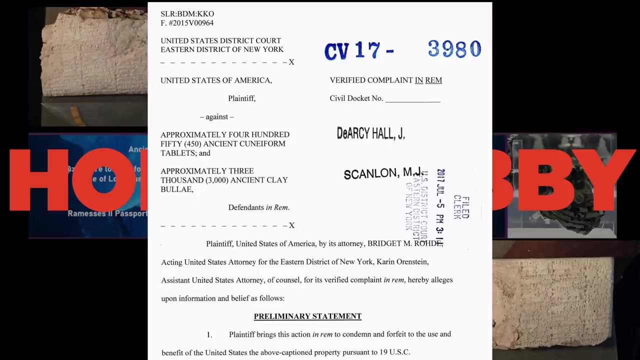 Archaeologists have since determined that several of the pieces Hobby Lobby purchased originally came from the National Museum of Iraq, which was rather violently ransacked less than a decade prior. The United States government prosecuted Hobby Lobby for the scandal and in 2017 the company made a settlement returning more than 5,500 artifacts to Iraq. 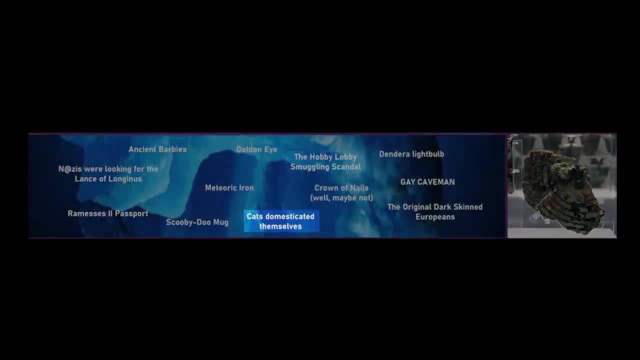 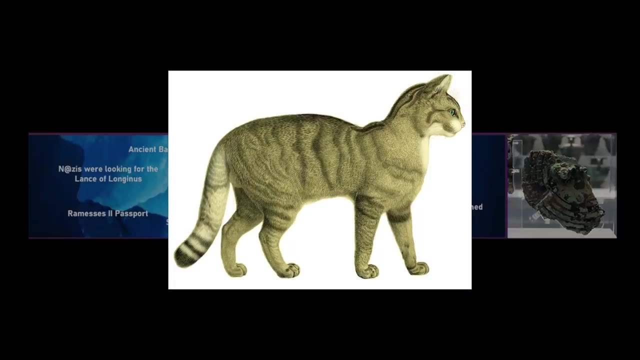 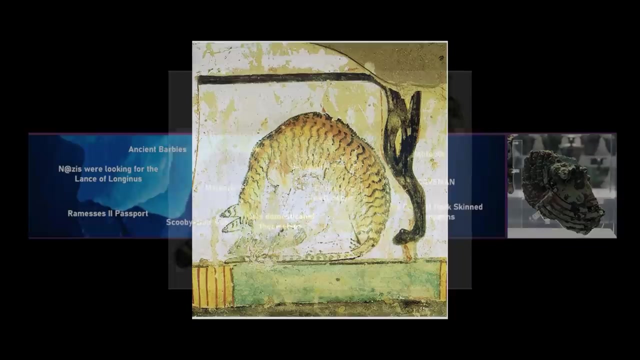 and having to pay a $3 million fine. Cats domesticated themselves. This is a popular theory on how wild cats were domesticated into house pets. They did so themselves. When early human farmers began to create food stores for their exes crops, it attracted mice and other pests Cats drawn by the high concentration of easy prey. 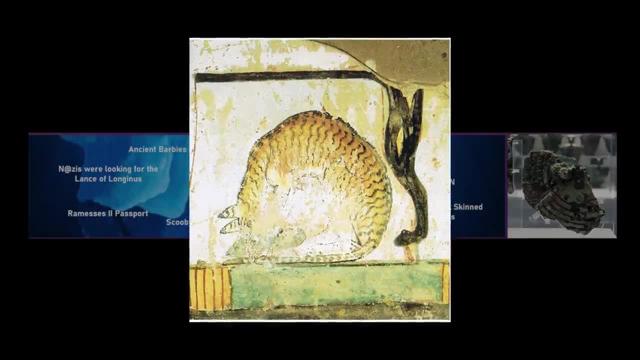 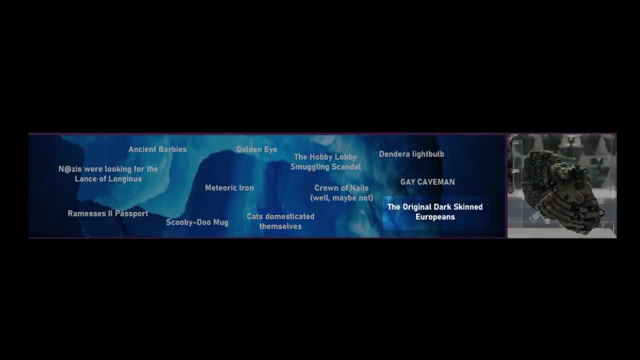 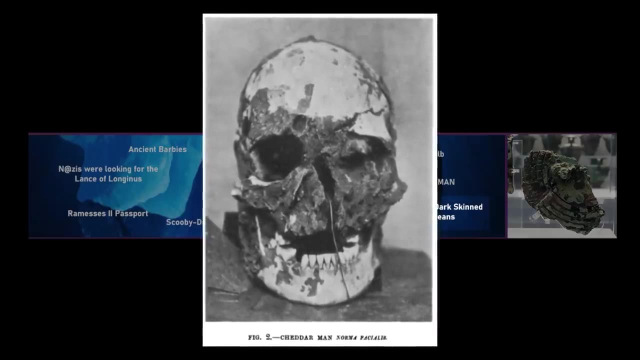 began to live near human houses until gradually, over time, cats learned to live with us and we just kind of let them hang out. The original dark-skinned Europeans. Several genetic studies on prehistoric human remains in Europe have revealed that several of the earliest Europeans looked very different when 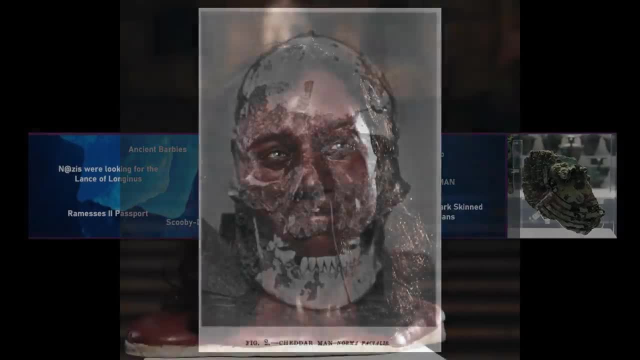 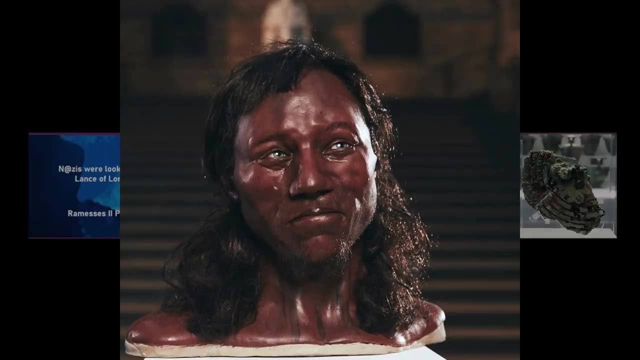 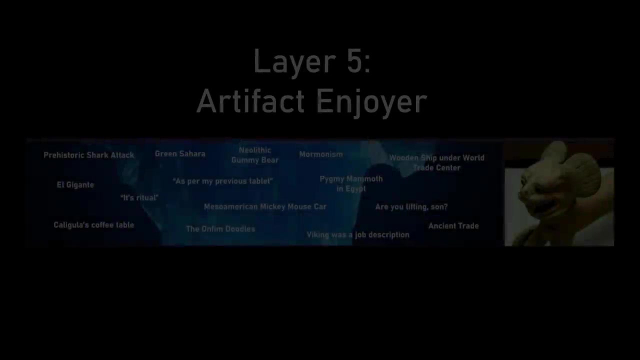 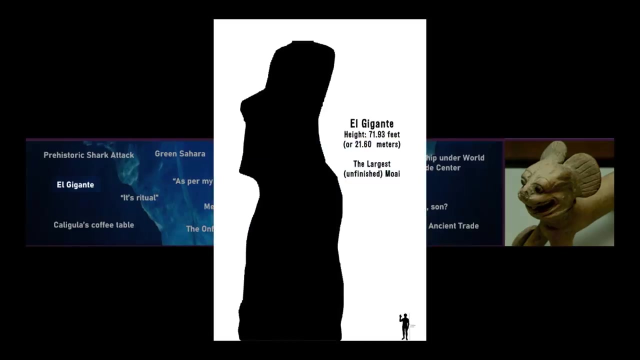 compared to the Europeans of today. Cheddar Man, for example, was a 9,000-year-old man in England who had a dark skin, dark hair and light-colored eyes- El Gigante. El Gigante is the name given to the largest moai. 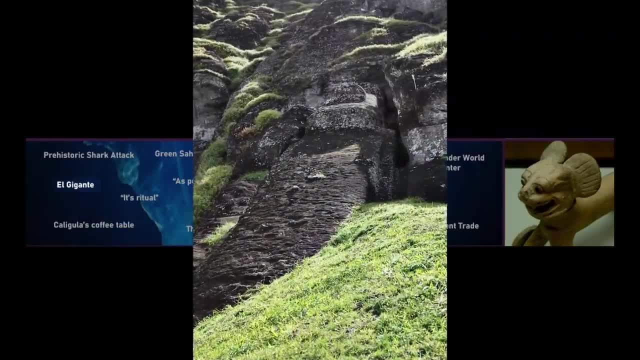 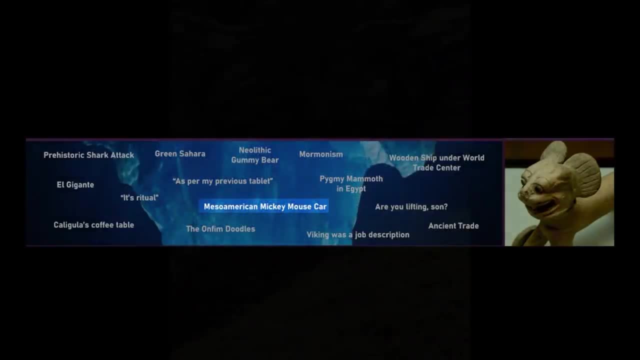 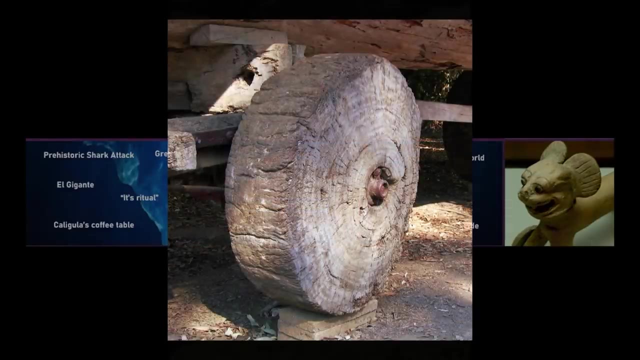 or Easter Island head ever constructed. However, it was never lifted or transported from its original quarry due to the sheer impracticality of its size. The Wheel and Axle are often regarded as one of the earliest and most essential inventions to humanity, as they make transportation, especially over long distances, much easier. 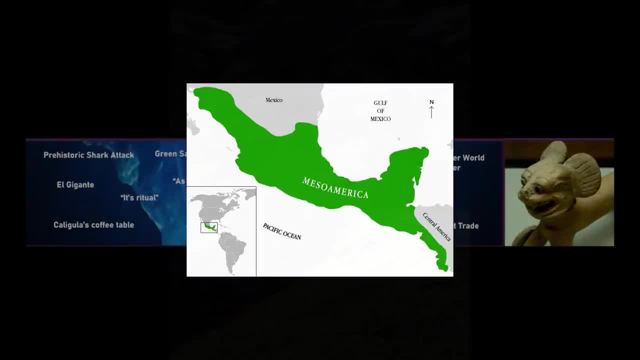 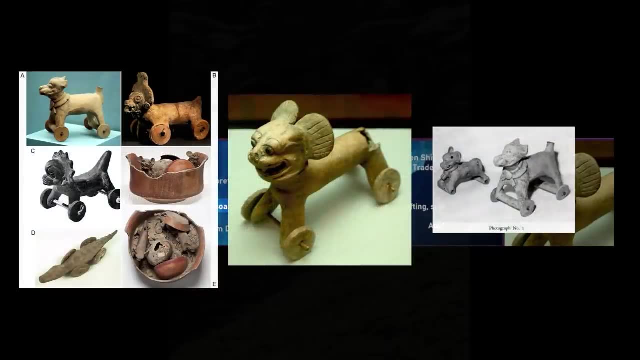 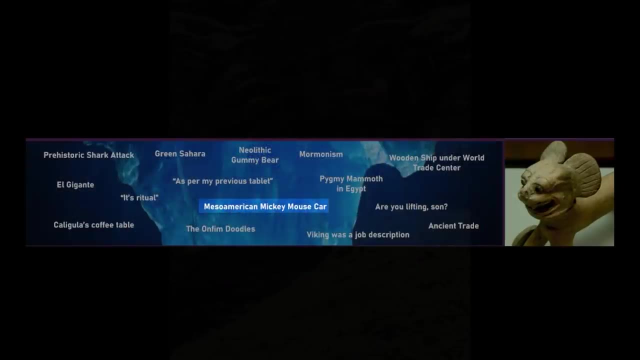 However, in some regions, like in Mesoamerica, it appears that wheels and axles never gained as much prominence. Oh, the Mesoamericans invented them, but appear to have only used them for kids' toys, never incorporating them into larger wagons or chariots. The reasons for this are unclear. 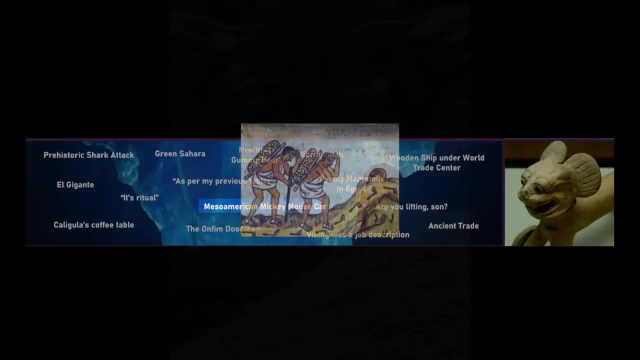 but it appears it might have something to do with the fact that Mesoamerica lacked large domesticated animals to be used as beasts of burden to pull said inventions, so there was little practical use for them. Green Sahara: There was a period in prehistory. 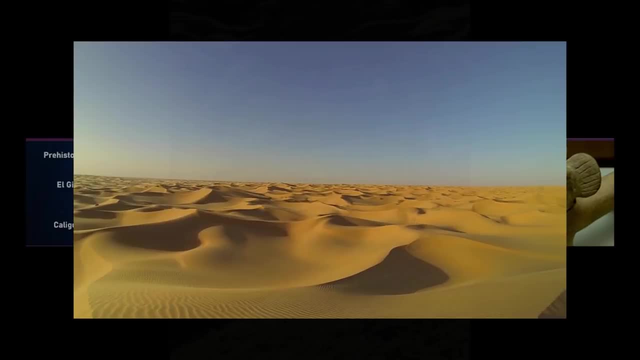 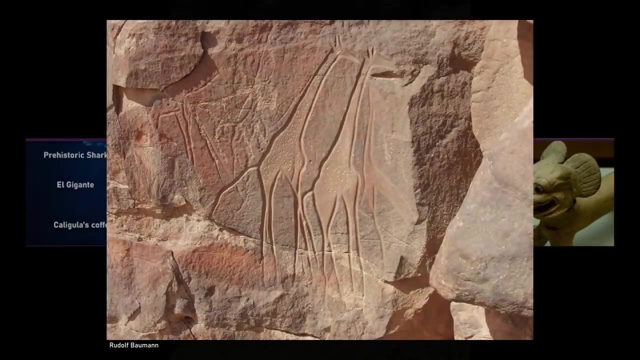 where much of the Sahara Desert, one of the most inhospitable places on Earth, was not a sandy wasteland but once a lush and wet grassland. Evidence of this period exists in prehistoric rock art, showing that giraffes, rhinos, elephants and other animals 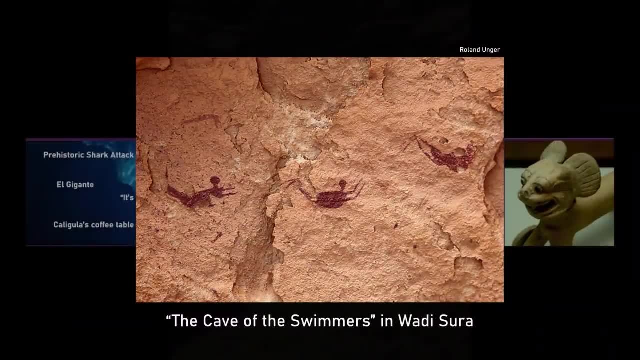 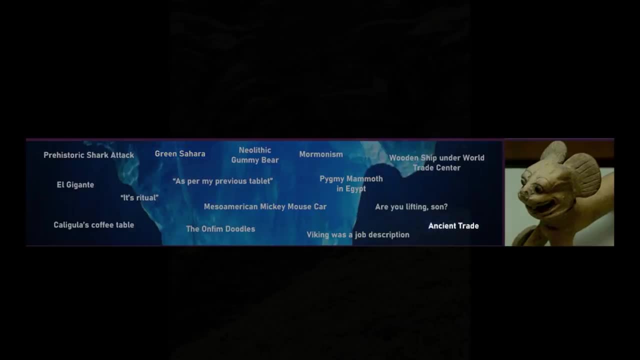 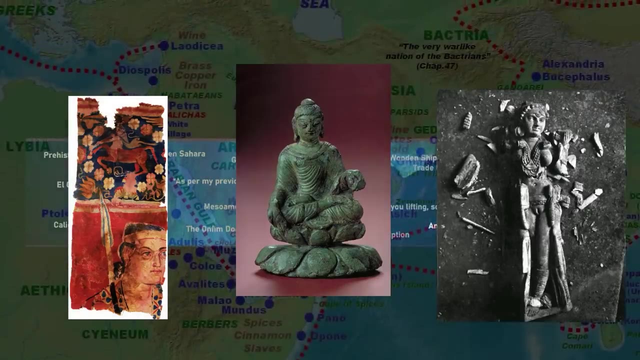 once lived in this region. People swam in freshwater lakes and had thriving communities here, but they died out or moved elsewhere once the desert sands crept in Ancient trade. Several archaeological finds have revealed that the world of the past was surprisingly much more interconnected than often thought, Although it was difficult for a single person. 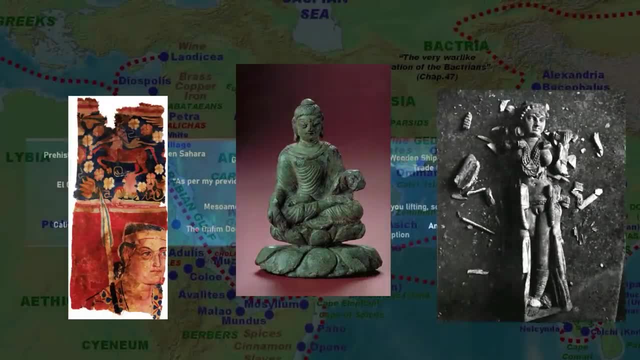 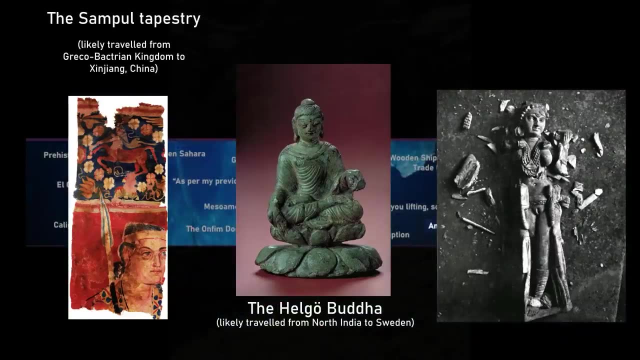 to travel far from home. in these times, objects could travel great distances through a complex network of trade. We've found a Buddha figurine in medieval Scandinavia, Ancient Greek tapestries depicting centaurs in China and carvings of Hindu deities in Roman Pompeii. 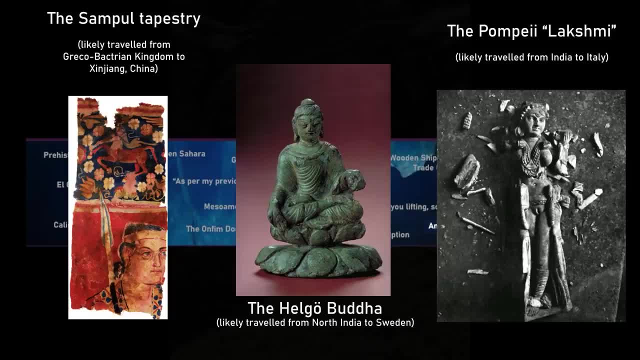 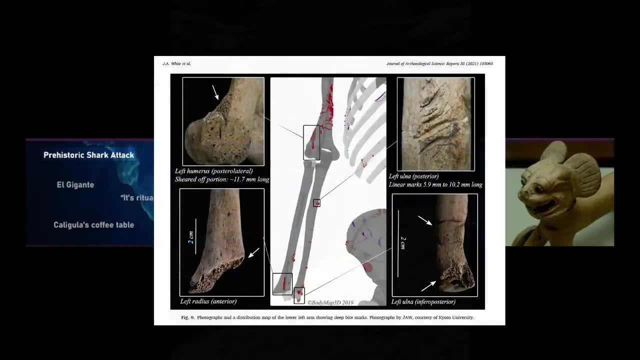 You could get goods thousands of miles from their original locations, but let's just say the shipping times were quite the long wait. Prehistoric Shark Attack. The remains of this 3,000-year-old Japanese hunter-gatherer show that he had been attacked by either a tiger or great white shark at some point. 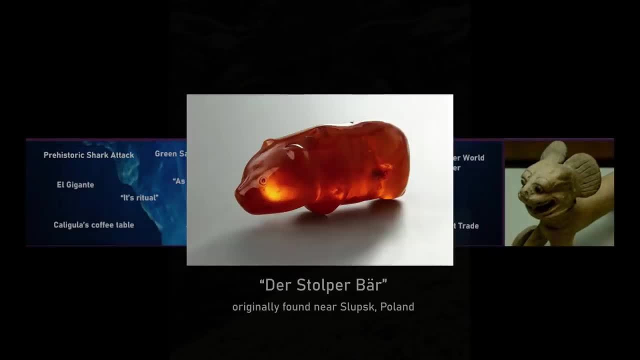 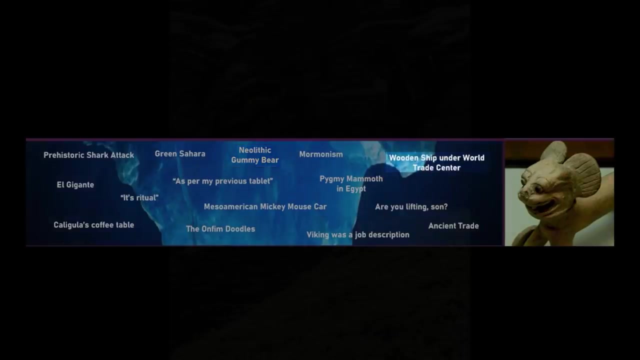 Neolithic Gummy Bear. This amber amulet was found in a Polish bog. Its provenience can't really be a mistake, but it seems like it was dropped by a prehistoric hunter sometime during the Neolithic period. It also looks really uh tasty Wooden Ship Underneath the World Trade Center. 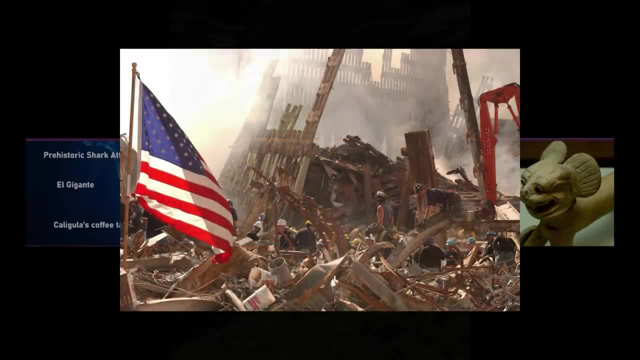 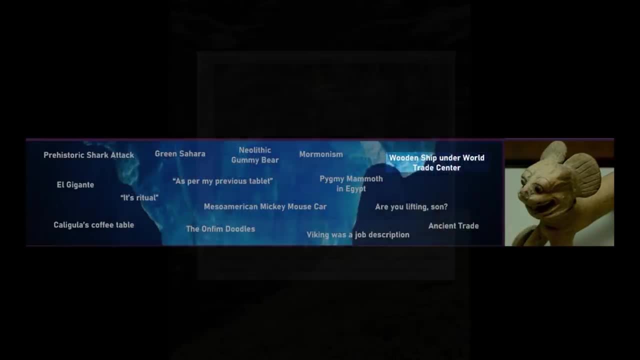 After the September 11th attacks on the World Trade Center in New York, a massive construction effort was made to rebuild the destroyed area of the city In 2010,. an excavation site revealed that 20 feet below the New York City street level. 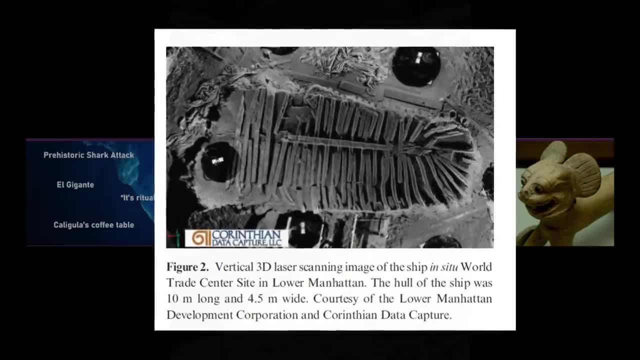 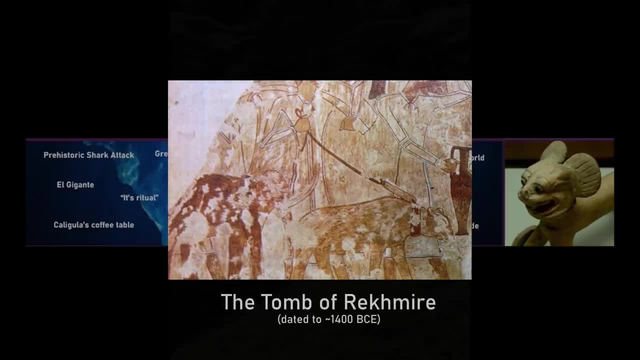 was the intact hull of a wooden ship dated to the 1700s- Pygmy Manor. Pygmy Manor is the largest mammoth in Egypt. There's a mural in an Egyptian tomb, the Rekmurei Tomb, that seems to depict a small hairy elephant on a leash. There is a kind of 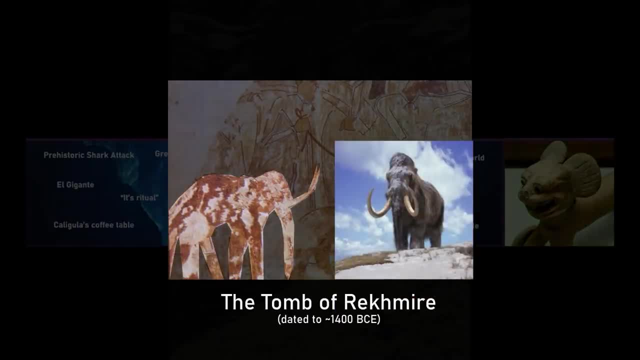 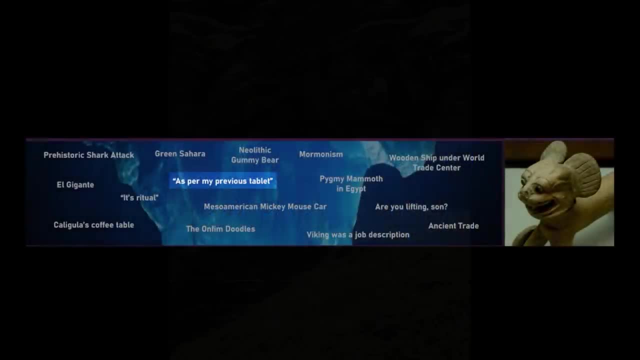 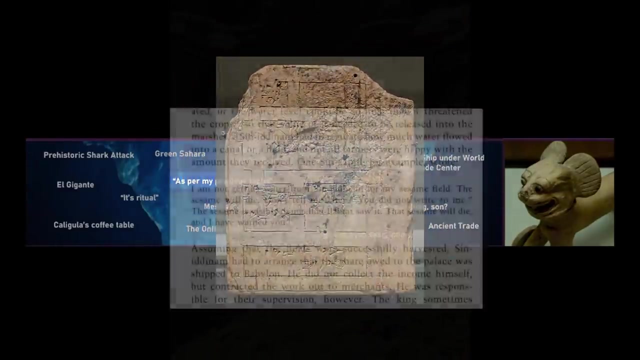 fringe theory that the animal depicted is not an elephant but a woolly mammoth. Although not entirely impossible, this probably isn't the case, As per my previous tablet. 4,000 years ago, a Babylonian administrator wrote a complaint on a cuneiform tablet that reads: 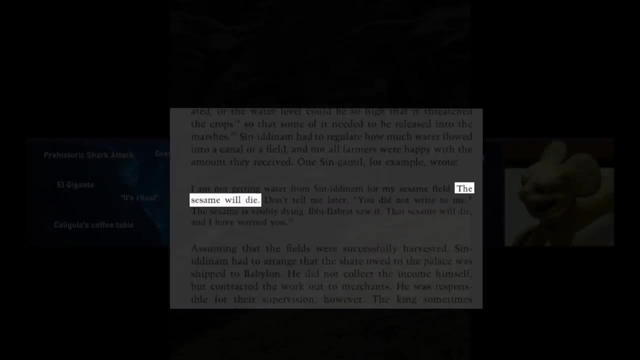 I am not getting water for my sesame field. The sesame will die. Don't tell me later. you did not write to me. the sesame is visibly dying. Ebi Ilaubrat saw it. That sesame will die and I have warned you. 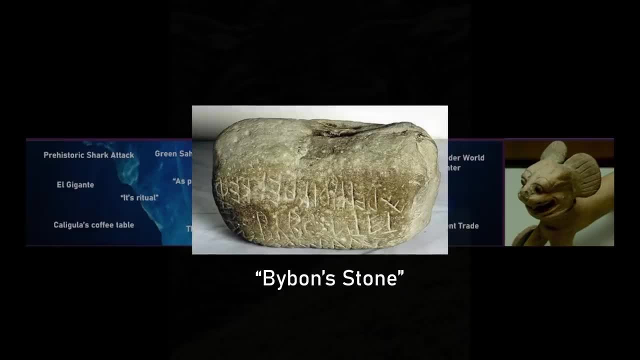 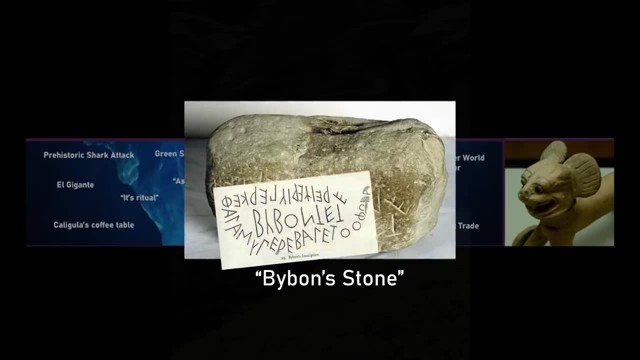 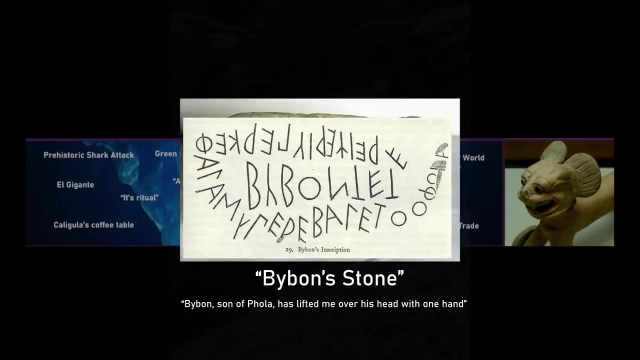 Are you lifting sun? refers to the infamous Bybon Stone, a large block of granite found near Olympia, Greece, and dating to the 6th century BC. The stone has been engraved, presumably by a man named Bybon, with an inscription that reads: Bybon, son of Fola, has lifted me over his head with one hand. 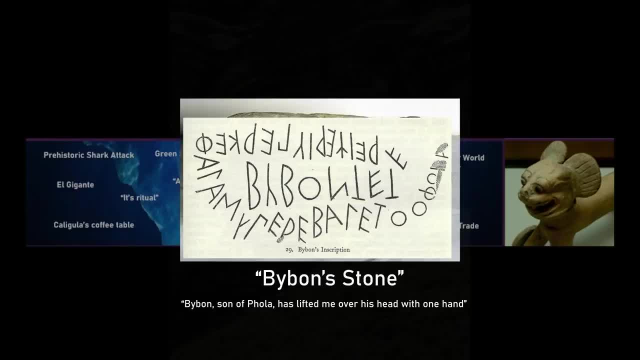 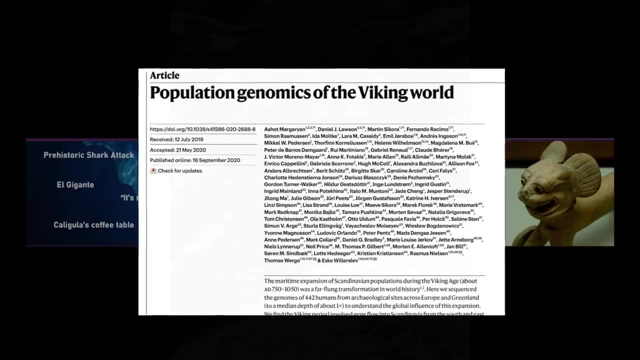 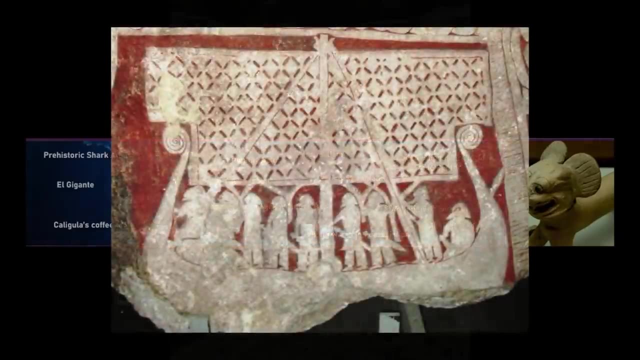 take a moment to appreciate how Bybond wrote his inscription in the first-person perspective of the stone. Viking was a job description. An extensive genetic study of Viking Age remains revealed that the quote-unquote Vikings were an incredibly genetically diverse group and not the necessarily homogeneous people that they were often thought of. They came from all over Europe and it is perhaps better thought of as a job description like pirate or mercenary, rather than an ethnic group. Antfim In the city of Novgorod in Russia: archaeologists. 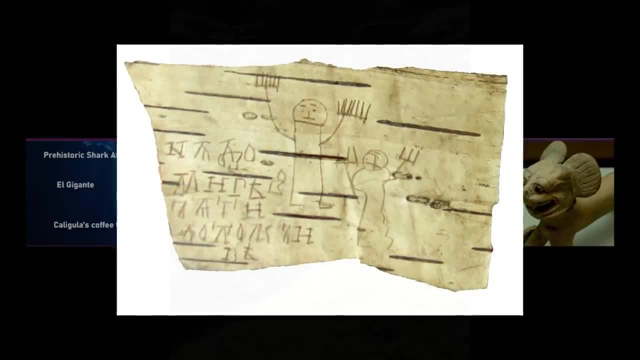 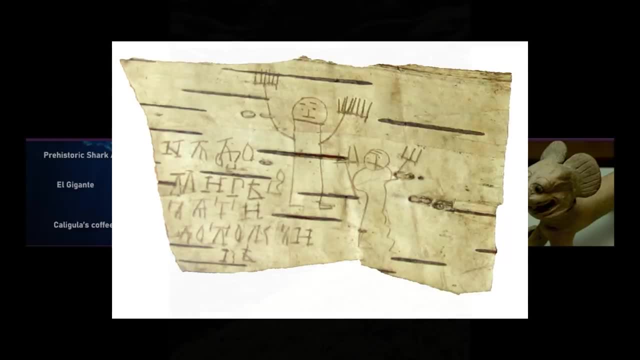 found the spelling homework of a seven-year-old medieval child named Antfim. Antfim was obviously disinterested in his homework, as he doodled all over it. I took a deeper dive into this story in a previous video, so you should check that out. 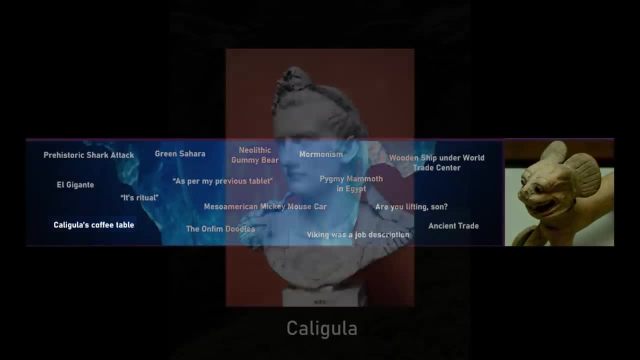 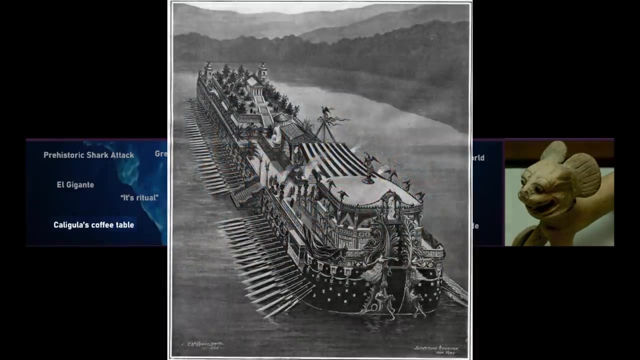 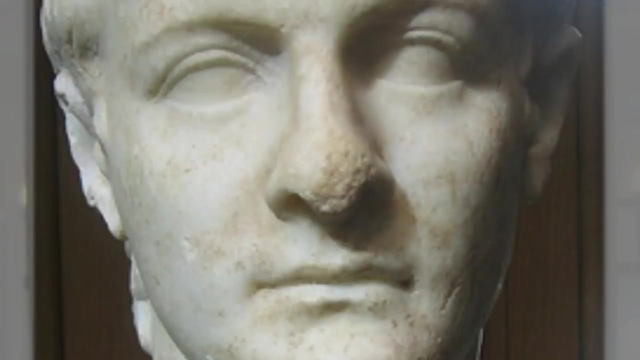 Caligula's Coffee Table. In the first century AD, the notorious Roman Emperor Caligula ordered the construction of two of the largest wooden ships ever built in antiquity. These pleasure barges were some of the most expensive and technologically advanced of their day and were said to host the emperor's lavish parties and orgies. 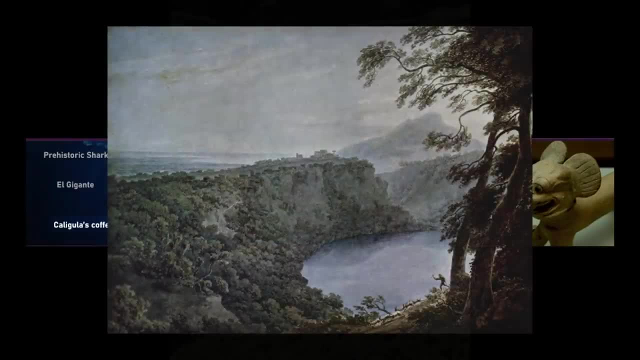 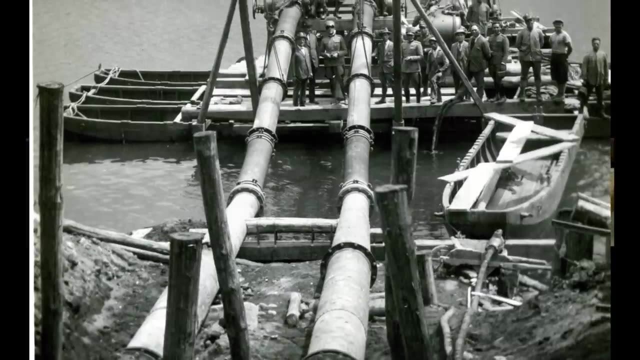 Caligula's fancy ships eventually sunk to the bottom of Lake Nemi, where they remained for almost 2,000 years. In the 1920s, however, Italian dictator Benito Mussolini ordered the lake be drained and the wreckage of the ships recovered. 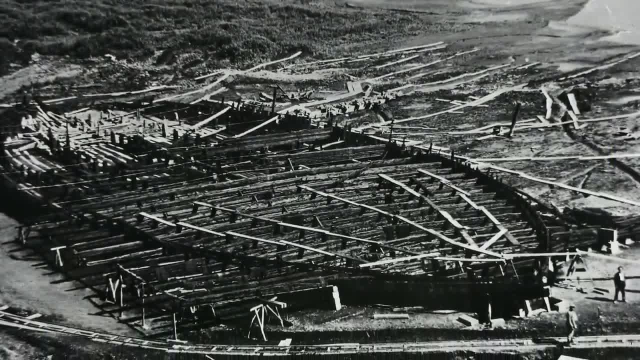 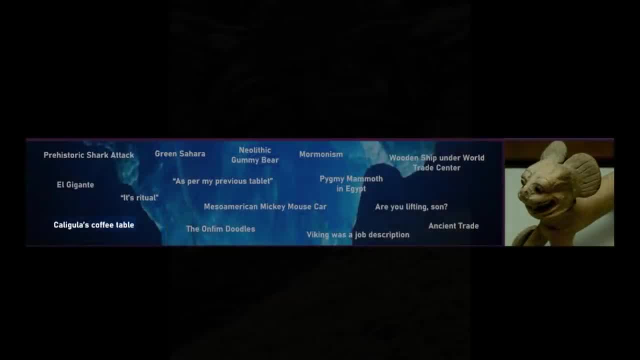 The two Nemi ships were successfully razed and eventually housed in their own museum, But in 1944, an Allied attack resulted in a fire that eventually burned down the museum. Sadly Caligula's Coffee Table In the first century AD, the notorious Roman Emperor. 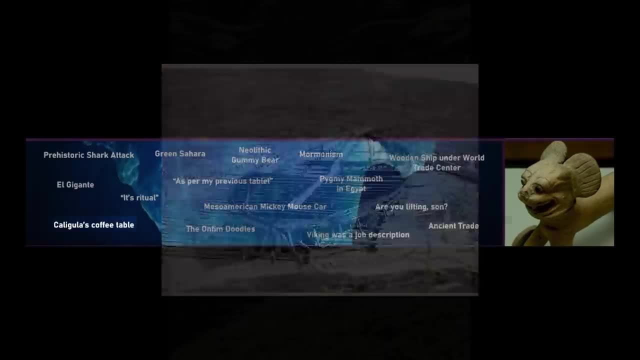 Caligula ordered the construction of two of the largest wooden ships ever built in antiquity. These pleasure barges were some of the most expensive and technologically advanced ships ever built in antiquity. Caligula's Coffee Table. In the first century AD, the notorious Roman Emperor 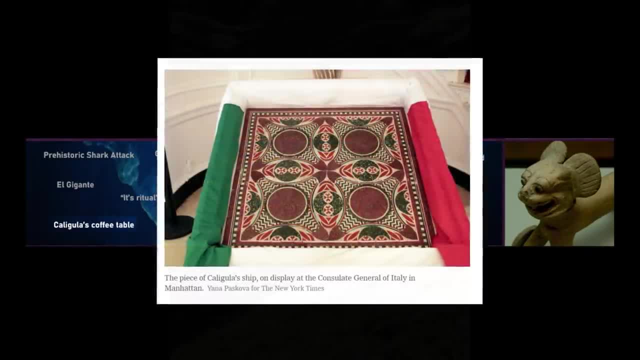 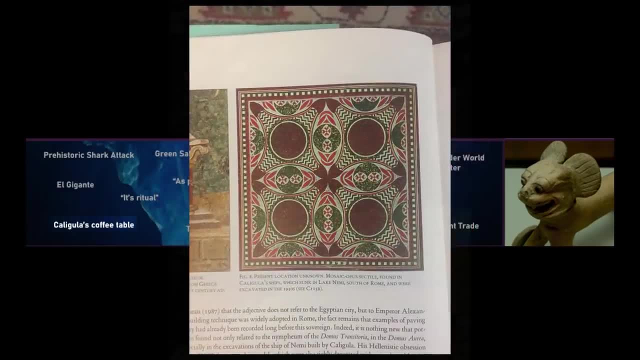 Caligula ordered the lake be drained and the wreckage of the ships recovered. The wreckage of the ships recovered. That was until 2017, when a New York attorney's office confiscated a mosaic panel from a private collector in New York City. The artifact turned out to be a Roman mosaic used to decorate the floor of one of the Nemi. 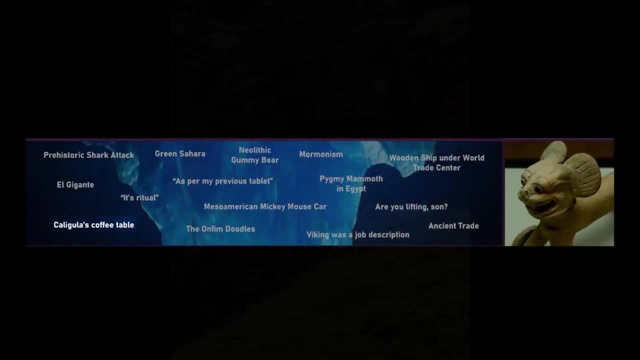 ships Surviving the fire. it had been sold by an Italian aristocratic family to antiquity dealers in America. The owner of the mosaic apparently had no idea how special it was and was using it for a few years as a coffee table. 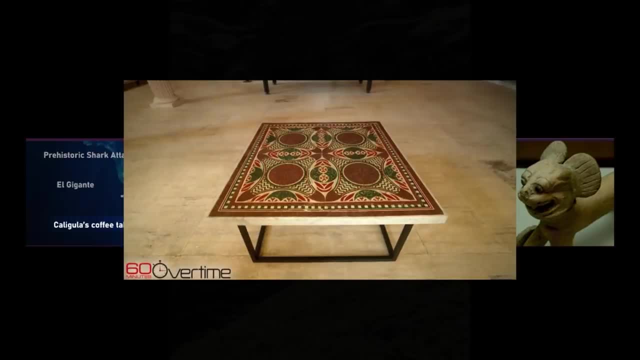 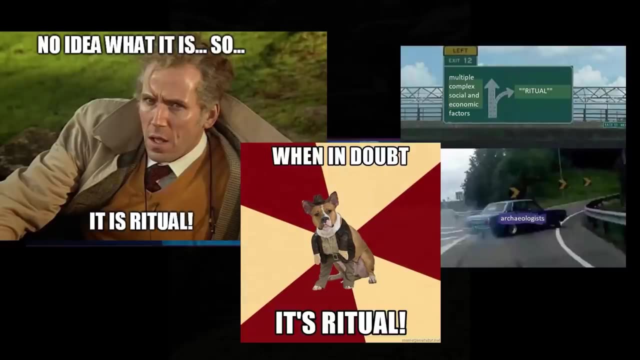 Knowing what Caligula probably did on that ship. I just hope they wiped it down a little before they used it. It's Ritual. It refers to the tendency for archaeologists to explain something like an artifact or burial custom as Ritual, which basically means that 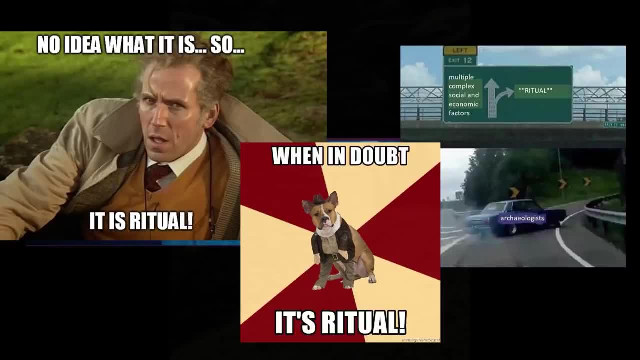 we don't know what the heck this thing is or what it was used for. It's kind of a vague catch-all term that really means nothing. in the end. Brushing your teeth can be considered ritual and a whole bunch of other stuff. Mormonism: The religion of Mormonism is based on the. 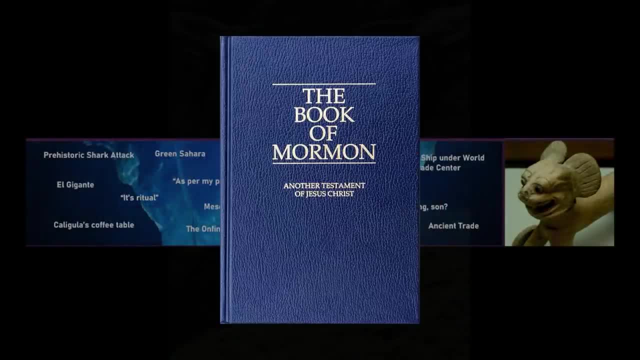 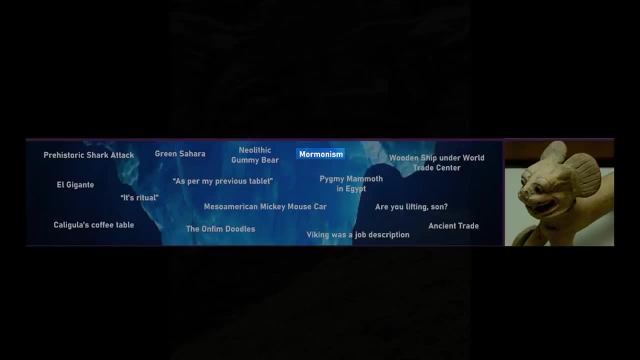 fact that the religion of Mormonism has this kind of weird relationship with archaeology. The founder of Mormonism, Joseph Smith, was a bit of an amateur archaeologist himself. In 1823, Smith claimed to have discovered, with the help of an angel, an ancient book. 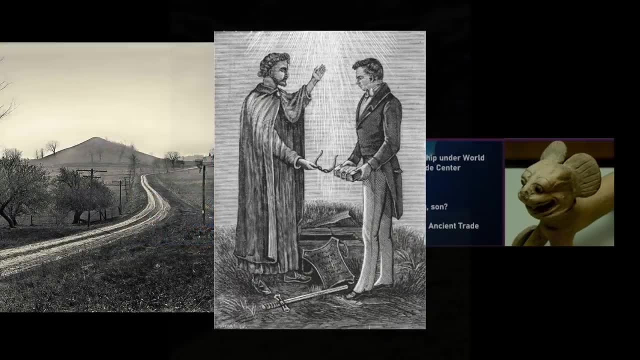 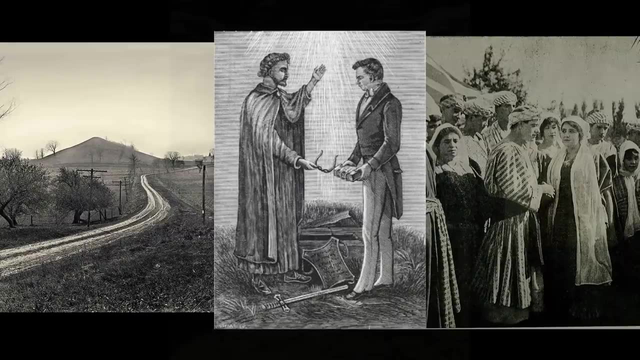 of gold plates buried on a hill in Manchester, New York Smith claimed that they were the remains of a bygone civilization of Israelites called the Nephites, who crossed the Atlantic Ocean in ancient times. Now, with the hindsight of modern archaeology and genetics, this claim of an ancient book 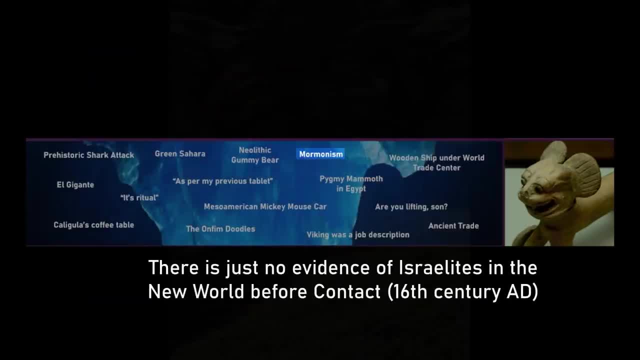 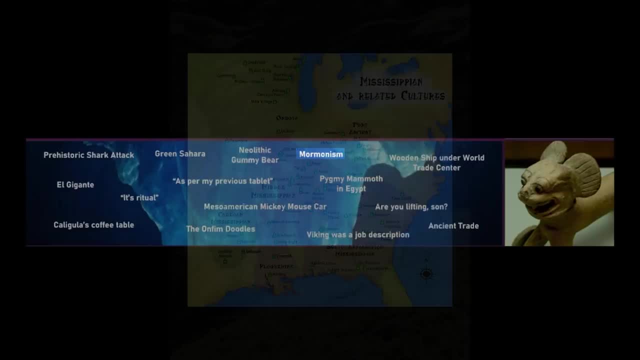 this claim of an ancient transatlantic crossing is simply not supported by the evidence, But it is possible that Smith might have actually uncovered the remains of the very real Native American Mississippian culture which existed across the eastern part of North America from. 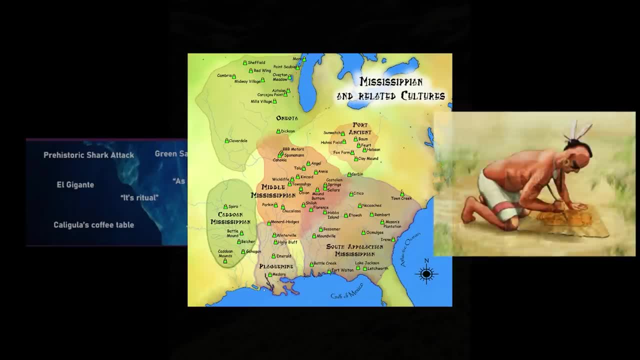 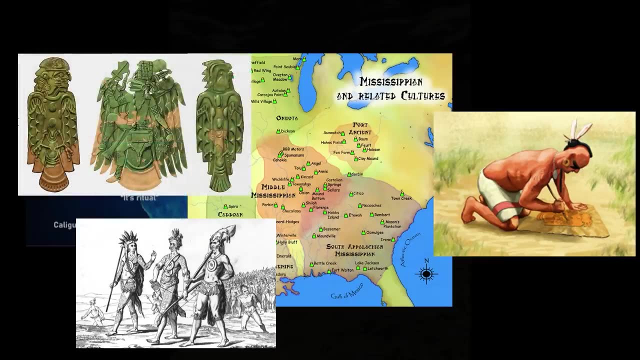 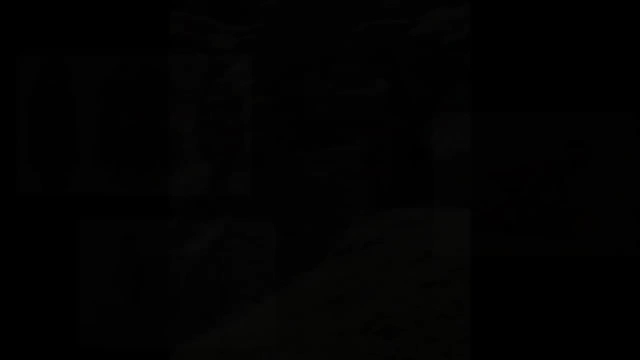 800 to 1600 AD. These Native Americans did know a bit of metalworking and crafted decorative copper plates with glyphs and designs. Perhaps Smith found a few of these copper plates and misidentified them as Israelite altres, The Schliemann level. 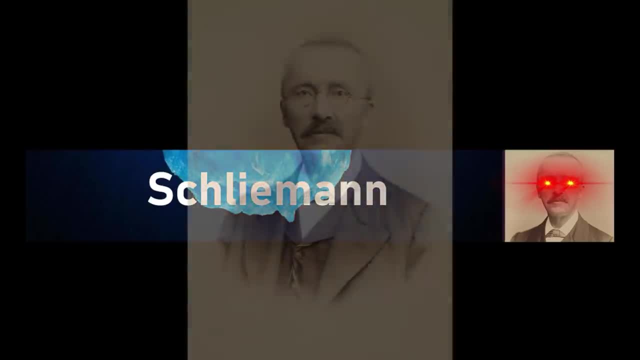 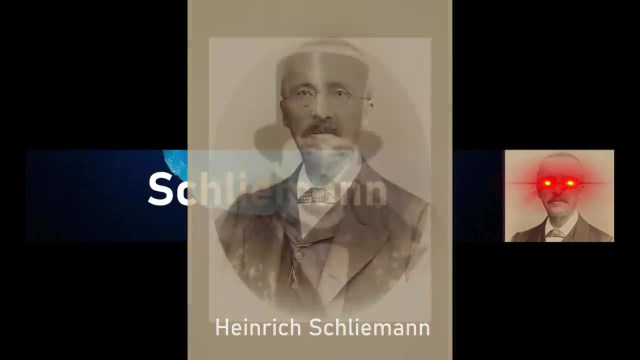 This level is devoted to the story of one of the founders of modern archaeology, the man us archaeologists loved to hate, Heinrich Schliemann. And oh boy, was this guy wild. Heinrich Schliemann was a German businessman in the mid to late 1800's who had a passion. 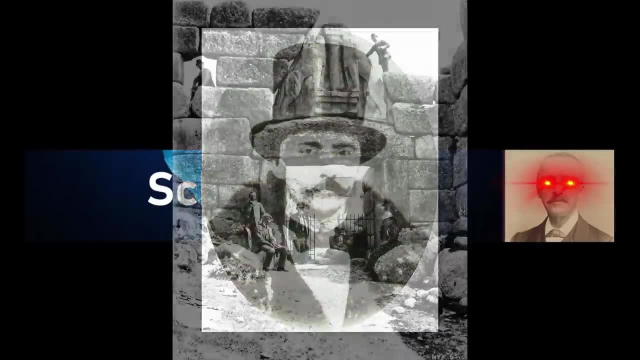 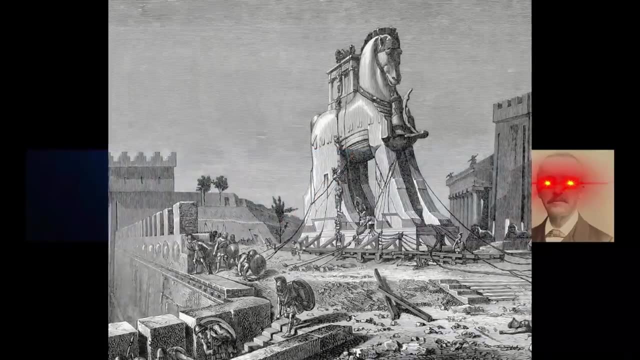 for the works of the ancient Greek poet, Homer, and used his extensive wealth to finance his hobby of digging up ancient sites across the Aegean. Schliemann's lifelong dream was to hunt down the legendary city of Troy mentioned in Homer's Iliad and the Odyssey. 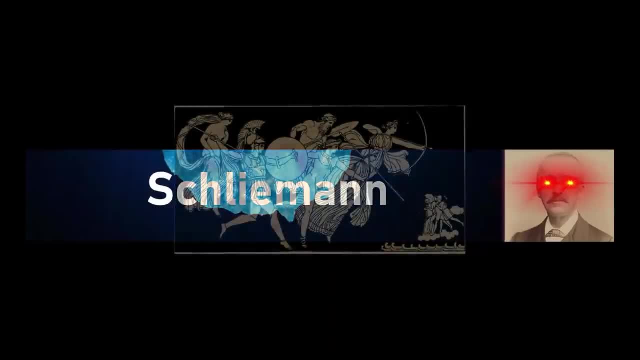 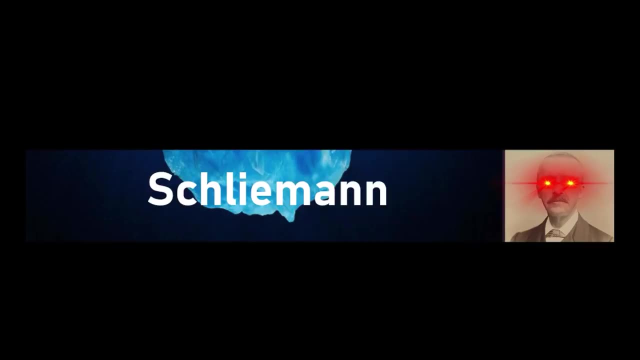 At the time this was seen as a bit of a fool's errand. Up until the late 19th century, Troy and the Trojan War was largely thought of as a fantasy or a myth with no historical basis. Schliemann disagreed and believed that the war was an actual historical event and the 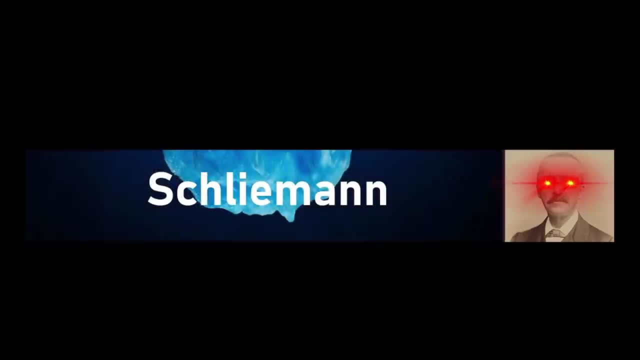 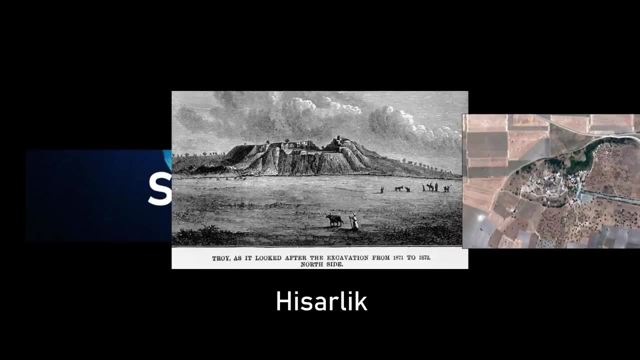 city was at one point a real location. After some sleuthing, he identified the site of Hiserlik in what is now Turkey as the historical Troy and began excavating it in the 1870s With the most delicate of archaeological methods: dynamite. 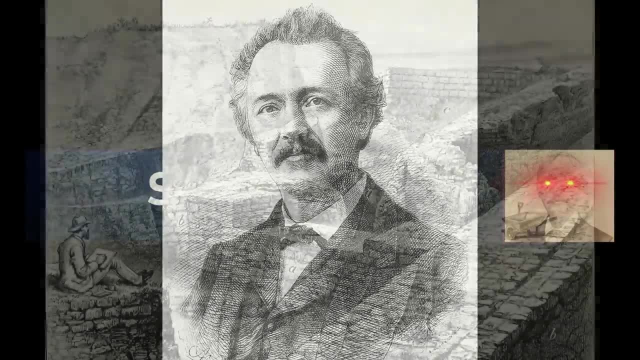 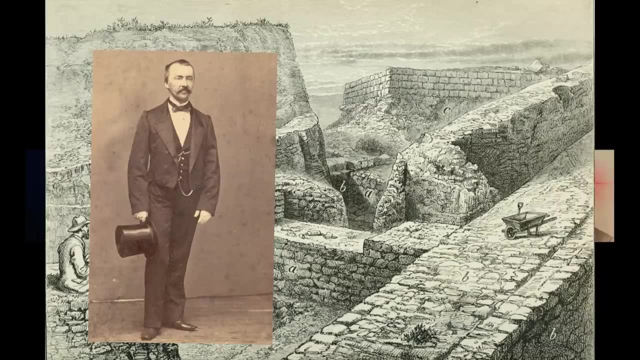 The crazy thing is that he was right. Hiserlik is seen by modern archaeologists as the historical Troy. Unfortunately for us, however, Schliemann was the one who found it first, and his explosive methods were devastating, destroying much of the important historical context of Hiserlik. 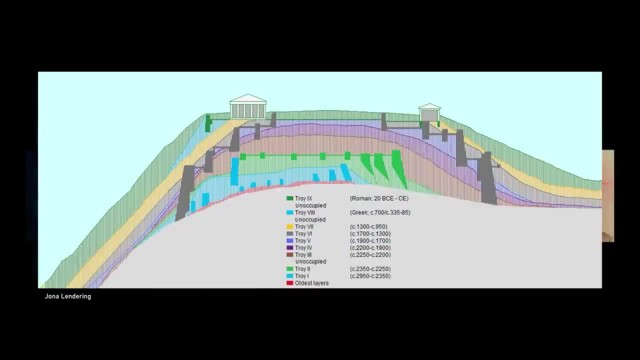 forever. For example, we now know that the soil level that Schliemann had found in the 1870s was the soil level that Schliemann had found in the 1870s. The soil level that Schliemann identified as the Trojan War was too old to be Homer's. 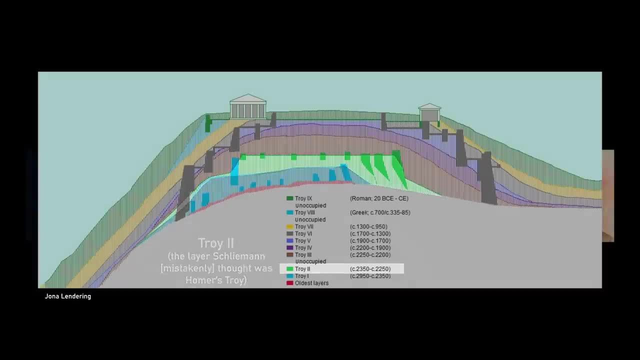 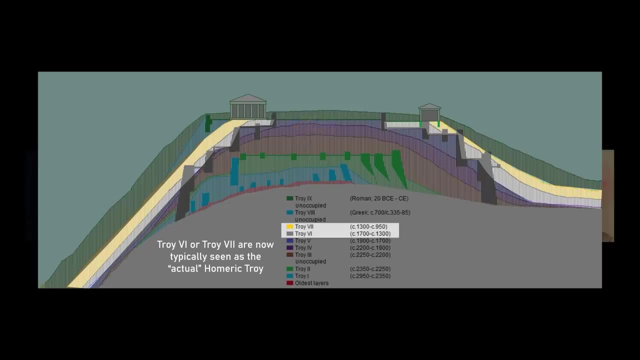 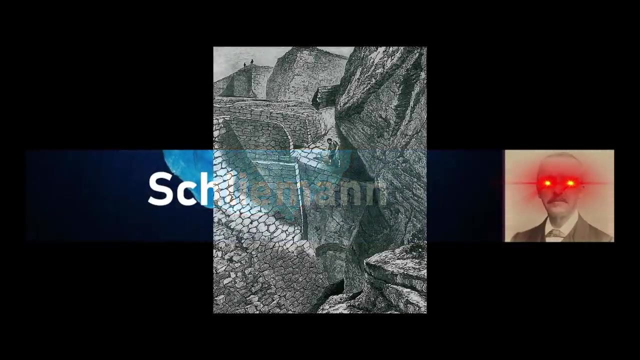 Troy, and in order for him to access this older level, Schliemann had to recklessly remove the younger layers above it, effectively obliterating all traces of the real Trojan War. in the process, Schliemann kept few, if any, records or maps of his excavations too so he took little. 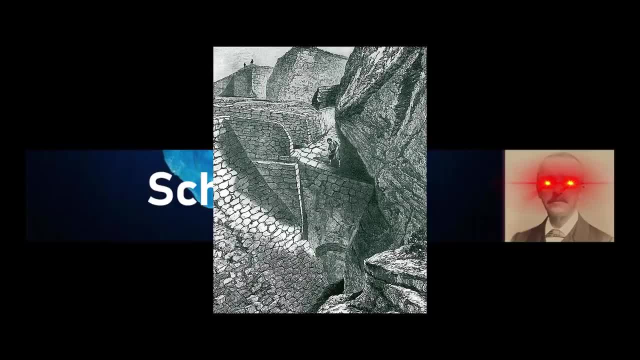 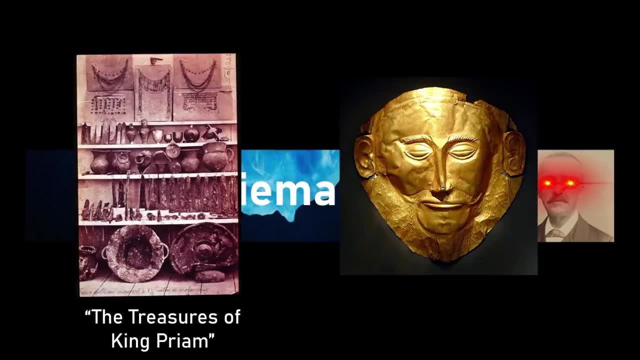 care to document the locations of objects or finds. He also had this tendency to claim any artifact he found must have belonged to someone who belonged to someone historically significant, calling things like the treasures of King Priam or the Mask of Agamemnon based onabsolutely nothing. 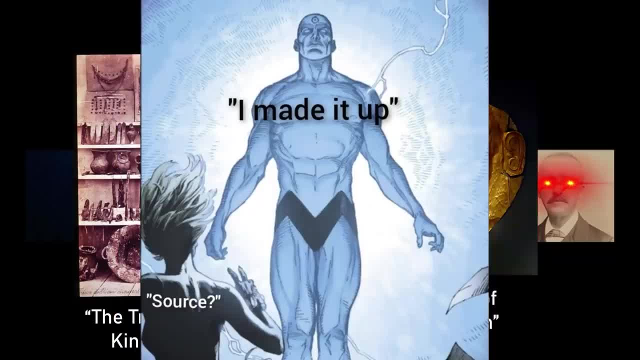 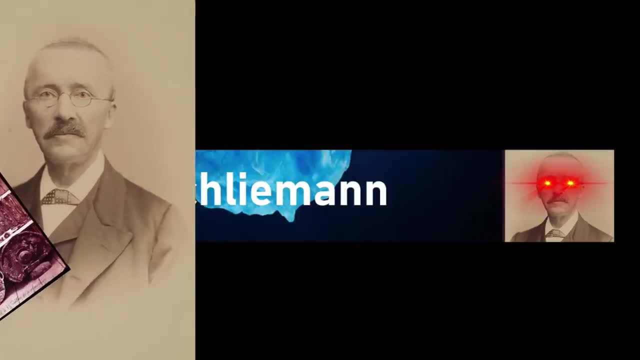 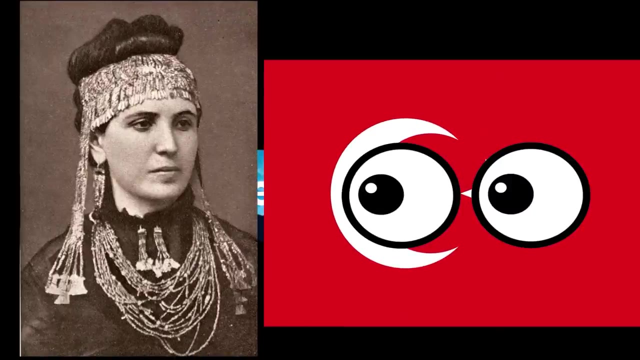 He literally just went. yeah, sure, that sounds right. Source: I made it all up. But wait, it gets worse. Schliemann smuggled several of the more valuable of Troy's treasures out of Anatolia, and the Ottoman Empire only knew about this because Schliemann let his wife Sophia wear the. 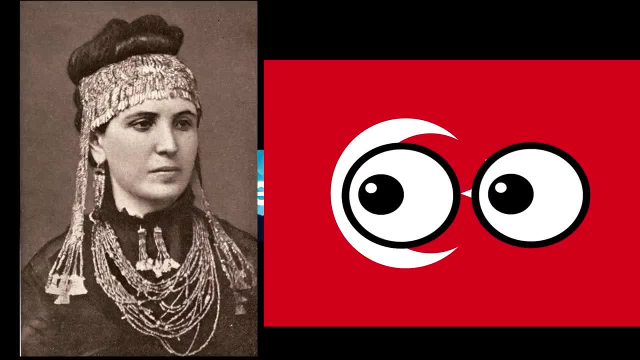 priceless 4,000-year-old jewels in public, And that's it. He didn't even get rich, I mean, you know. if you've been around the world ever since, you think that's something to see in your head, And you can imagine, though, that he was always literally traveling at like parties and stuff. 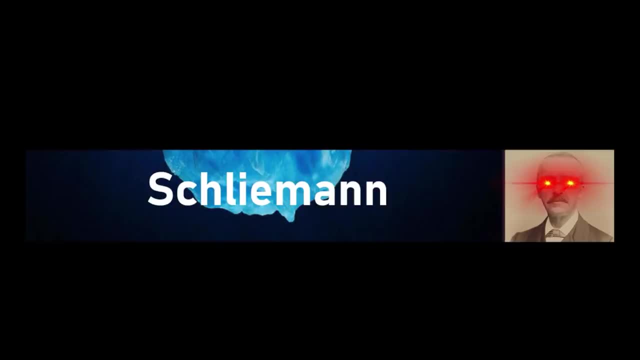 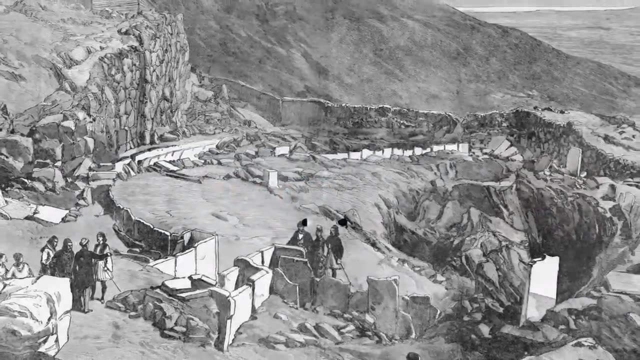 which is like what? Upon learning this, the Ottoman government understandably banned Schliemann from digging in their country and tried to sue him for the gold, But he just fled to another country and dug up the ancient city of Mycenae in Greece instead. 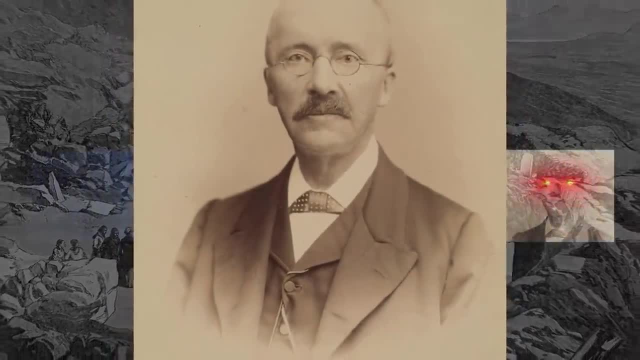 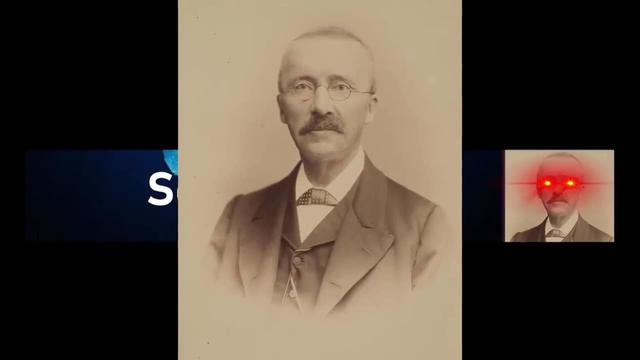 All agree Schliemann was pretty bad, Pretty, pretty bad, Even for the time when the field of archeology was still in its infancy. the amount of damage to science Schliemann did through his needlessly careless investigation of things like this. 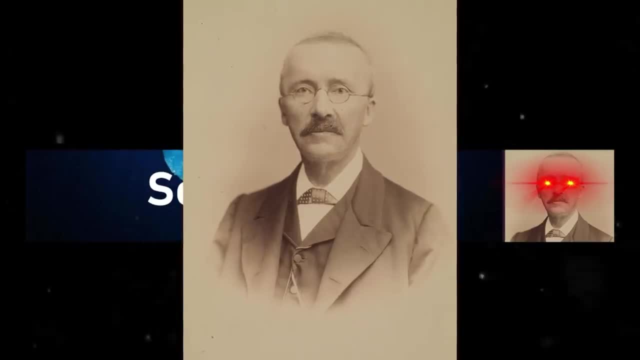 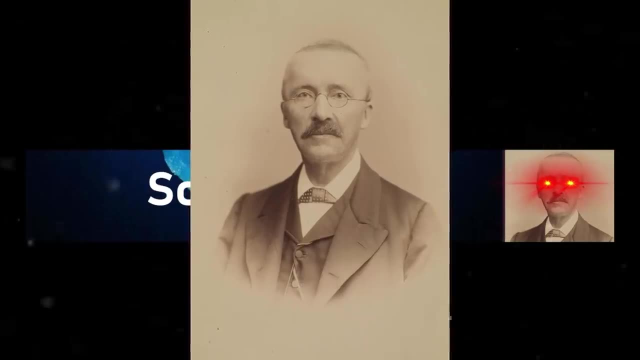 his needlessly careless methods is immeasurable, to say the least. We can never get the knowledge he destroyed back. Schliemann's story basically serves as the textbook example of how not to do archaeology. Oh, Schliemann, you rapscallion you. 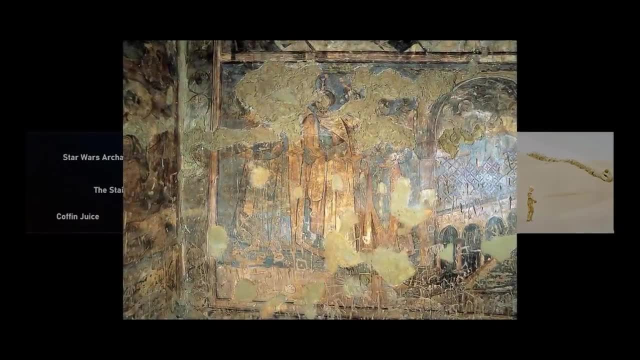 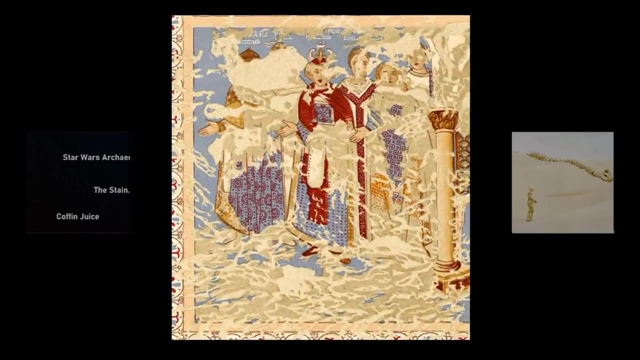 Kings of Earth refers to a rather obscure fresco at the Umayyad Caliphate site of Khuzra Amra. It is said to depict the six kings of the world known at the time. The fresco is very damaged. so it's hard to say who all of them would have been, But of the ones we know, there was the Visigothic king of Hispania, Roderick the Negus of the kingdom of Aksum, Najashi, an unnamed Byzantine. 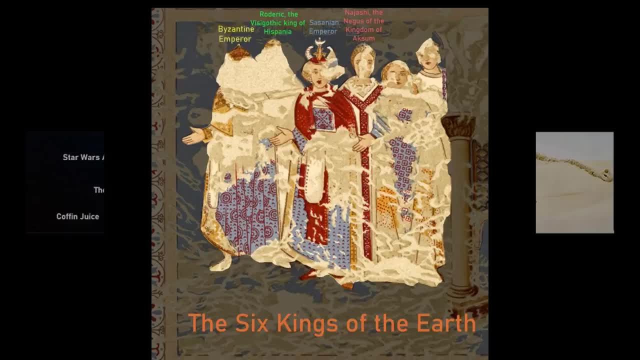 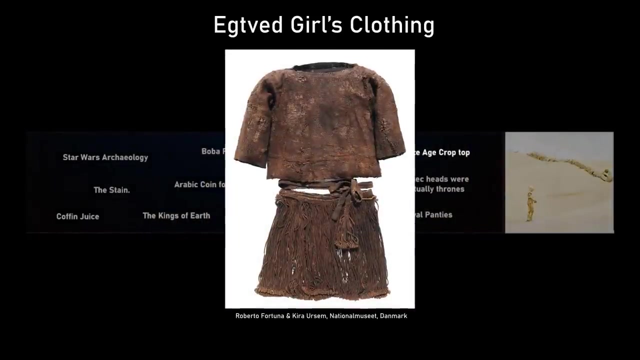 emperor and an unnamed Sasanian emperor. The identity of the last two kings is a subject of much debate, but they are speculated to be a Chinese emperor and a king of India, But this is still very much conjectured. Bronze Age Crop Top. This is a reference to the Ektvedt girl's well-preserved clothing. 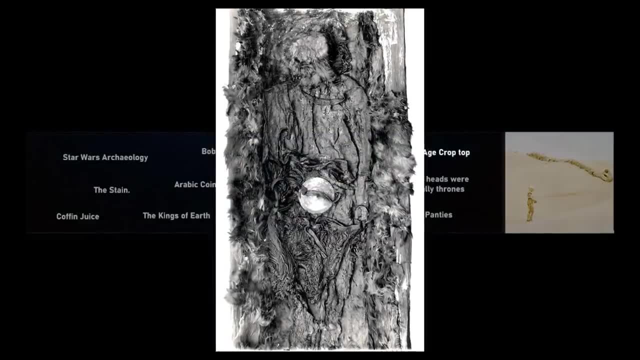 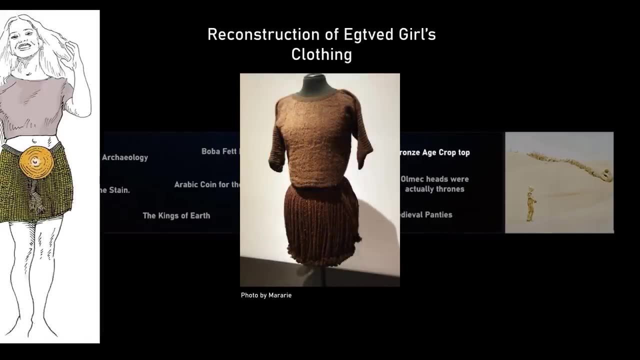 This Bronze Age girl was buried in a wooden coffin in what is now Denmark. Her surviving 3,400-year-old clothes consist of a loose bodice that left her waist bare and a short-string skirt with a large decorative disc. A bit of a Bronze Age waifu. 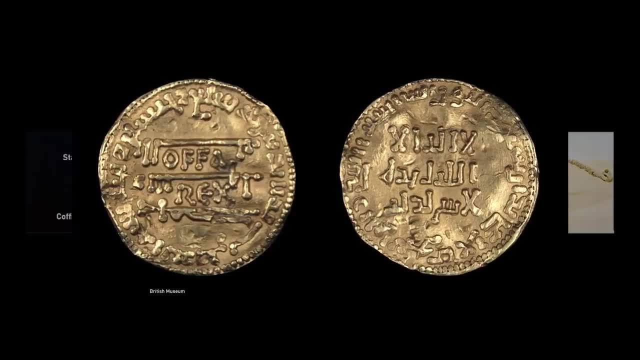 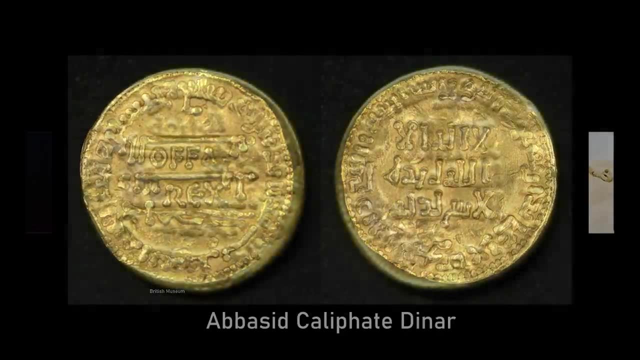 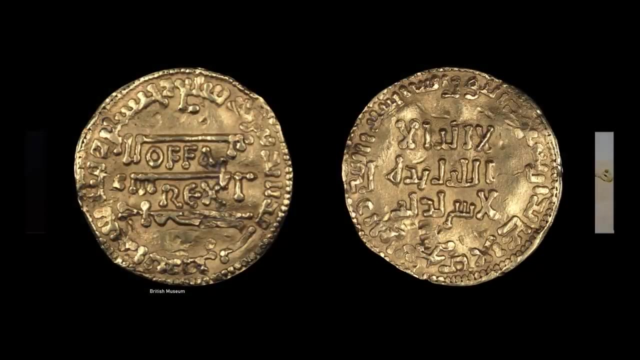 Arabic Coin for the Pope Refers to a rather unique gold coin minted by the English king Offa of Mercia In 774 AD. the coin appeared to have been a blatant copy of the coin struck by an Islamic caliph with the words Offa Rex awkwardly added in. The engraver who produced it tried their. 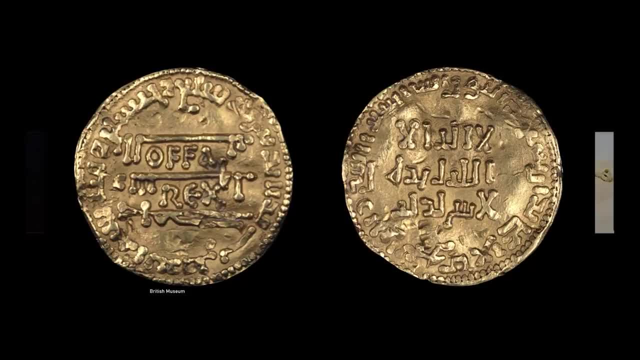 best to copy the original Arabic inscription, but obviously had no understanding of the language, so the text contains many grammatical errors and typos. Why this bizarre coin was made in the first place is unclear, but one theory posits that it was a gift to the Vatican. 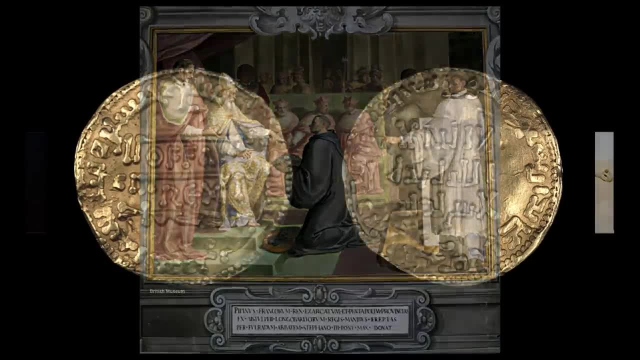 Pope. This is a bit funny, given that the original Vatican Pope was named after the Roman abbot, but now he was called the Holy Pope, Which is kind of funny when you realize that this Arabic letters on it read: there is no god but Allah alone. I'm guessing that probably wouldn't. 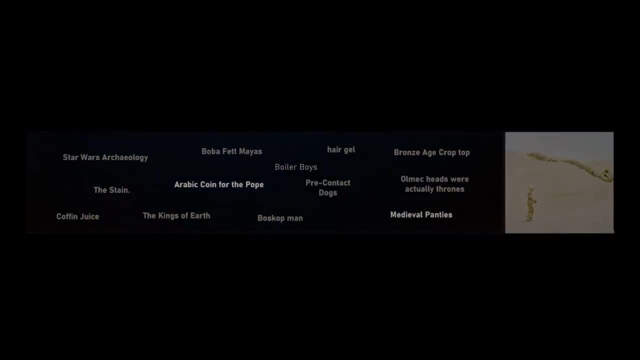 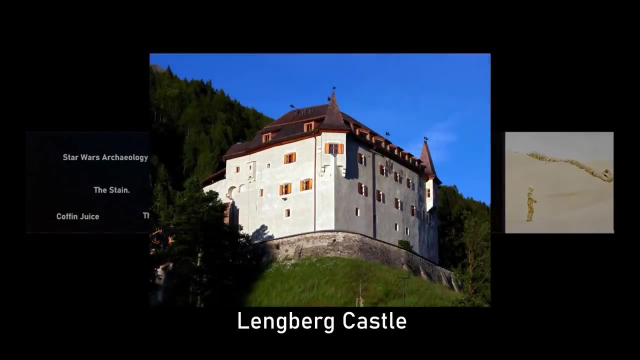 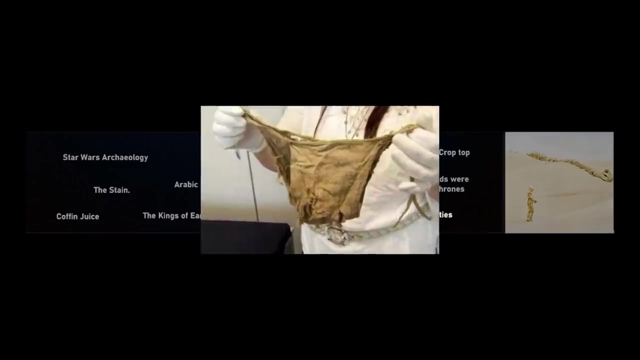 have gone over well with the Christian Pope Medieval Panties. In 2008,, archaeologists discovered a secret chamber in Langberg Castle, Austria. Inside was a hidden stash of clothes dating to around the 1400s. Among these garments were some of the best preserved medieval underwear. 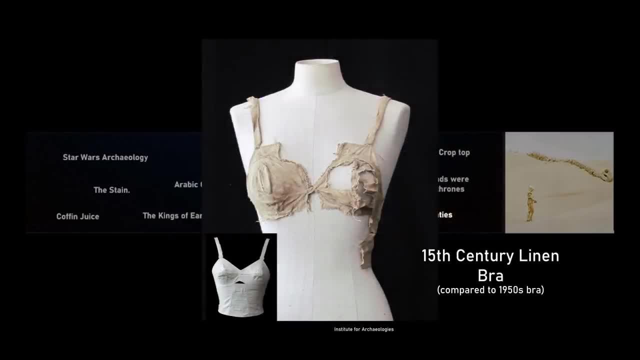 including four linen bras. This was a bit of a surprise, as it had been previously thought that female bras like these, with two separate supportive cups, wouldn't be invented until much later in the Victorian era. Discovery provided, I quote, a missing link in the history. 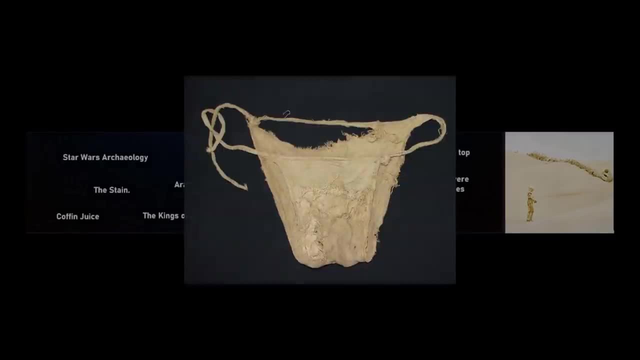 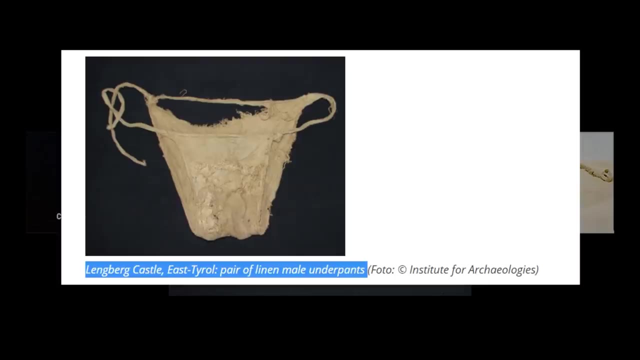 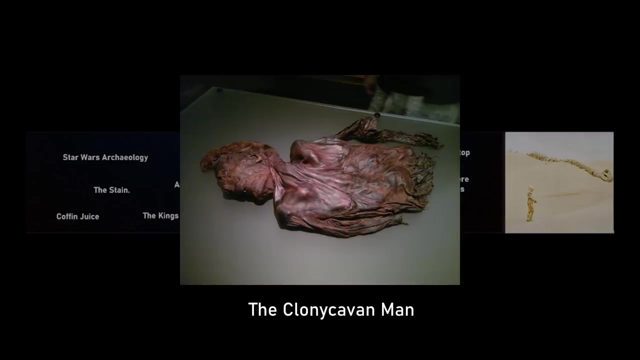 of women's underwear. Also, it is pretty funny that the linen panties found in the chamber probably belonged not to a woman but a dude. Hey, I get it, I'm more of a briefs guy myself. Hair Gel. The Cloney-Caven Man is a well-preserved Iron Age bog body found in Ireland. Analysis of 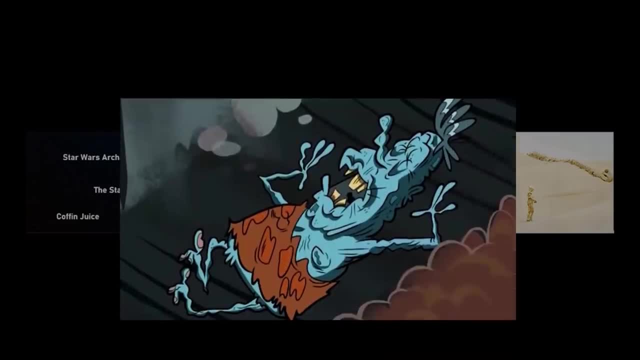 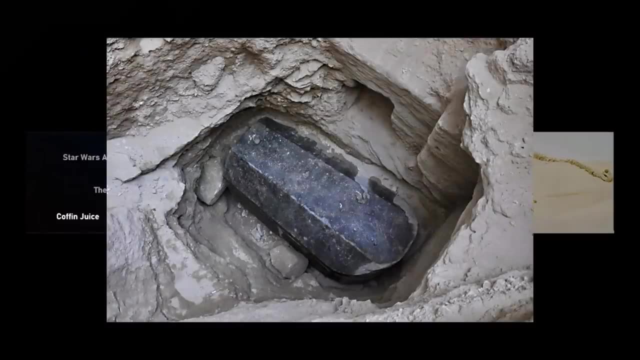 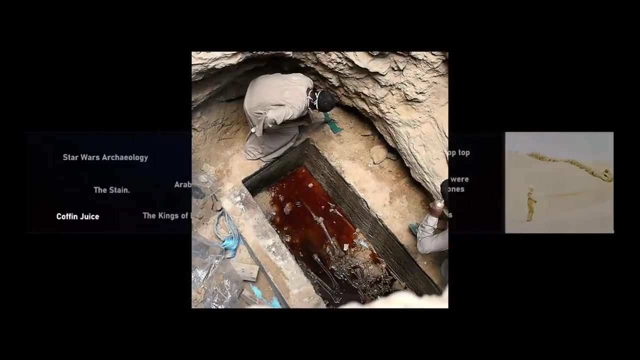 his body showed that the man liked to style his hair using tree resin as a primitive type of hair gel: Coffin Juice. When the so-called Black Sarcophagus in Alexandria, Egypt, was opened in 2018, news outlets reported that it was filled with bones floating in a soup of red, dark sludge. 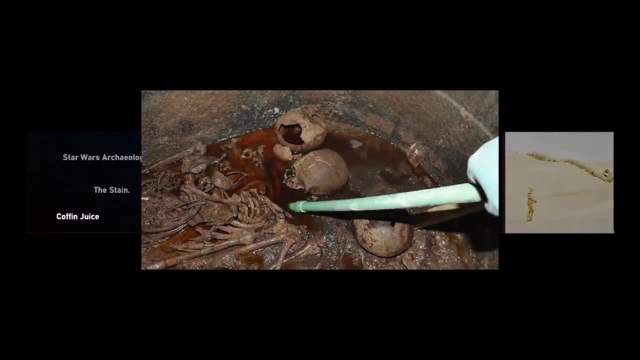 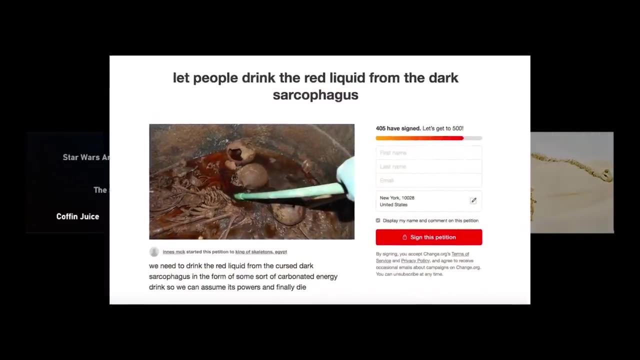 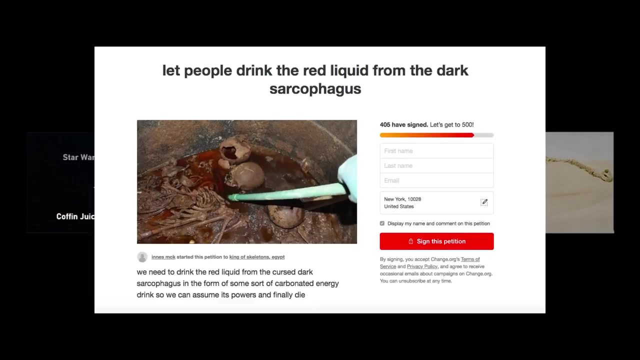 The story and its accompanying photos quickly captured the attention of the public In maybe not the best of ways. many online petitions circulated around, demanding that the archaeologists allow people to drink the Coffin Juice. The uh juice in the coffin was actually sewage from Alexandria's underground drains, so it is in my humble opinion that 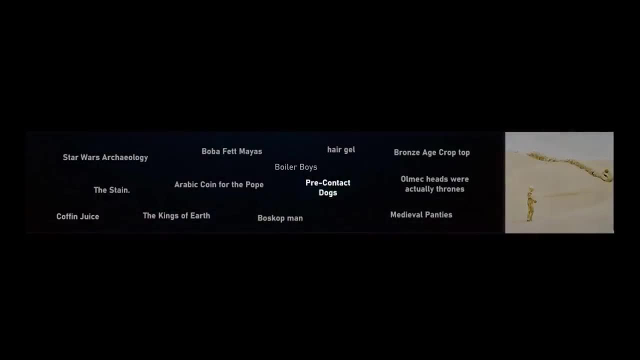 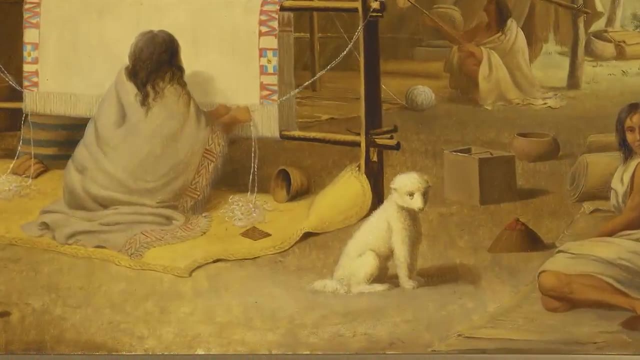 you probably shouldn't drink it. Pre-Contact Dogs. Prior to European contact, the indigenous peoples of North and South America had their own unique dog breeds found nowhere else in the world. These dogs were known for their unique appearance and their personality. However, aside from Chihuahuas and a handful of other breeds, all these dogs became 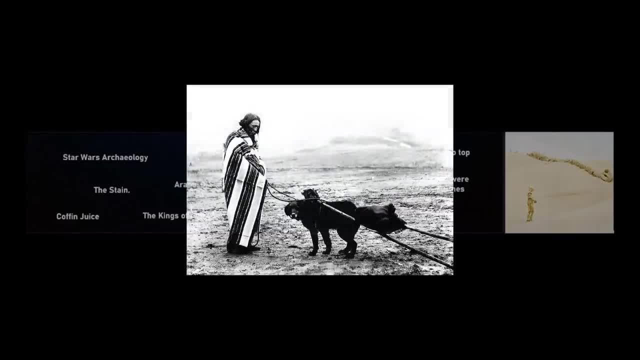 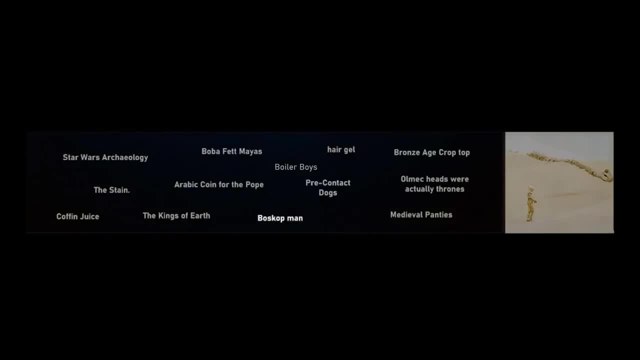 extinct after European contact, likely due to disease and competition with European dogs. I also did an entire video on these guys, so check that out. Boskop Man. In 1913, the fossil remains of a prehistoric human were discovered in South Africa. 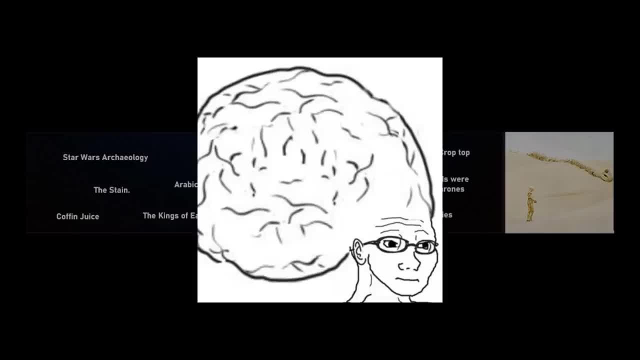 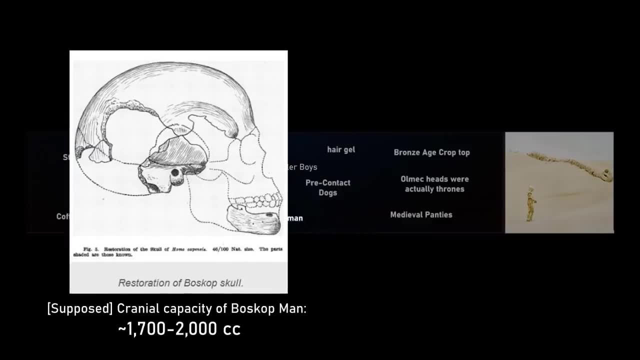 and according to anthropologists at the time, it apparently had a massive brain. The Boskop Man, as it was later known, had a calculated cranial capacity between 1,700 and 2,000 cc. By comparison, the average human today has a cranial capacity around 1,400. 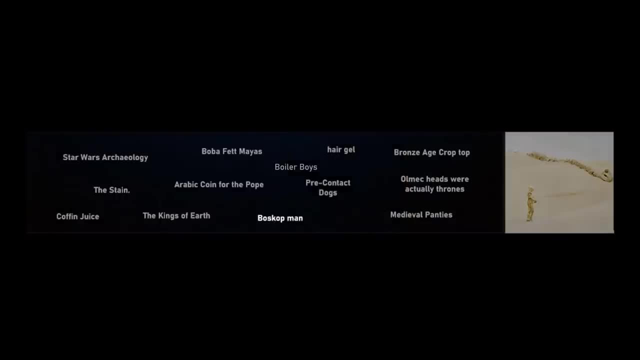 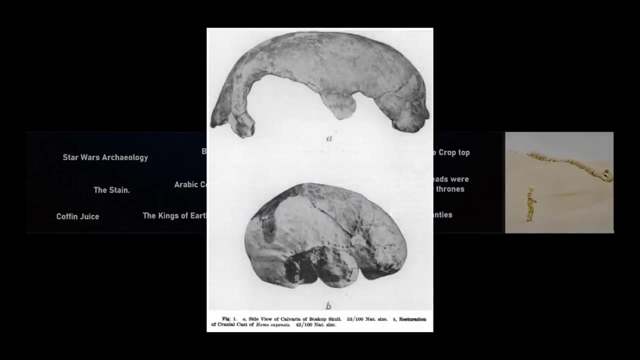 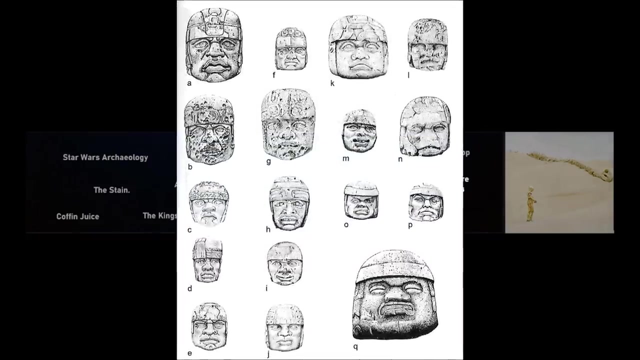 to 1,500 cc. Now, reexamining the story, it is hard to ascertain the truth of this claim. The fossil was highly fragmentary, so I would chalk this unusual cranial capacity to researcher error. Olmec Heads Were Actually Thrones. It appears that at least some of the famous 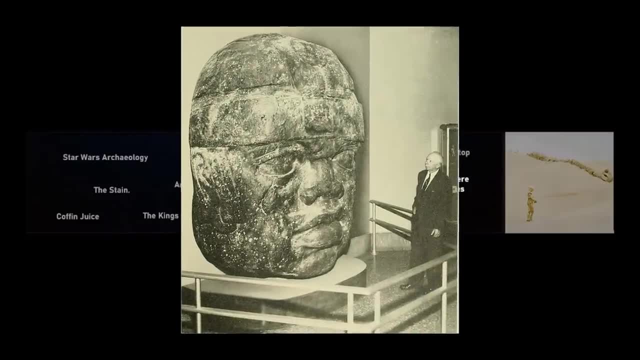 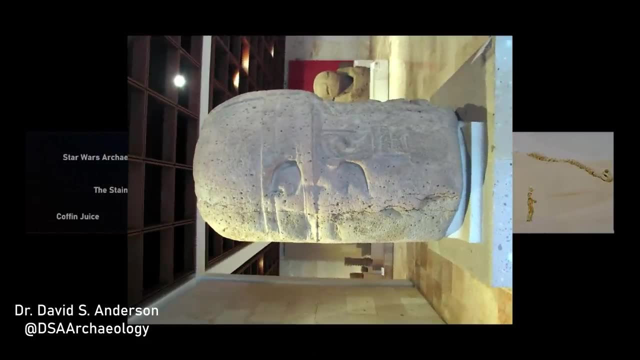 Olmec Heads of Central America were not, at least originally, to be heads. At least two of the colossal craniums show the unmistakable signs of being re-carved. They originally seemed to have been stone chairs or thrones prior to being re-sculpted. 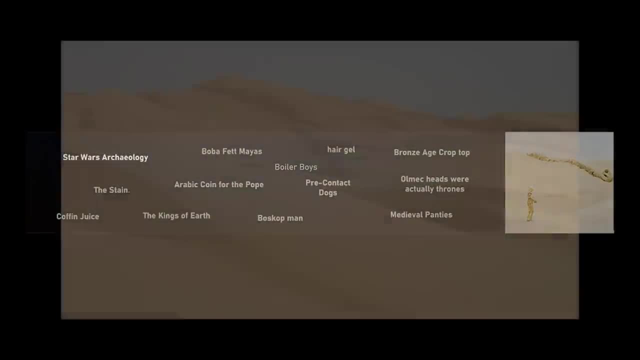 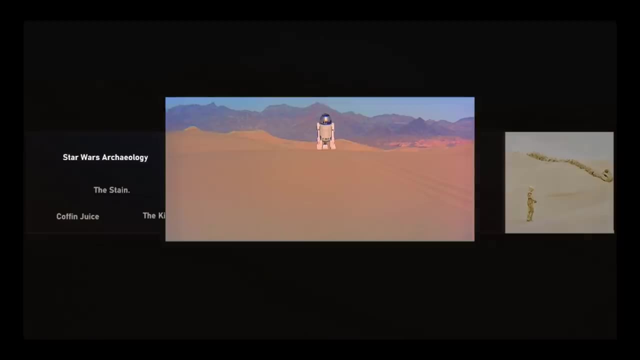 Star Wars Archaeology. For decades, people have been searching in some of the most remote parts of the globe, not for the remains of a lost civilization, but for artifacts from a galaxy far, far away. You see, after filming the iconic Star Wars film franchise, the behind-the-scenes 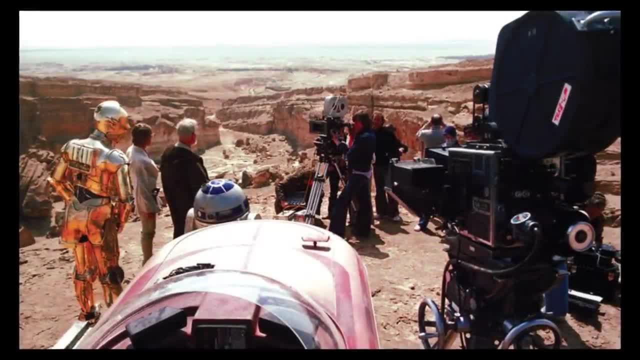 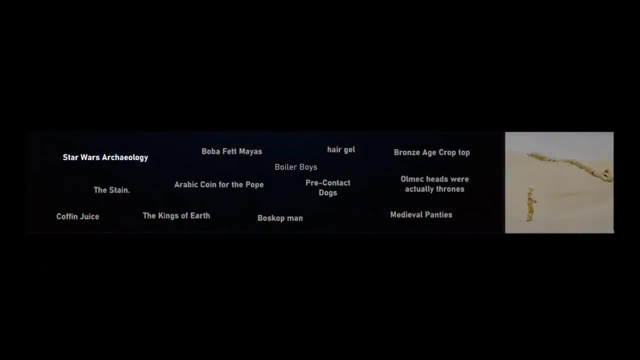 crew for several of the movies apparently just left many of the original props at their filming locations, where they sat abandoned for years. Enthusiastic movie fans have tracked down several of these artifacts, from the charred ruins of Uncle Owen in Aunt Beru's house to the fiberglass. 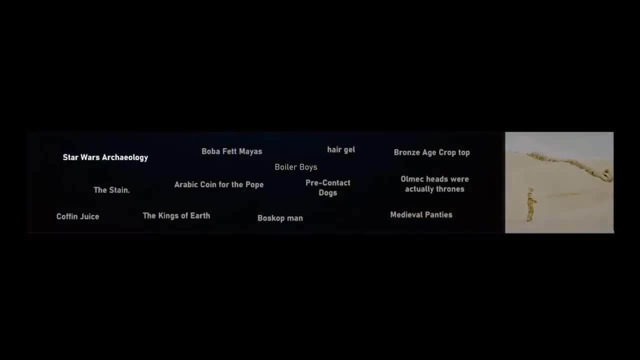 skeleton of the Krayt Dragon in the deserts of Tunisia, to the fragmentary wreckage of Jabba's sail barge in Buttercup Valley, Arizona. Unfortunately, many of these unique pieces of film history have either been destroyed by the elements. 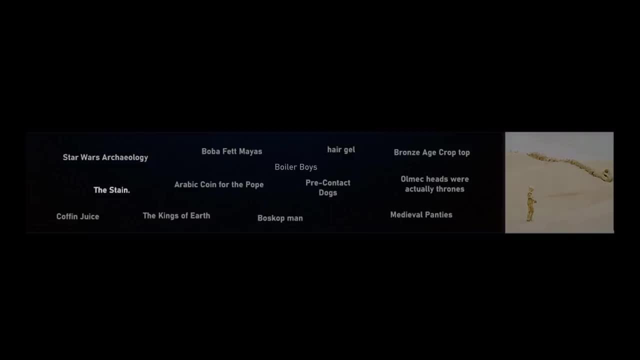 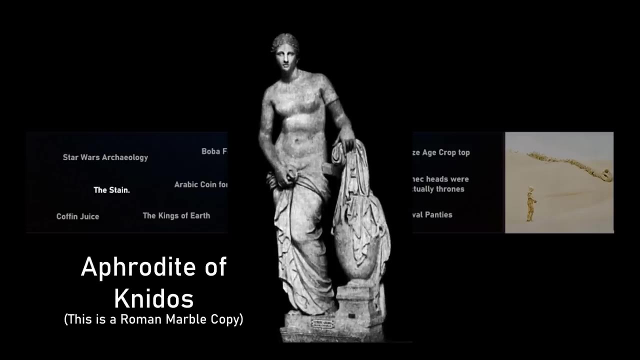 scavenged by locals or resold to private collectors. The Stain: There was once an ancient Greek statue called the Aphrodite of Kindos. It was supposedly so attractive and lifelike that at night young men would sneak into the. 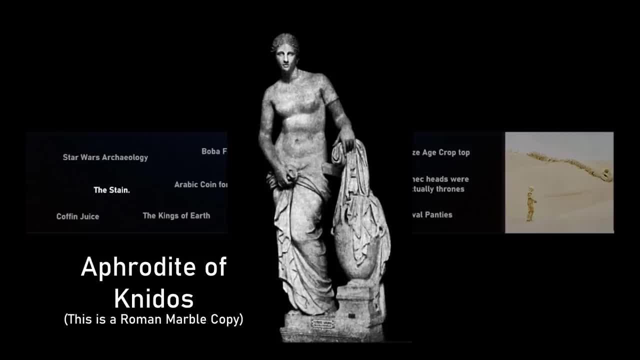 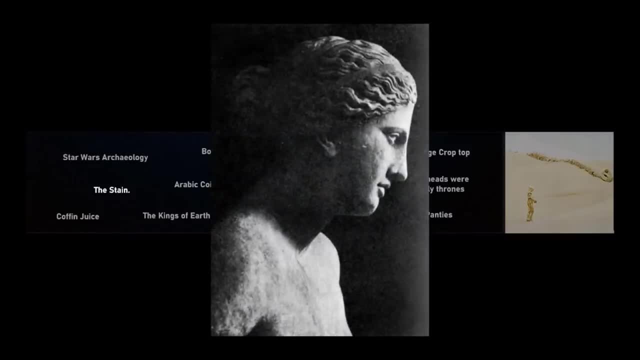 temple that housed it and, uh, let's just say, used it inappropriately. According to legend, this happened so often that, over time, a dark stain became visible on the statue. Now we can't verify the truth of this claim because, although we have numerous Roman copies, 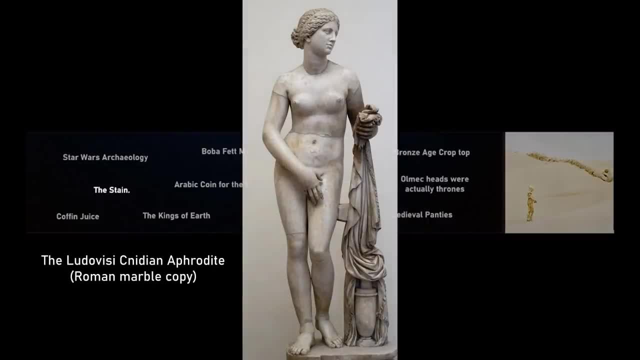 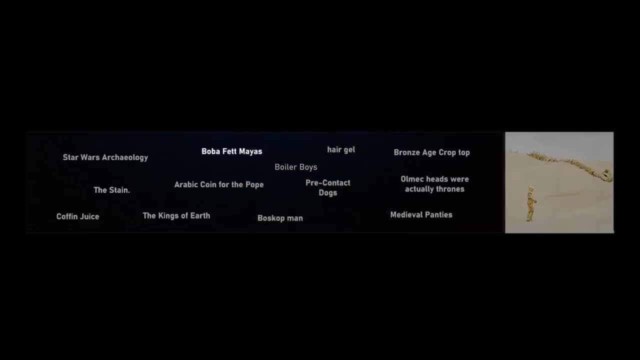 the original statue had a dark stain on it. The original statue had a dark stain on it and most likely it never will. But who knows, the statue and its possibly legendary stain might still be out there. Boba Fett, Mayas: The helmets of Mayan ritual boxers look a lot like 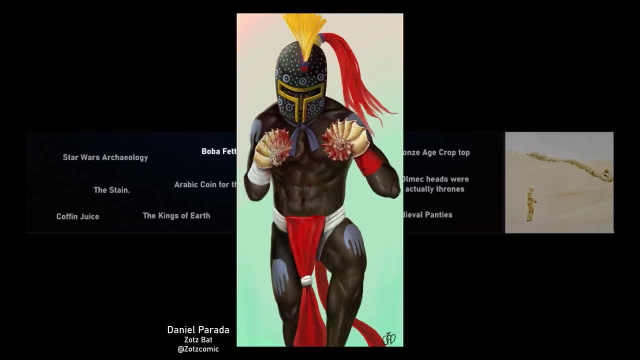 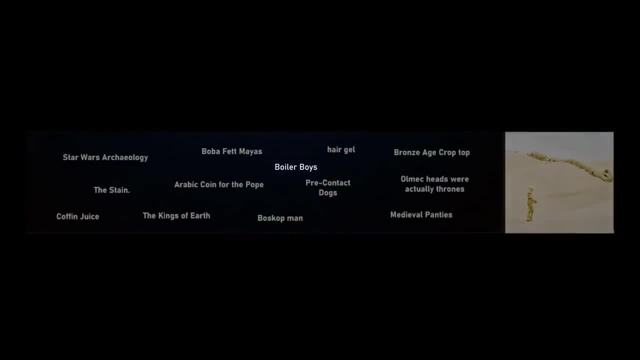 Mandalorian helmets from Star Wars. These boxers use giant spiky conch cells as boxing gloves in their very bloody sport, The Boiler Boys. There is an obscure and ancient grave in what is now Germany that commemorates two brothers named Saluda and Rikki. They are the only ones who have ever been found. The Boiler Boys are the only ones. 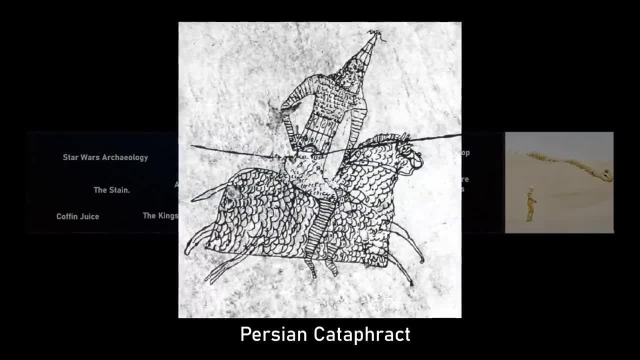 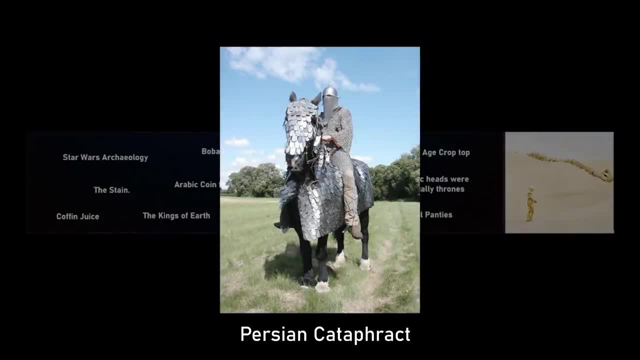 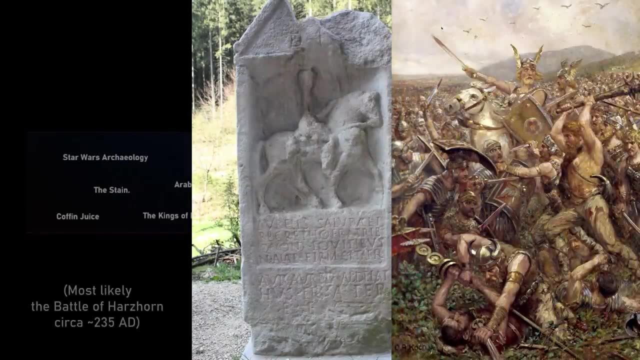 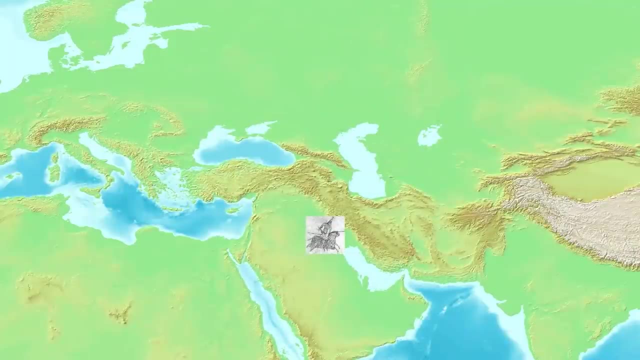 demeaningly called Boiler Boys because they tended to boil in the sun. under all that metal plate, These particular Boiler Boys apparently fought on the Roman side against barbarians in Germany circa 235 AD. The two brothers appear to have originally come from all the way in Mesopotamia. 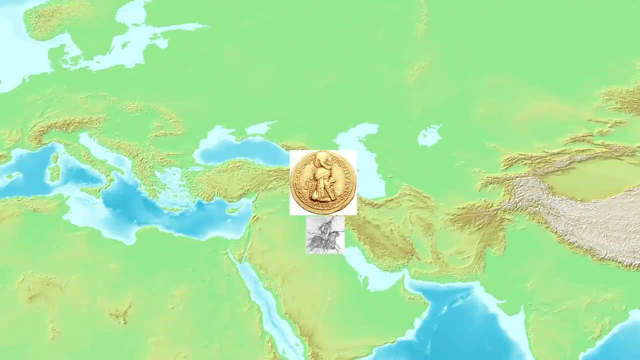 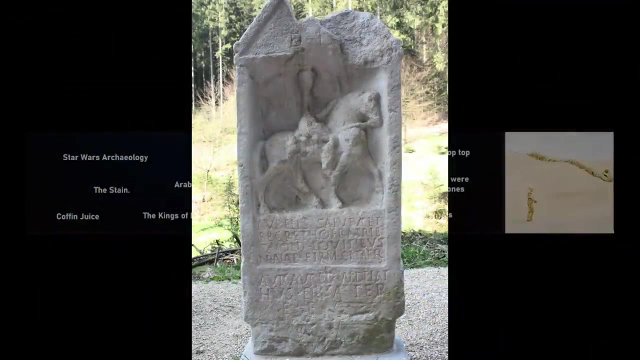 and served under the Sasanian king Adashir. They were likely mercenaries who sold their services to whoever needed strong fighters. Under Adashir, they might have traveled as far as the Indus before serving under Rome in the defense of its borders on the Rhine. This simple grave, in truth. 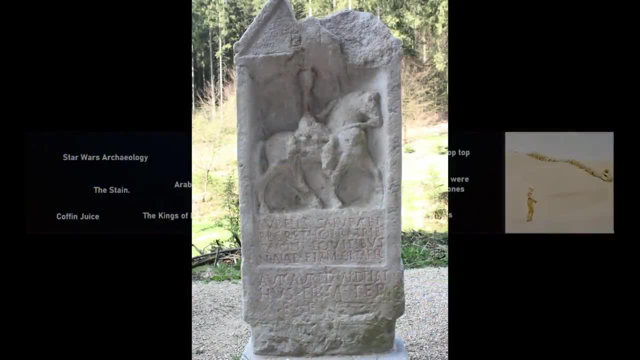 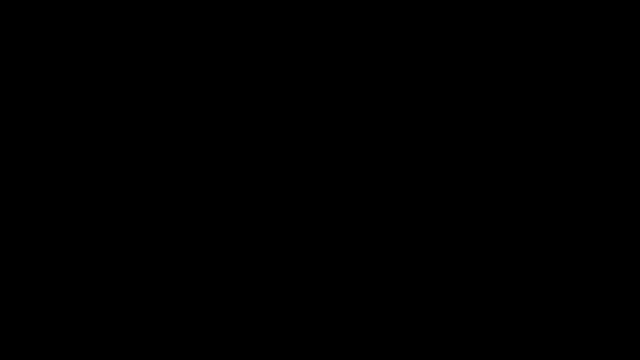 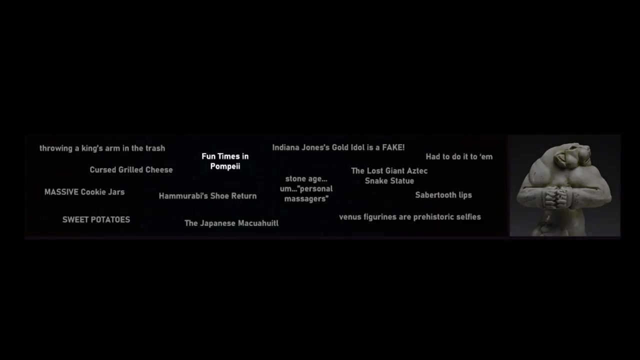 tells the story of two brothers who traveled the whole width of the known world together and fought in dozens of brutal and bloody battles, only to die in a swamp. so far from home and fighting for an empire. they probably didn't particularly care for Fun Times in Pompeii. 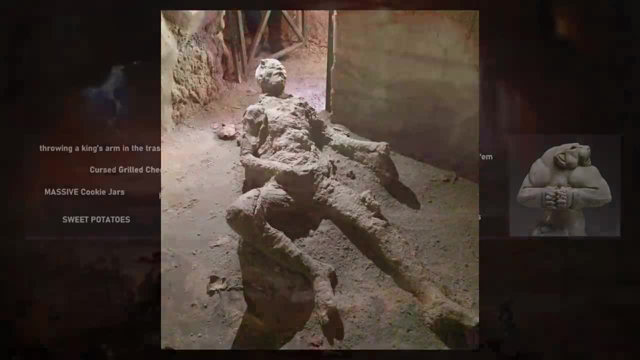 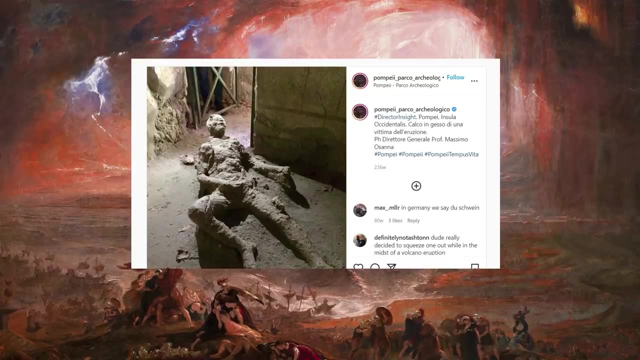 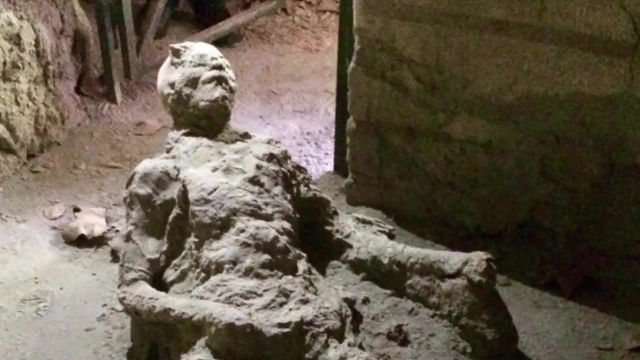 This refers to an image of a cast belonging to a man killed in the eruption of Mount Vesuvius in 79 AD, originally uploaded on Pompeii's Instagram. This image started to circulate online, with people claiming that the man was, uh, having a fun time. 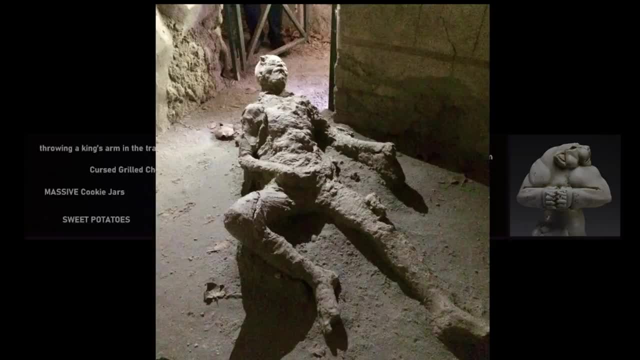 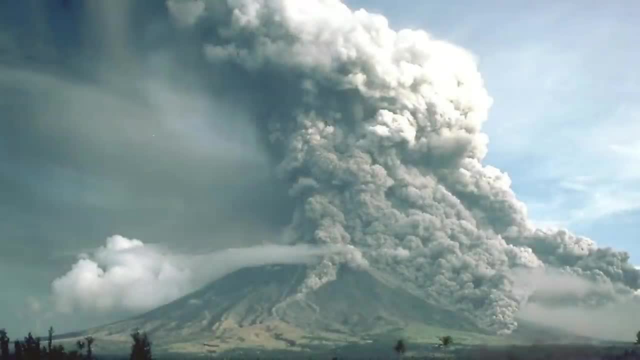 the moment he died. As it turns out, no, he's not giving it one last stroke before the end. The man probably just ended up in this position because his arms and legs flexed after death due to the intense heat of the volcano's pyroclastic flow. Sweet potatoes. 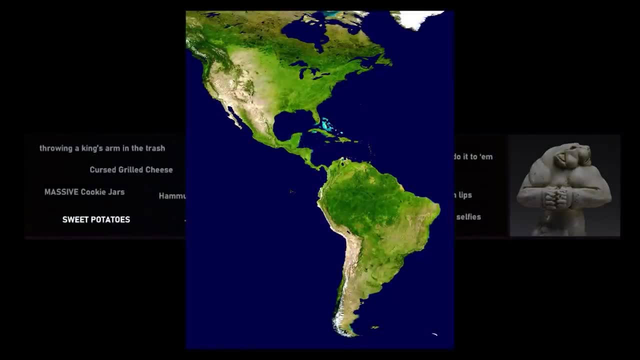 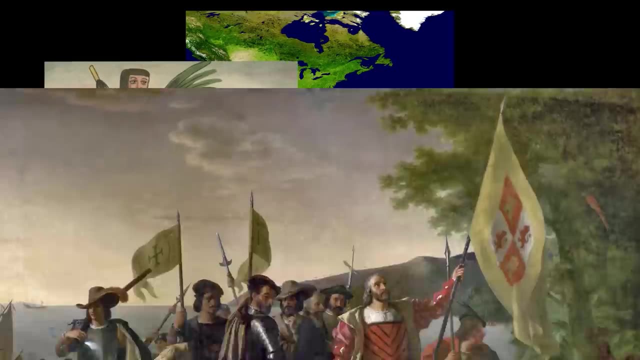 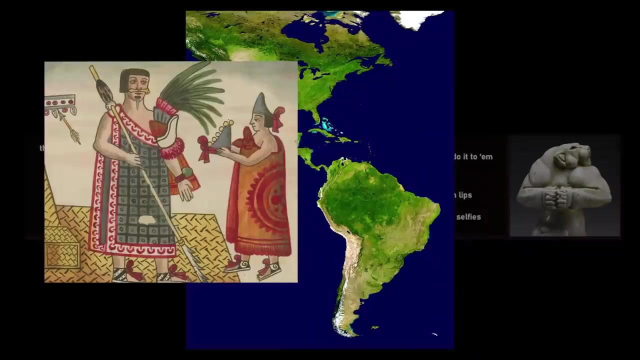 The common narrative we are taught in school is that North and South America and their native inhabitants were isolated from the rest of the world for tens of thousands of years, and it wasn't until Christopher Columbus crossed the Atlantic Ocean in 1492 that this isolation was broken. However, something is overturning this view. 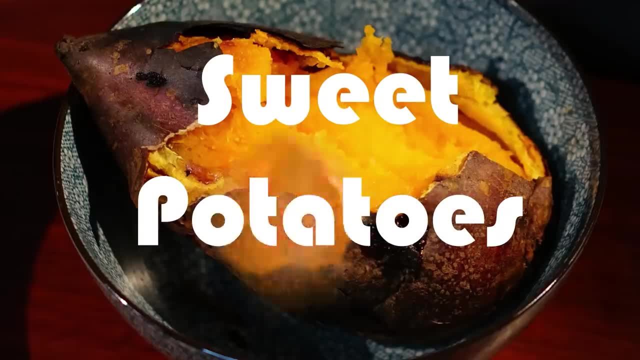 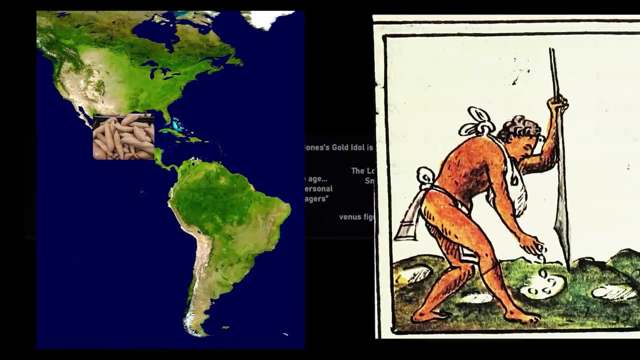 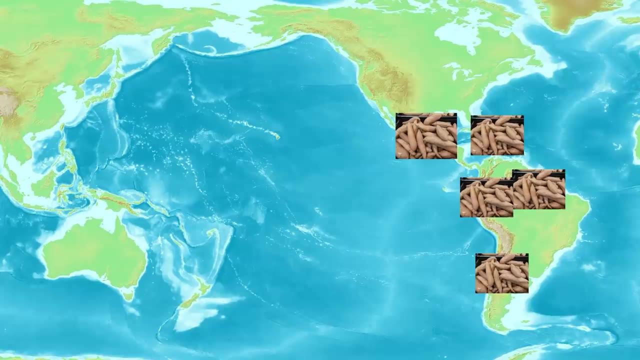 Something you wouldn't expect: Sweet potatoes- Potatoes- Sweet potatoes are a crop native to the Americas and were cultivated by Native Americans for many thousands of years. Interestingly though, archaeological evidence has shown that sweet potatoes were being cultivated in some of the very distant Pacific Islands since the 1000s AD. 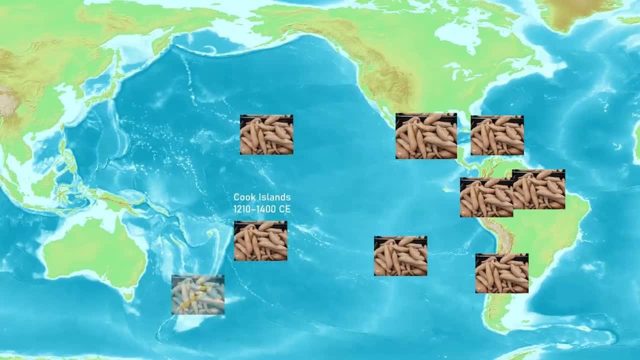 Polynesians on the Cook Islands, Easter Island, Hawaii and even New Zealand were growing sweet potatoes centuries before Christopher Columbus or any other European knew about the Americas. How these sweet potatoes made it all the way from Central or South America to these islands in the Pacific Ocean is a bit of a mystery. These potatoes are some of the strongest. 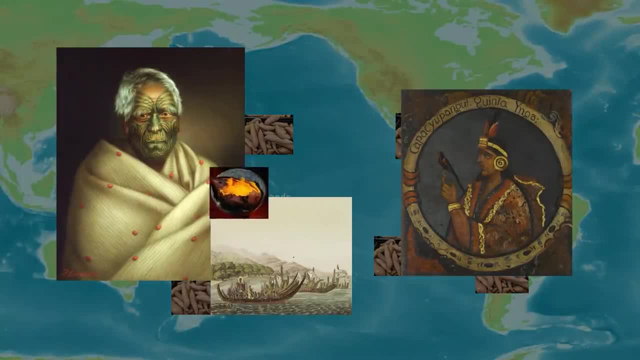 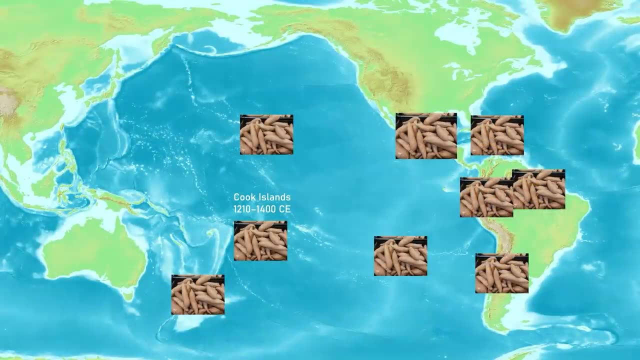 pieces of evidence that there might have been actual interactions in trade between Polynesians and South Americans long before European contact. On top of this, the word for sweet potato in Polynesian languages and South American languages are suspiciously similar, suggesting a shared 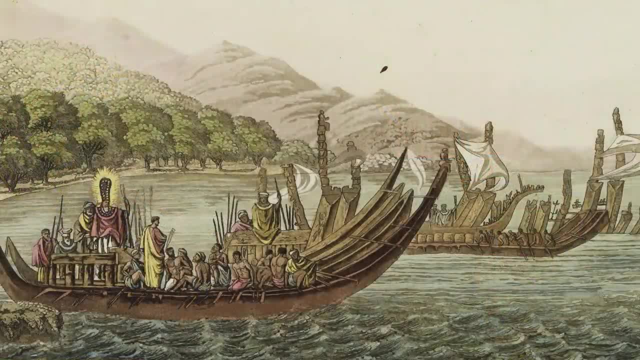 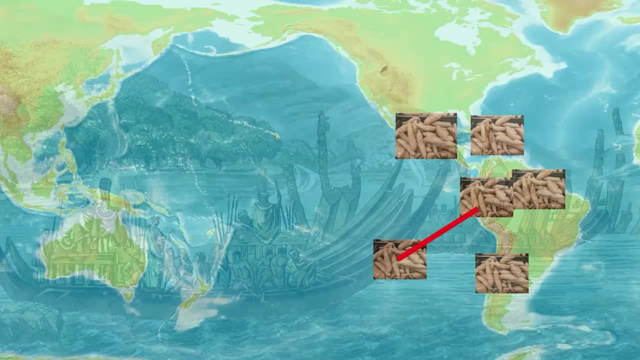 origin. Perhaps some canoes from the Polynesian language or Polynesian canoes from the South Polynesian islands, like Easter Island, traveled to South America. or perhaps the dispersal of this crop occurred naturally and the language thing is a weird coincidence. 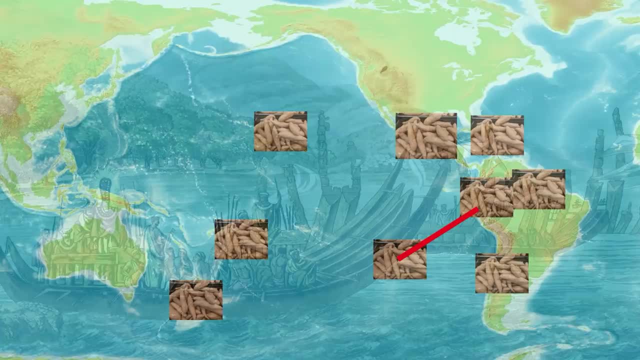 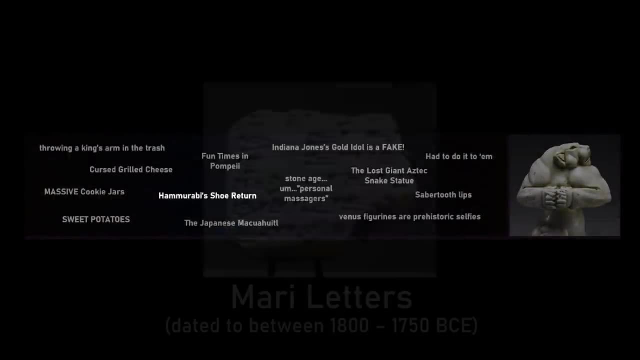 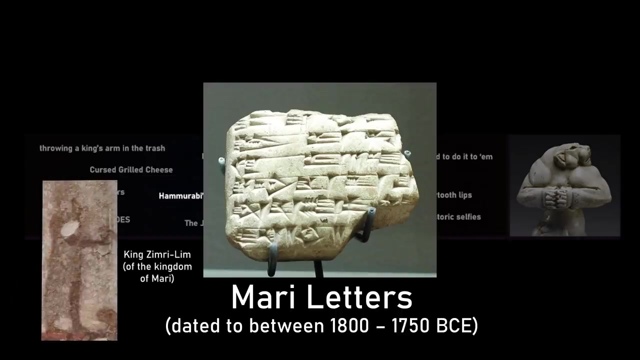 The point is we don't know exactly, and the whole Trans-Pacific sweet potato debate remains as this kind of unresolved mystery. Hammurabi's Shoe Return. This refers to one of the Mari letters, a series of clay tablets in Syria documenting written conversations sent and received by the King Zimri-Lim. 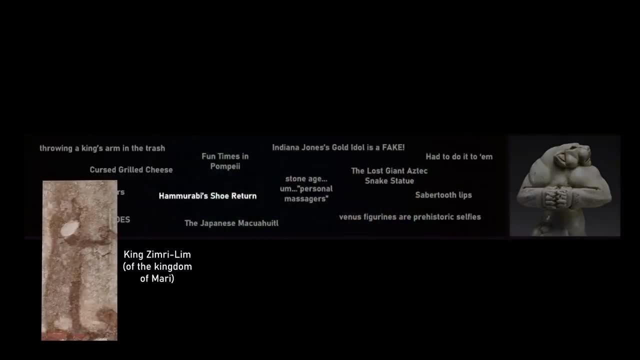 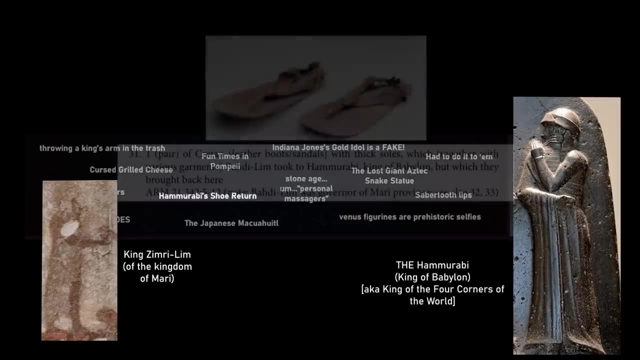 A rather curious letter records an interaction between King Zimri-Lim and the King of Babylon, Hammurabi. Yes, that, Hammurabi. In the letter it states that Hammurabi received a pair of Cretan leather boots or sandals. 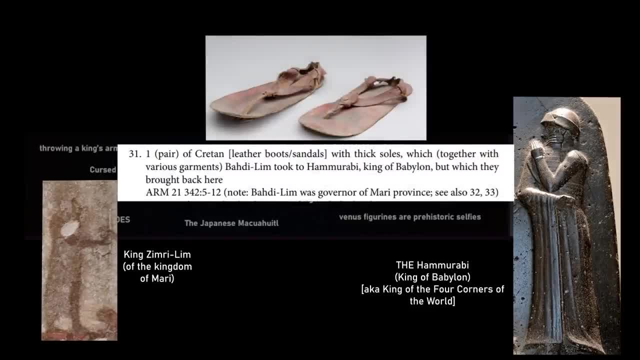 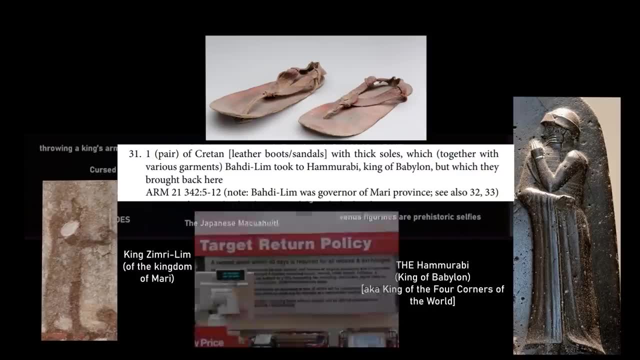 as a gift from Zimri-Lim, but Hammurabi returned them. These boots would have been a rather fancy and expensive gift, especially to transport so far. so it begs the question: why did Hammurabi return them? Were they too small or too big for his feet? 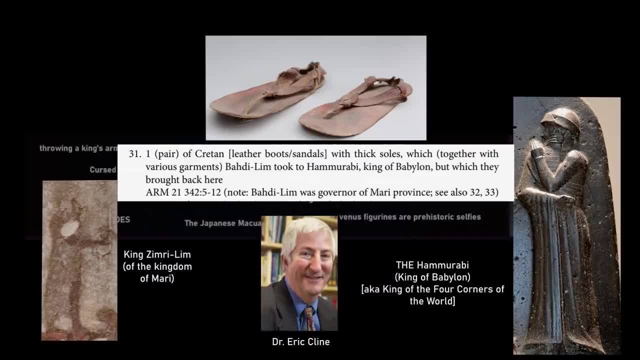 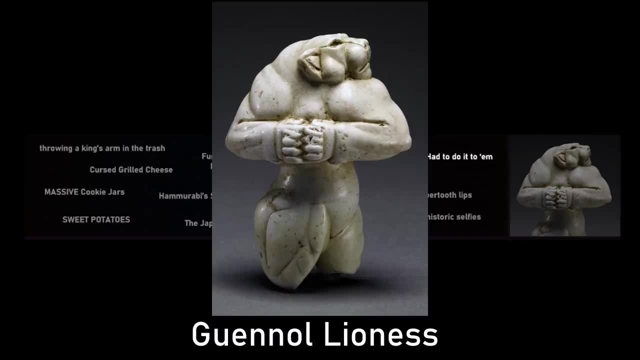 As historian Eric Klein says, Had to do it to him, Refers to the Gwinol Lioness, a supposedly 5,000-year-old Mesopotamian statue allegedly found near Baghdad, Iraq. It is better known as the most expensive antiquity to be sold in an auction. In 2007,. it was sold for $57.2 million. Why, I have no idea. don't ask me. Somebody must really like their 5,000-year-old jacked furries Throwing a king's arm in the trash. 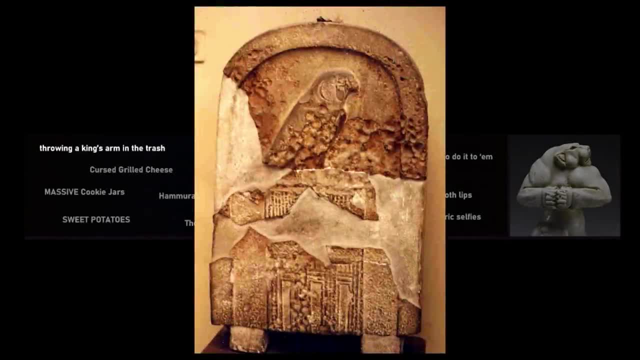 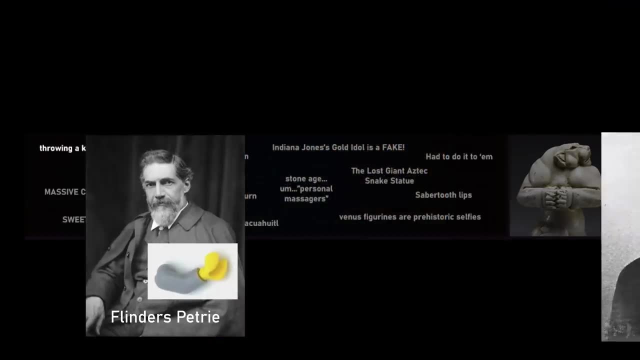 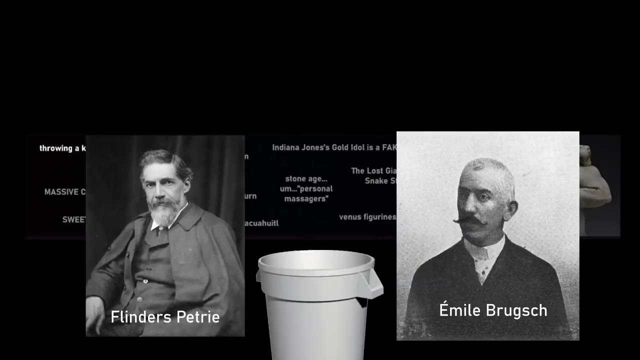 Possibly the oldest royal remains ever found was a skeletonized arm found in the tomb of King Jur by Egyptologist Flinders Petre. Petre gave the arm to fellow Egyptologist Emile Bruch, who supposedly promptly threw it away, thinking it was too drab for the museum to feature. 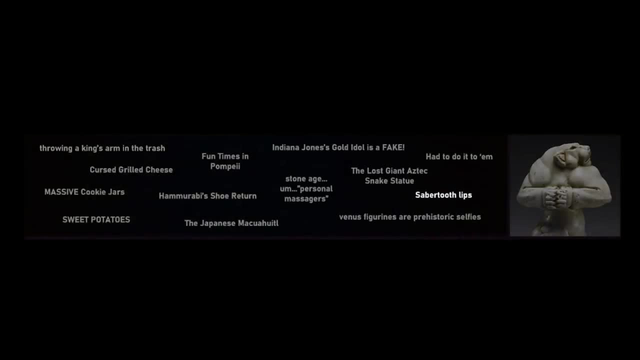 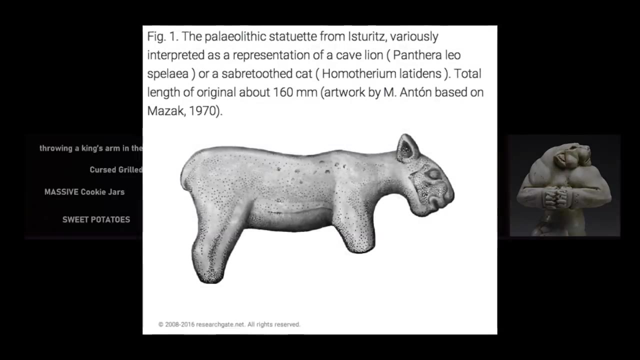 Welp Sabretooth Lips. Okay, this refers to a Paleolithic statuette from the prehistoric French site of Itzuetsu. The statuette has been lost since at least the early 20th century, So all we have of it are drawings based on the original. 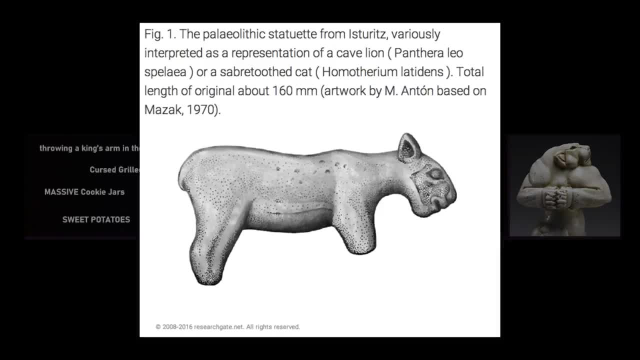 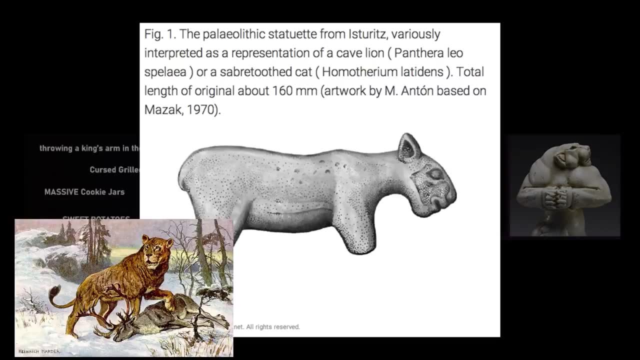 It depicts some kind of big cat, but what type of big cat is a point of contention. Most think it is a representation of a cave lion, but a small minority have posited that it might represent a sabretooth cat, specifically a homotherium, which is definitely the more 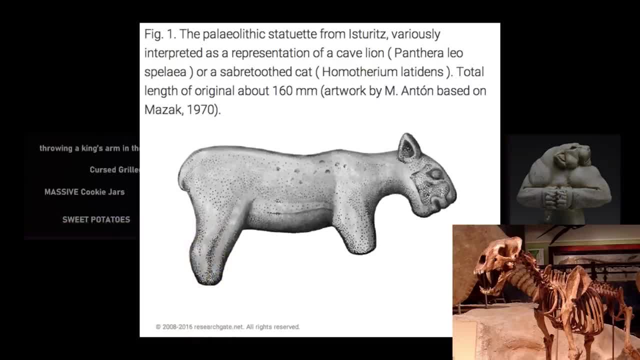 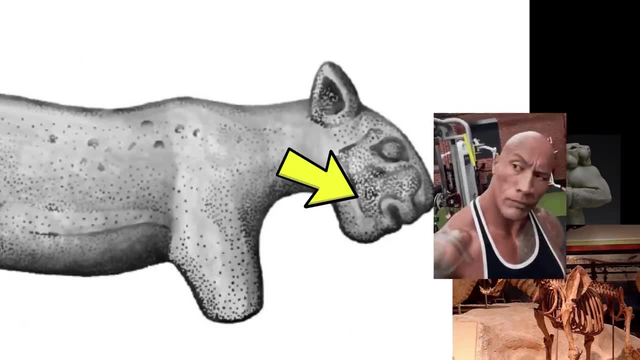 intriguing possibility, as it would be the only eyewitness depiction of such a creature while it still lived. If this is in fact the case, it raises another question: Why are there no sabre teeth? This oddity has spawned a theory that, contrary to most pop culture depictions, sabretooth 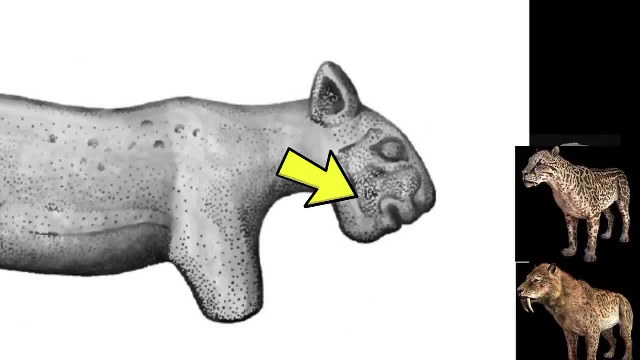 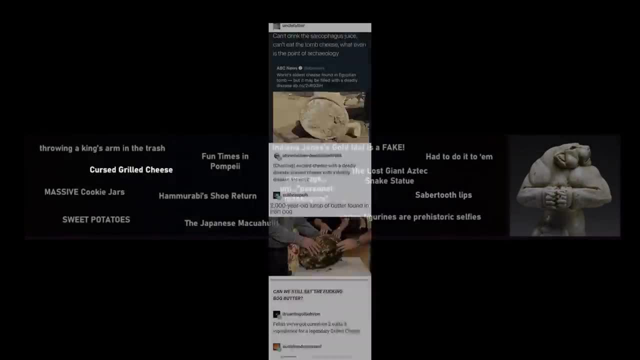 cats had fleshy lips that actually hid their long fangs in life, But this is a bit of an extrapolation based on pretty tenuous evidence. Cursed Grilled Cheese. This refers to a pretty funny Tumblr thread where users wanted to use the combined ingredients. 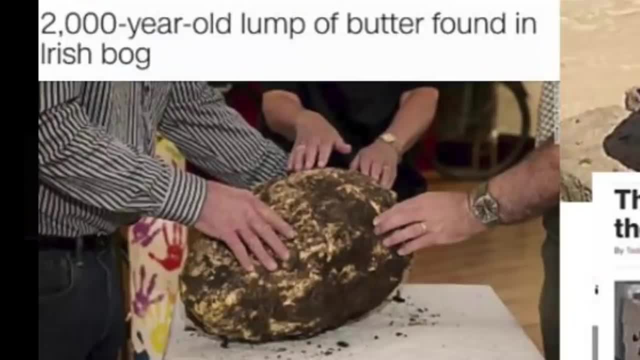 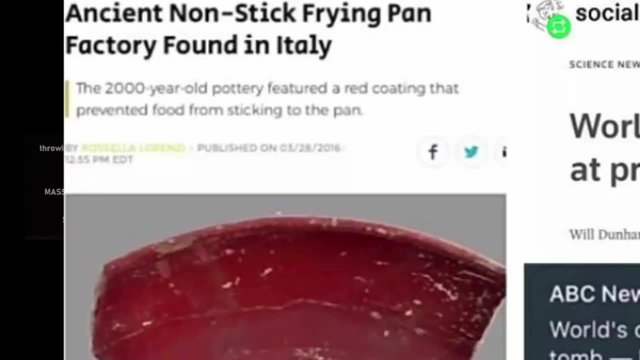 of the world's oldest cheese: a lump of 2,000 year old butter and pieces of 14,500 year old bread from Jordan on an ancient non-stick frying pan discovered in Italy To make the world's oldest grilled cheese. 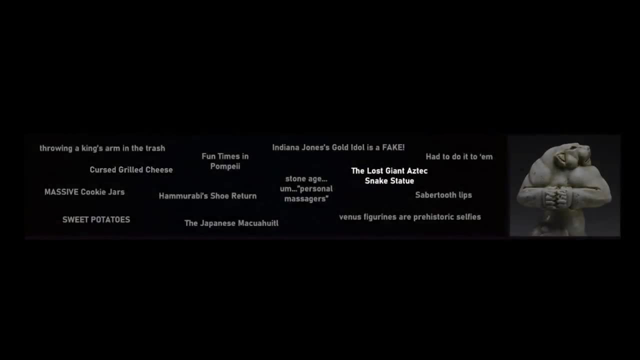 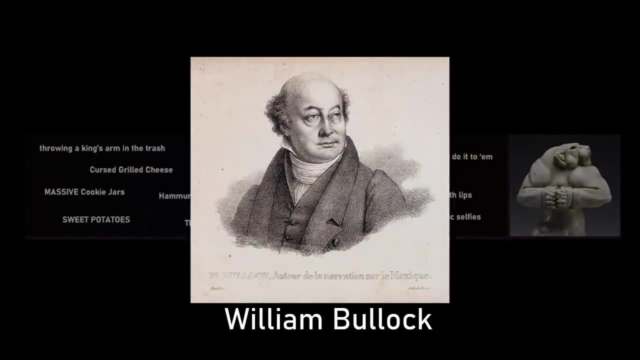 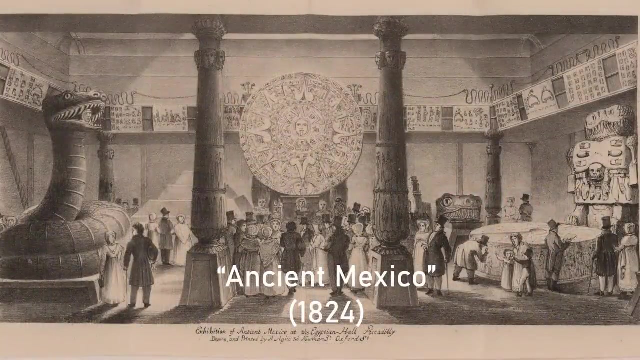 The Lost Giant Aztec Snake Statue. This refers to a very enigmatic and poorly understood artifact. In 1824, the English naturalist, William Bullock held a museum exhibition at the Egyptian Hall in London, England, titled Ancient Mexico. This exhibit primarily consisted of Aztec artifacts acquired by Bullock, such as authentic 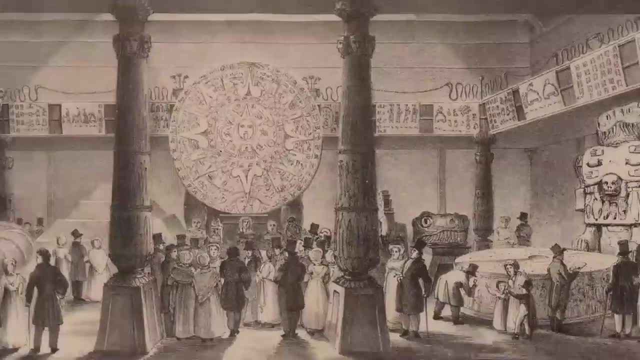 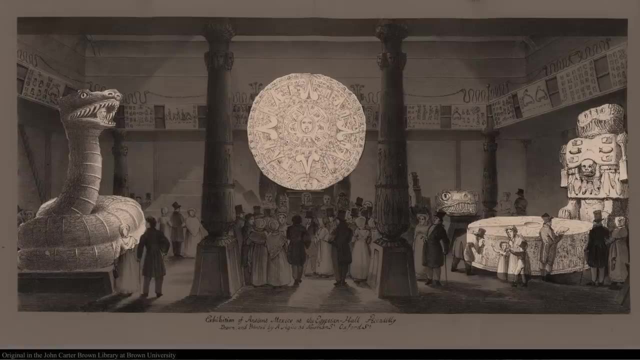 pottery and codices. However, In Mexico were several full-scale plaster casts of Aztec statues, These casts being based on the stone originals all the way back in Mexico. Two contemporary sketches exist of this exhibition and we can see that almost all the statues 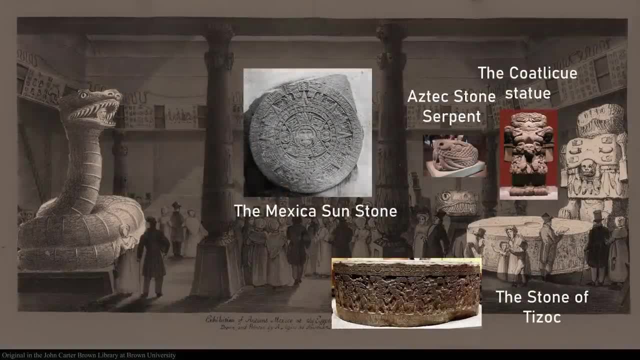 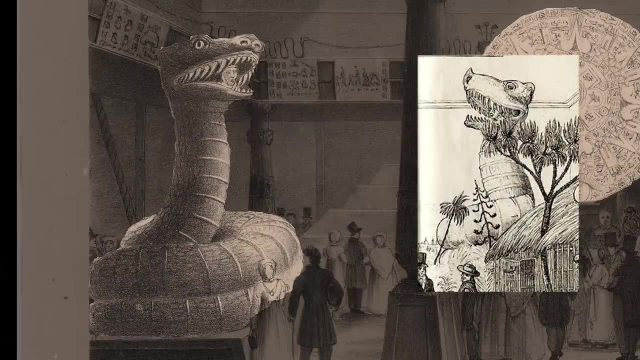 are known to us All, but one that is The most eye-catching of the plaster statues is this incredibly large and fearsome serpent with a man's head in its mouth. Suspiciously, there are no references to this giant Aztec snake statue. 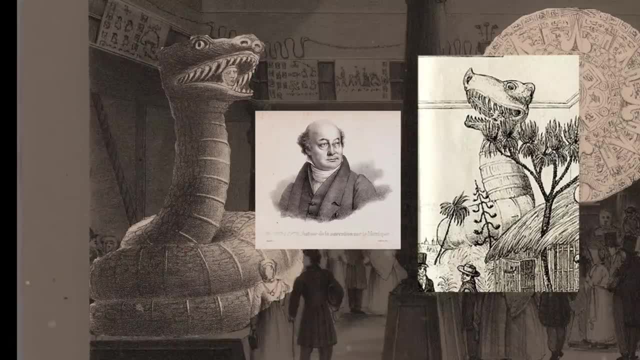 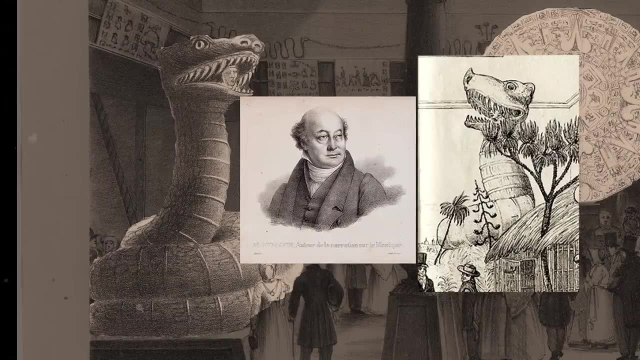 In fact, it is said to have been created by a man named William Bullock, and the original it was said to be based on has not been found. Some have said it could have been straight up fabricated or invented by Bullock, but this seems unlikely to me. 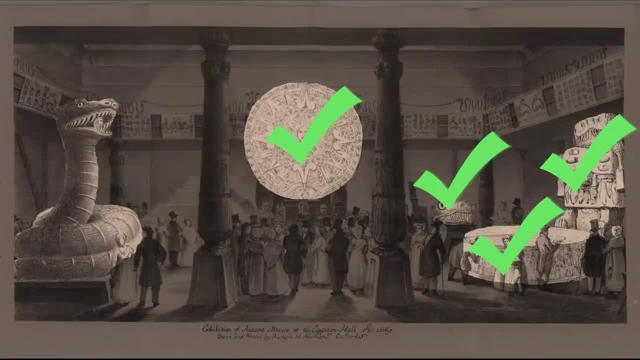 We know that pretty much everything else of the exhibit was based on real, authentic Aztec specimens, many of which we still have, All except this one. Even the plaster cast appears to have gone missing. as contemporary sources report, it was sold to a private collector after the exhibit ended. 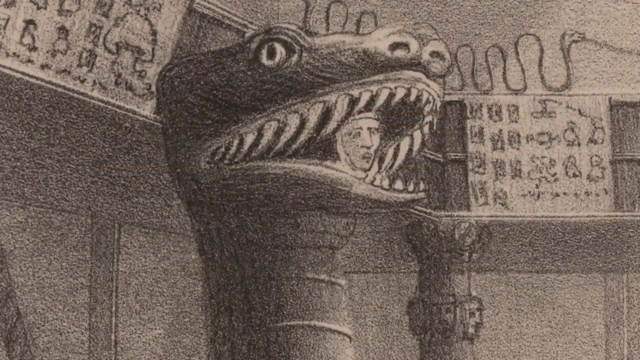 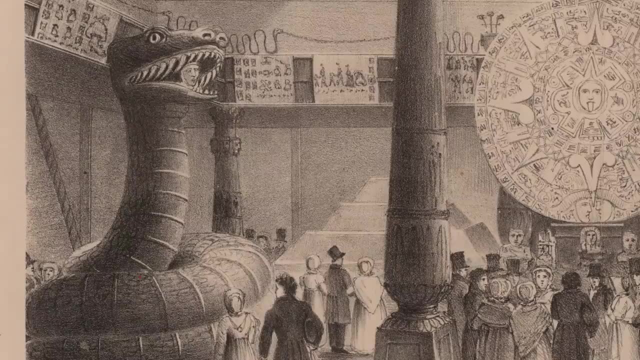 Never, Never, to be seen again. But like, how does something this big get lost or misplaced? It's all very weird and crazy that this huge, badass snake statue has straight up disappeared from history and no one knows any details about it or where it went. 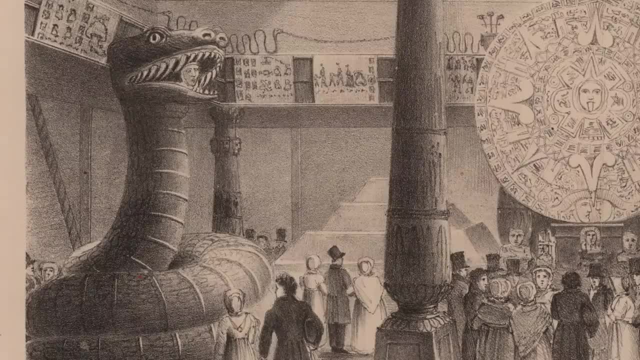 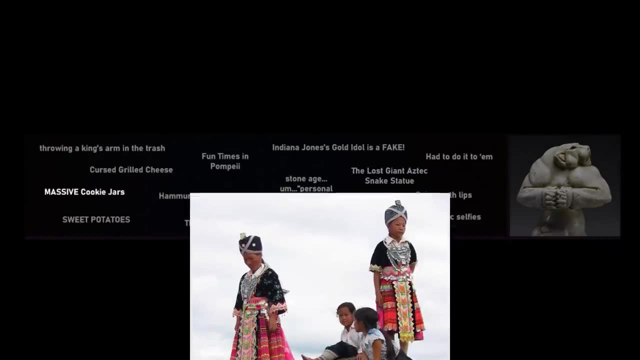 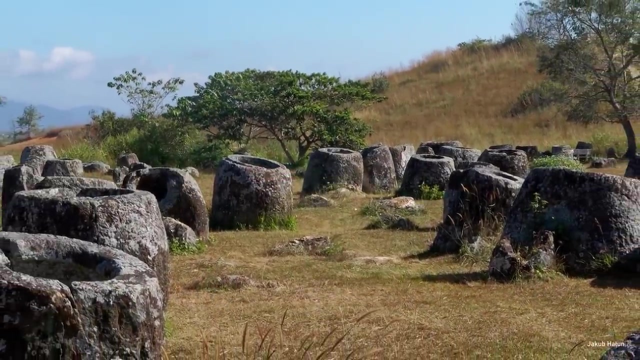 With hope. it's still collecting dust in the basement of some old English manor right now, just waiting to be uncovered- Massive Cookie Jars. This refers to the Plain of Jars in Laos, scattered across the valleys and footpaths. Some of the largest foothills of the Shangquan Plateau are thousands of stone jars, some 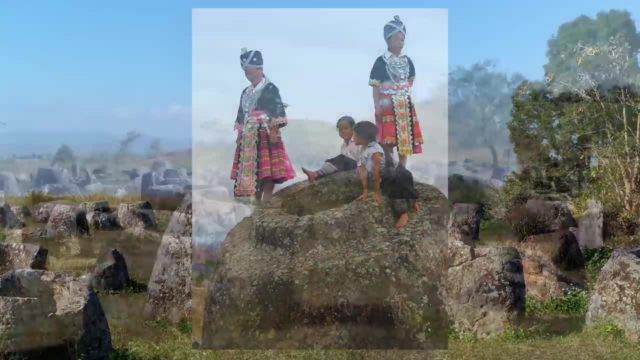 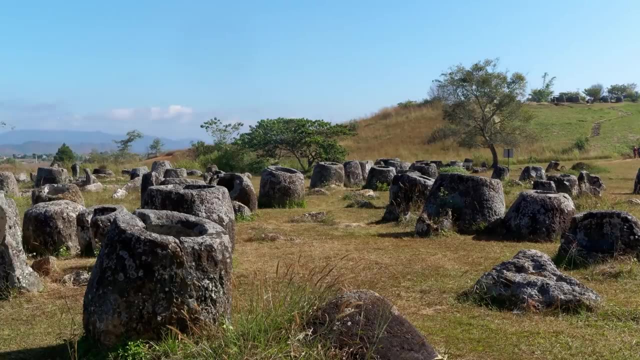 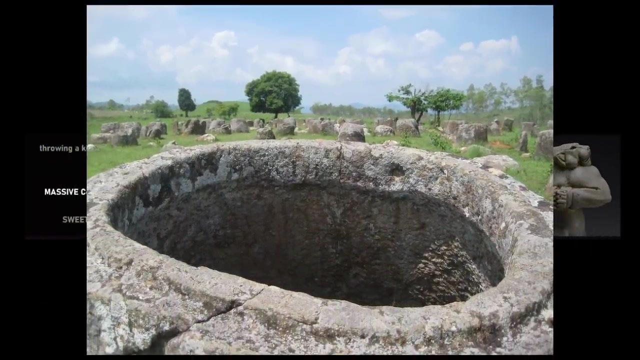 small and some truly gigantic. They were constructed by an unknown prehistoric culture between 1240 and 660 BC for an even more mysterious purpose. Some human skeletons were buried around the jars, while others have been found within them. A few show signs of cremation, so maybe the jars were prehistoric crematoriums. 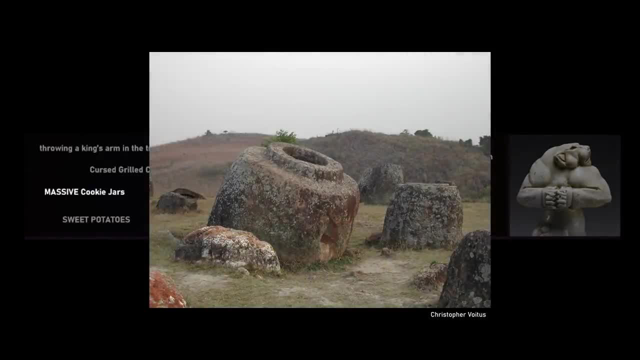 Most of the jars are unadorned, Lacking any inscriptions or pictures. All that is, save one which has a pictogram of a frog-like humanoid on it. The Plain of Jars are truly an archeological mystery. 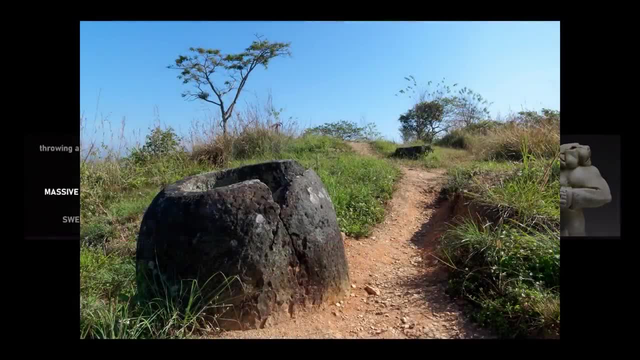 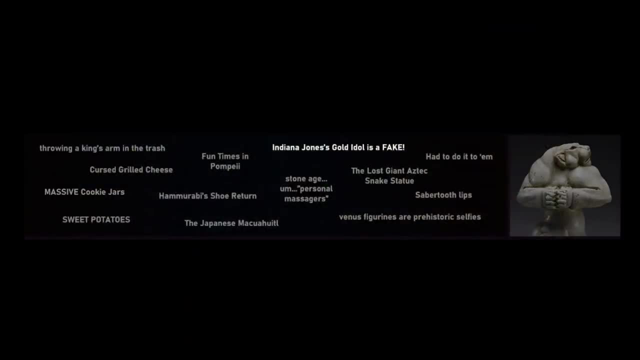 They obviously served a religious or spiritual function to a bygone people. but we can't really say much beyond that Indiana Jones' Gold Idol is Fake. In the first Indiana Jones film the fictional archeologist grabs a gold idol from an abandoned temple somewhere in South America. 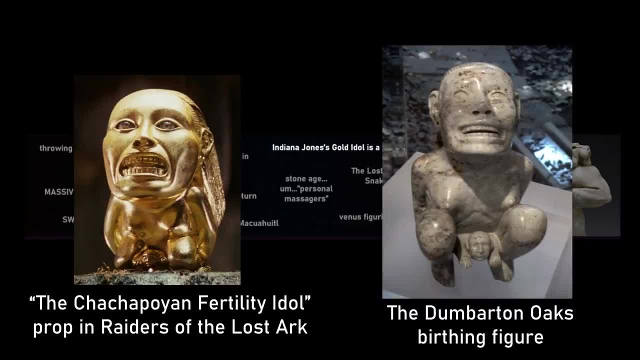 This prop is actually based on the real Dumbarton Oaks birthing figure. This figurine is said to be a piece of pottery, but it's not. It's just a piece of jewelry. It's a piece of jewelry. It's a piece of pre-contact art depicting an Aztec goddess giving birth. 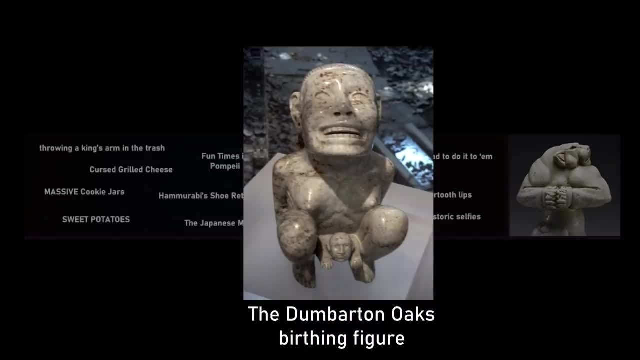 Now the Dumbarton Oaks figure has come under scrutiny and it very well might be a clever fake. The provenience or origins of the artifact cannot be confirmed because it first appears on the shelves of an antiquity store in Paris, France. 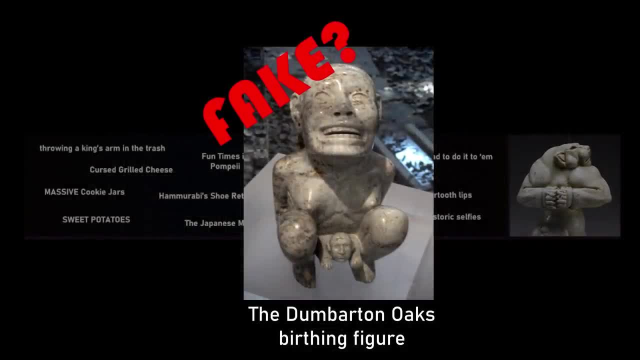 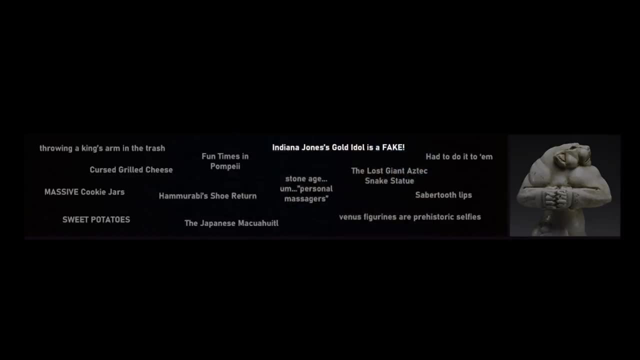 Additionally, recent microscopic analysis of the artifact have shown that the incisions and drill holes on it were probably made by modern tools, not ancient ones. This is an incredibly similar situation to the infamous Crystal. It's a very similar situation to the famous Crystal. 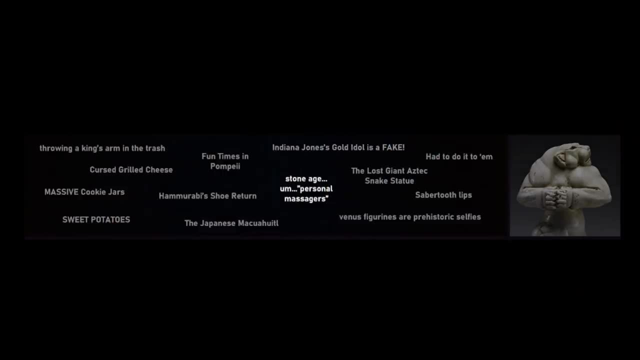 It's a very similar situation to the famous Crystal. It's a very similar situation to the famous Crystal. The reason behind it is that many of our ancestors were of the same origin, but they all had one and only one identity and they all were sent out to the world. 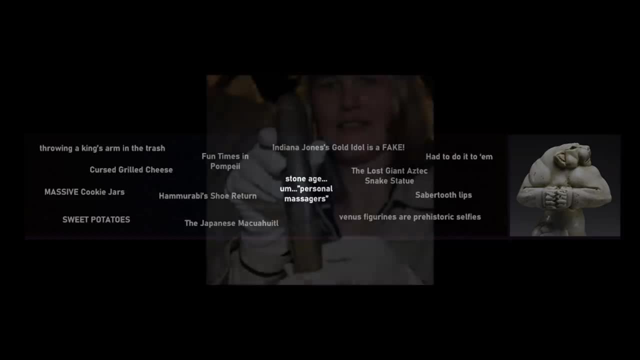 That's why we would use the word Crystal. Crystal Shades were discovered to be key to the Native American culture, as they were also known as the Black Dimensional skulls, which were, in fact, one of the most important archaeological artifacts. Stone Age personal massagers. 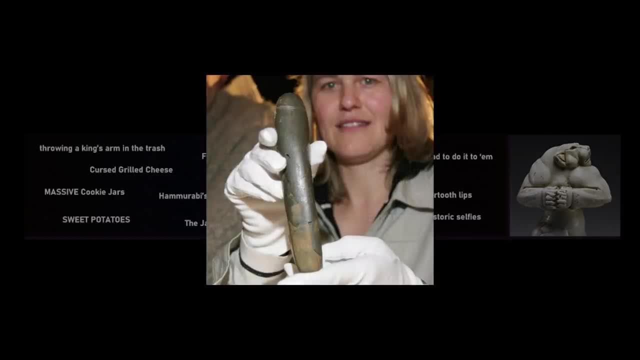 Stone Age personal massagers. There are several interestingly shaped stone artifacts found in prehistoric sites all over the world. Some were simply ceremonial or artistic in their purposes, while others are used for something else by our early ancestors. I'm glad she's wearing gloves. 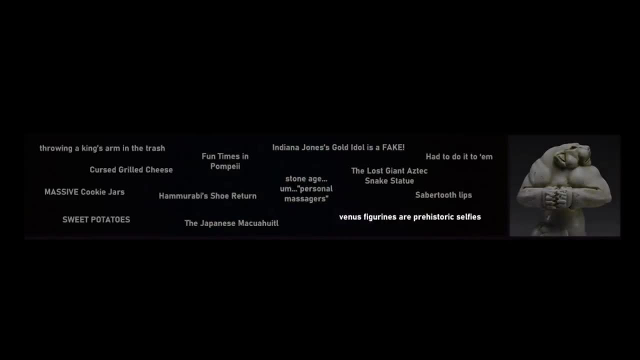 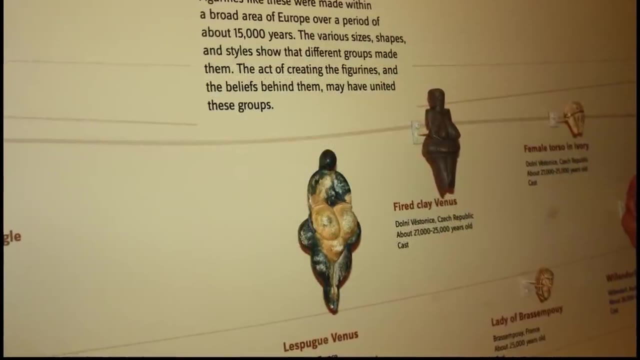 Venus Figurines are Prehistoric Selfies. This refers to a theory presented by anthropologists McCoyd and McDermott to explain the puzzling Venus figurines, a collection of Stone Age statuettes with large breasts and hips, and often lack heads or faces. 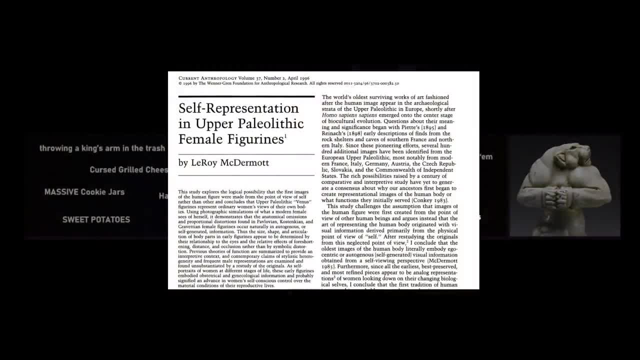 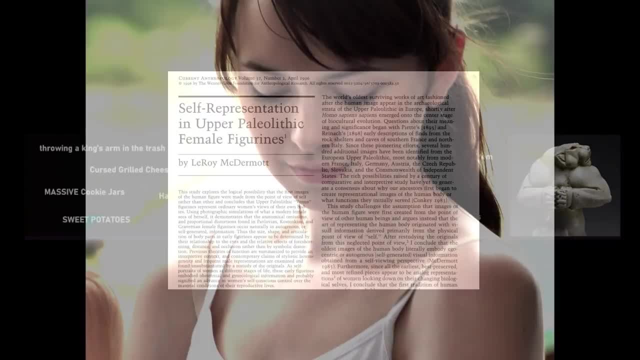 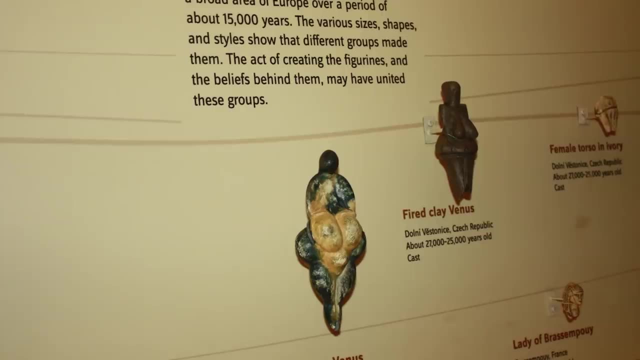 The scientists suggest that the Venuses look this way because they were made by prehistoric women looking down at their own bodies. According to them, without mirrors, early humans had to rely on their first-person perspective to describe themselves, and the reason why many of the figurines lack heads or faces is because the artists did not have mirrors to see their own faces. 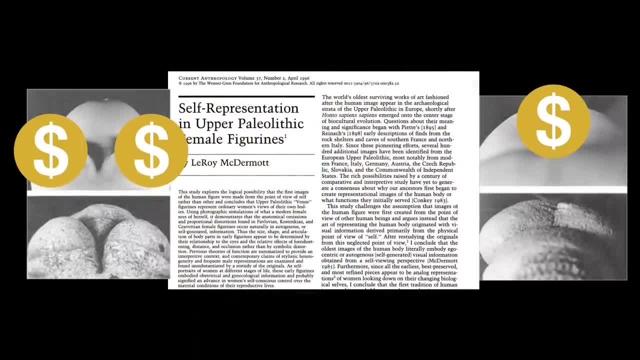 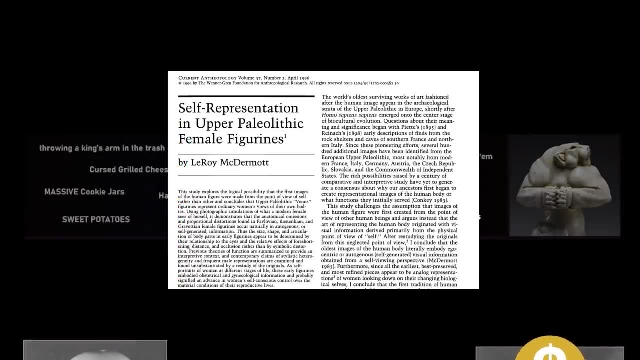 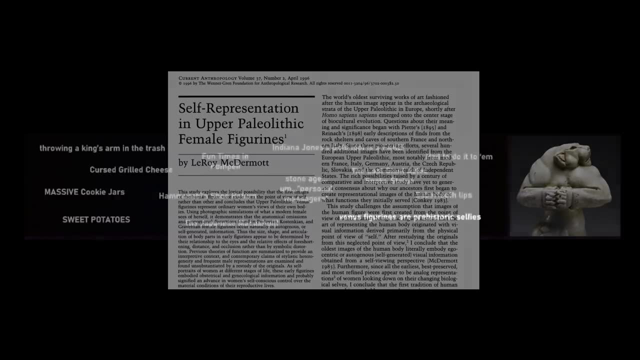 To top it off, McDermott's paper had these really great visual experiments that essentially consisted of pictures taken from a woman's first-person perspective looking down at her own nude body. Other anthropologists have criticized this interpretation because prehistoric humans would have obviously had access to streams and puddles which could have been used as mirrors. 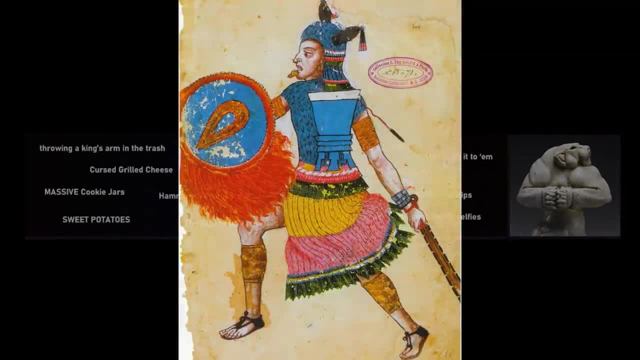 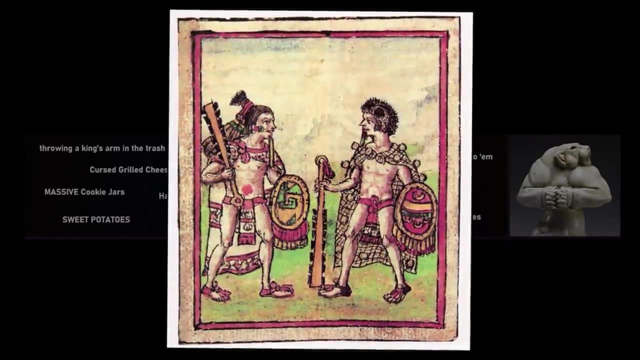 The Last Makiwattle. The Makiwattle was the first figure to have a face. The Makiwattle of Mesoamerica was one of the most badass weapons in history. It essentially consisted of a wooden club held in one hand with several obsidian blades as sharp as steel razors embedded in its sides. It was said to be so sharp that some Spanish conquistadors reported it could cut the head off a horse with one strike. although this might be a bit of an exaggeration, The Makiwattle was the choice weapon of countless Aztec, Mayan and Toltec elite warriors for centuries. 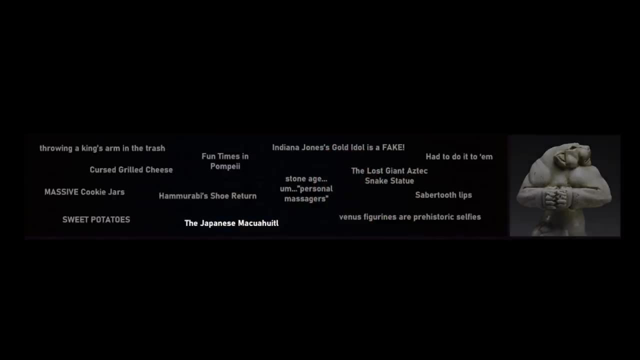 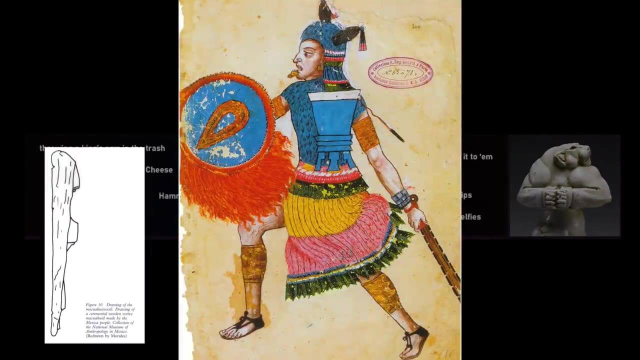 so it might be a little shocking to learn that up until the late 19th century there was not a single surviving Makiwattle dating to the pre-Columbian era. Oh, there were replicas made centuries after European contact, but no authentic specimens from before. 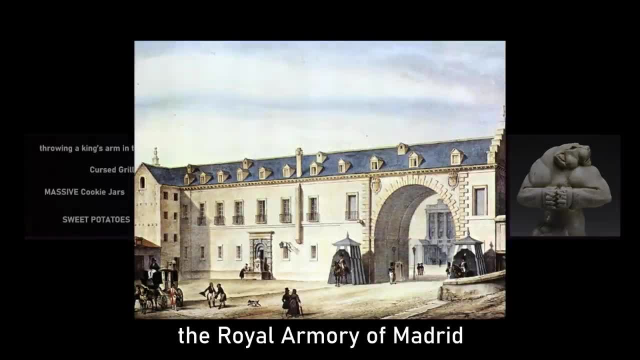 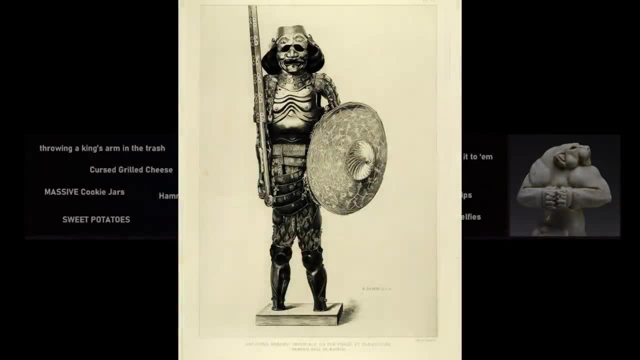 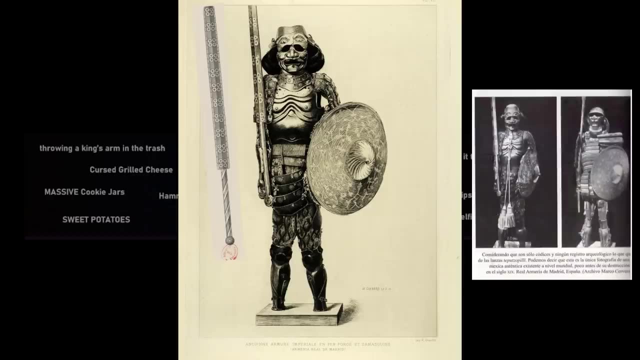 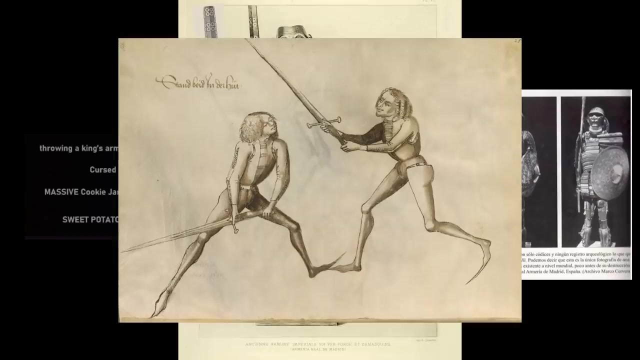 The Makiwattle in question appears in a catalog of the original Makiwattles. The Makiwattle in question appears in a catalog of the original Makiwattles. Some experts have suggested that this specimen represented a rare two-handed version of the Makiwattle. 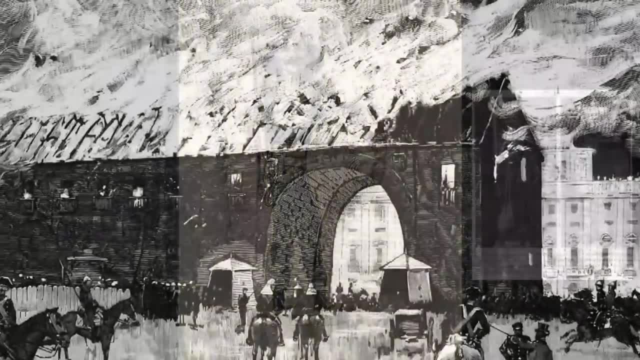 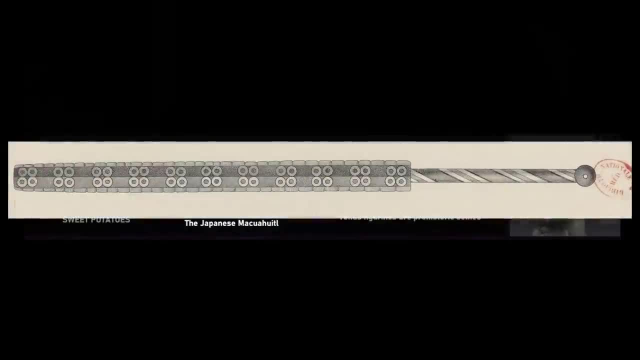 The from pocket znajduity of the animal started along the lateral edge of the armory in 1878, in 1884, meaning this elusive two-handed variant has been lost to time. Some have suggested that it might have served a purely ceremonial purpose, but with no artifact.